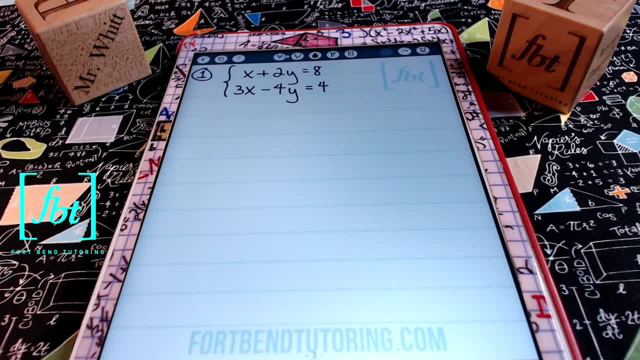 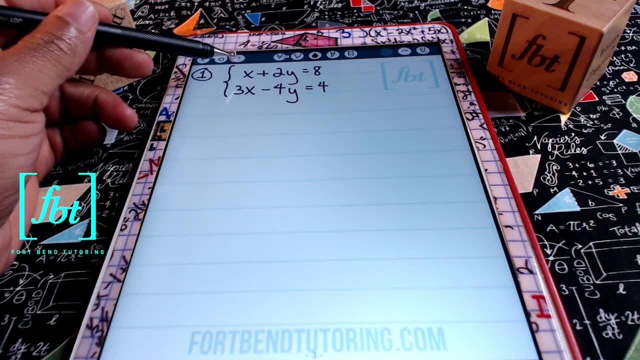 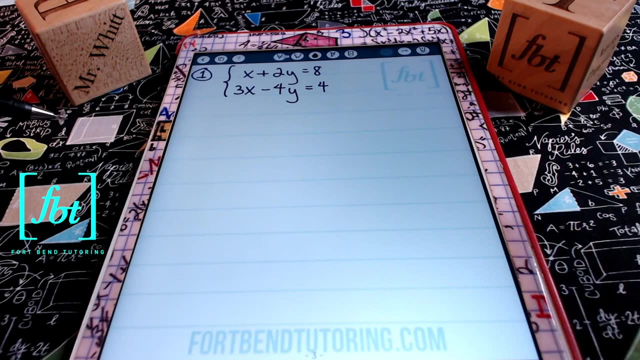 let's go ahead and look at problem number one, where we're given a system of linear equations. We have two variables with two equations. I have the first equation here, which is X plus two: Y equals eight. I have the second equation, which is three X minus four, Y equals to four. And what is? 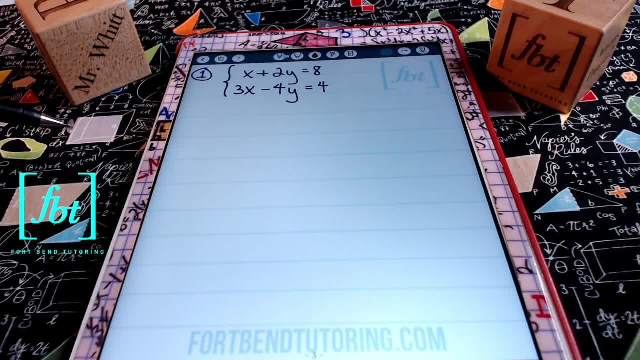 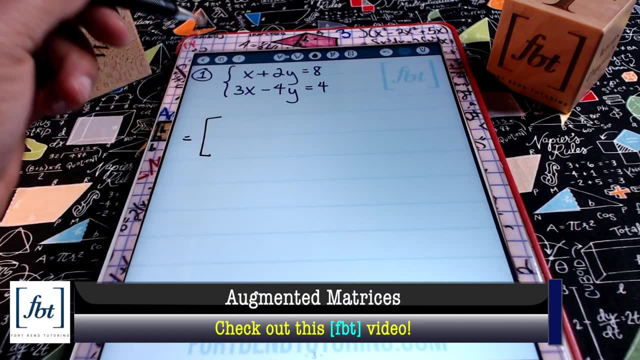 the first step. guys, That's right. We want to write our system in an augmented matrix and it's going to be just like this. Let's go ahead and take a look at it. We'll be needing the coefficients from both equations. I'll start out with one coming from that one X. I'll need a two from the two Y. 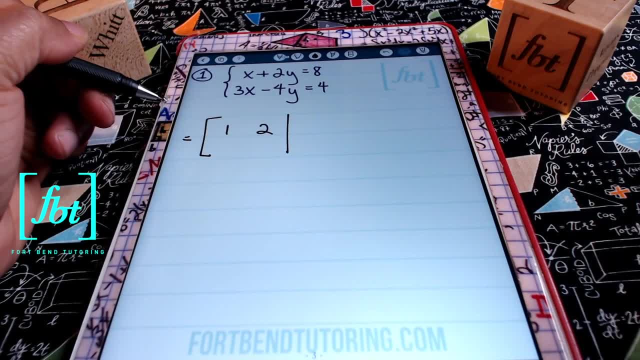 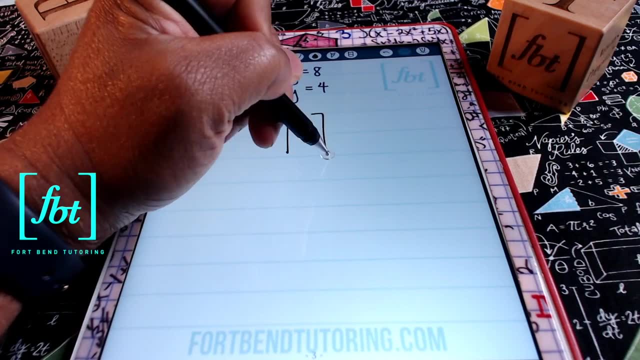 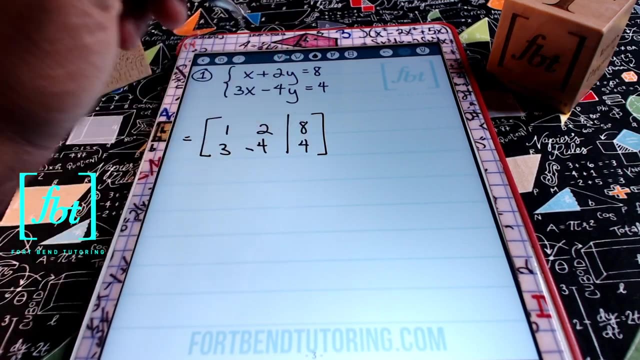 And then I'm going to have here that solid line separating the left side of the equations from the right side of the equation, And then I'll bring down that eight And I'll also have the second row which has coefficients three negative four, And then we have that set equal to four, And 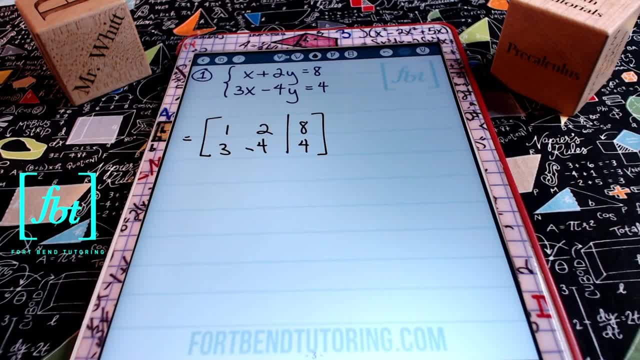 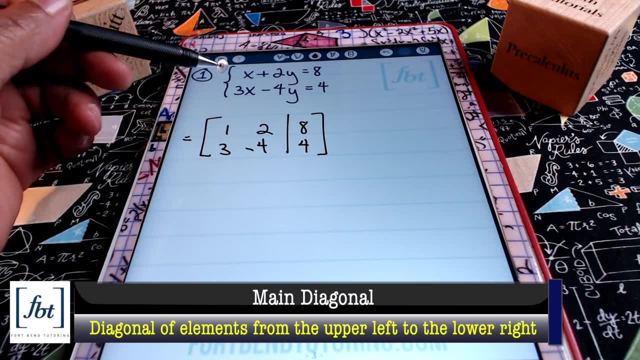 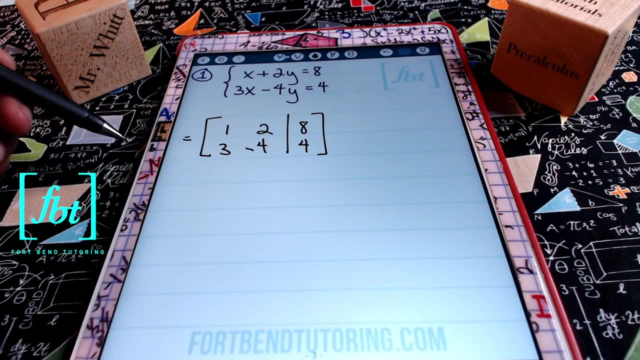 that augmented matrix guys. here we want to rewrite the augmented matrix and row echelon form. So our goal here is to make sure that we have ones down this main diagonal here. That diagonal comes from the upper left down to the lower right, with zeros underneath or above, for that matter. the main. 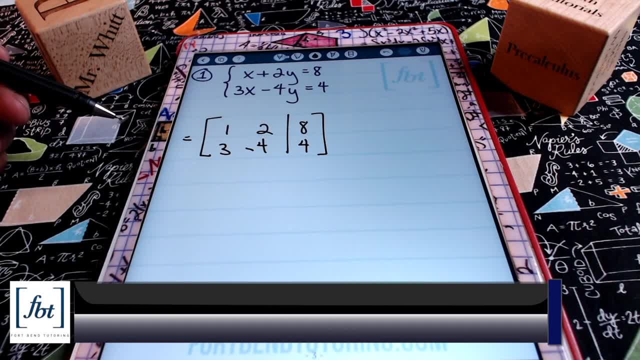 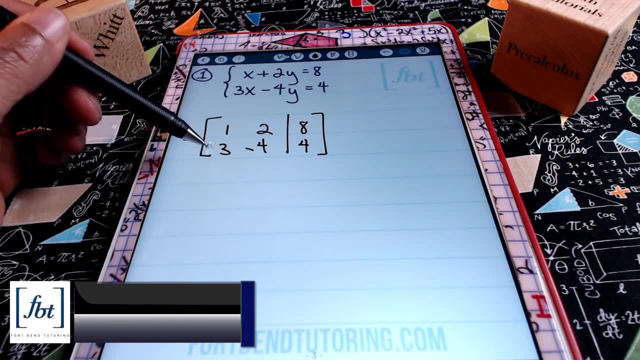 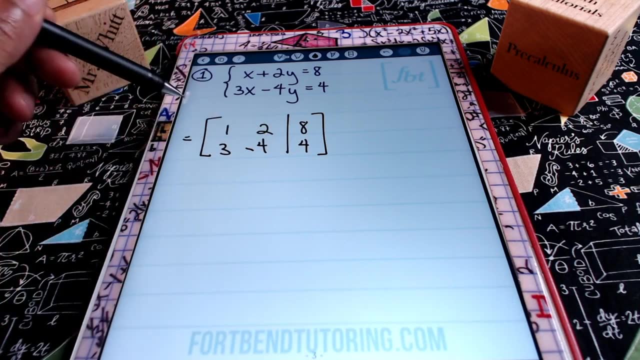 diagonal. Okay, So we want a triangular form. That's right, And the triangular form simply means that along this main diagonal here, that there's going to be zeros found above it or beneath it. In the examples that you'll see, you'll see that they'll have zeros beneath the main diagonal here. 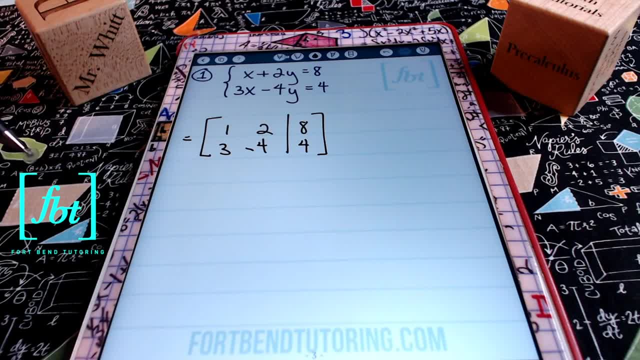 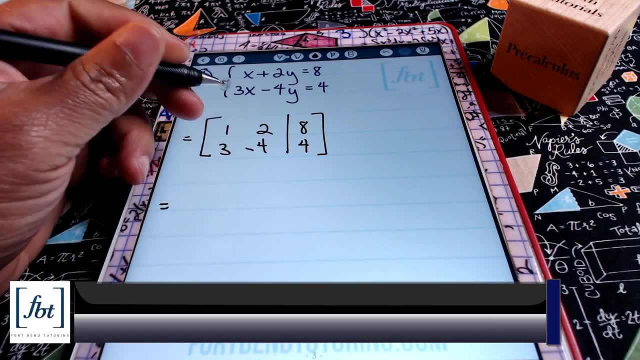 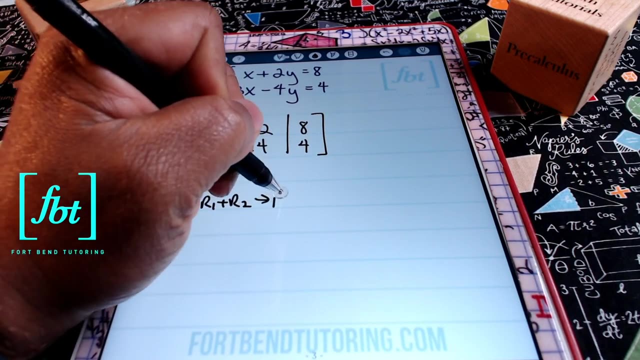 That is your goal here for getting your matrix simplified in row echelon form. So in order to get a zero here where the three is, I'm going to show that my row operation is going to be to multiply negative three times row one. add that to row two and then put the result in row two. 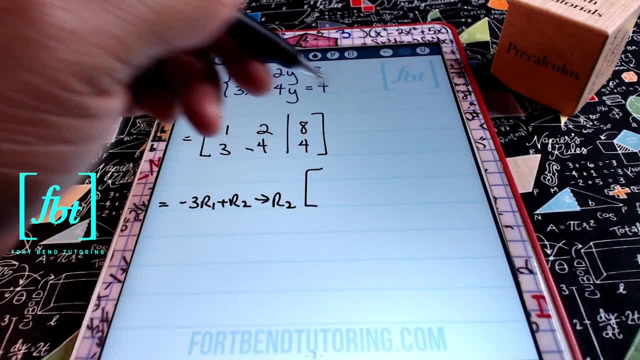 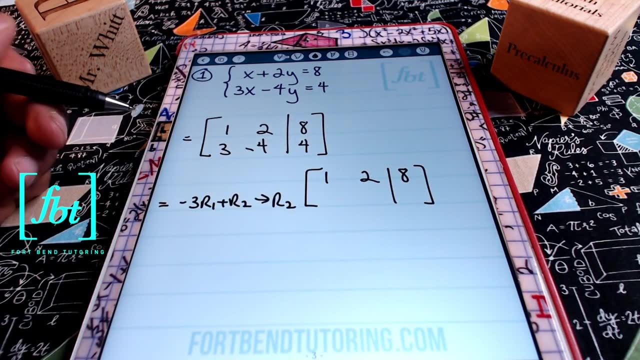 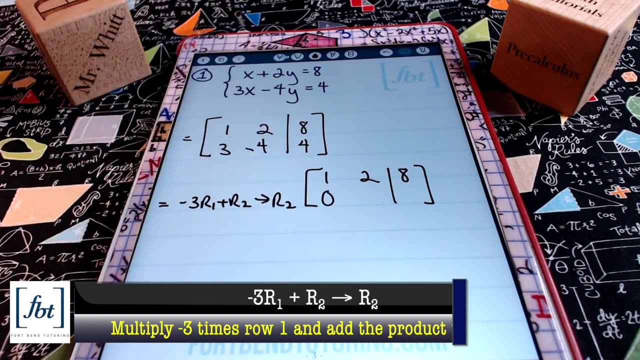 That means that the first row will remain the same. I'll have a one, a two, then an eight in that first row, Whereas in the second row, after multiplying one times negative three, you'll get negative three. Negative three plus three gives me zero for that first element. 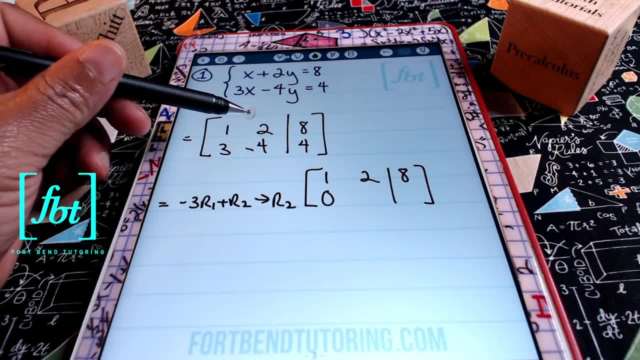 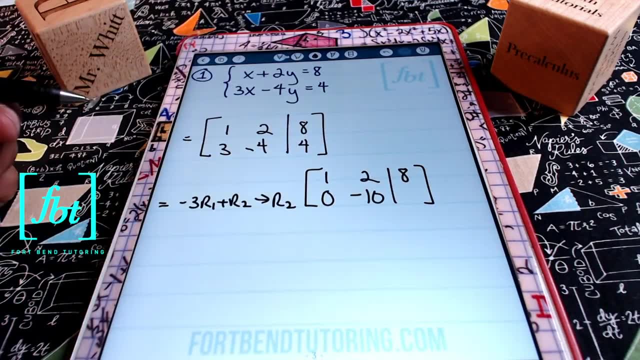 in the second row. Then I'll be multiplying two times negative three to give me negative six, And then negative six plus negative four gives me negative 10.. All right, And that becomes the second element in the second row. From here we'll go ahead and multiply negative. 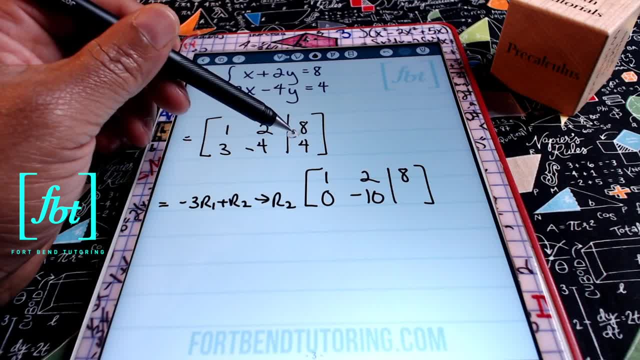 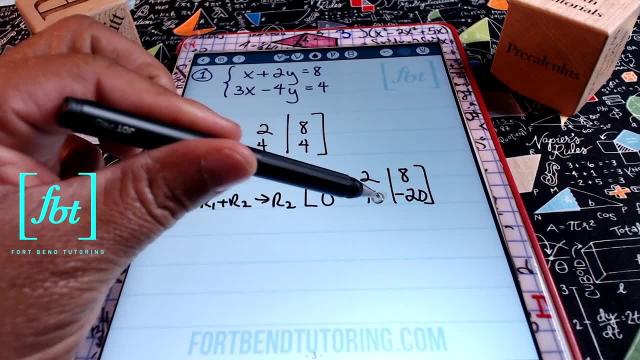 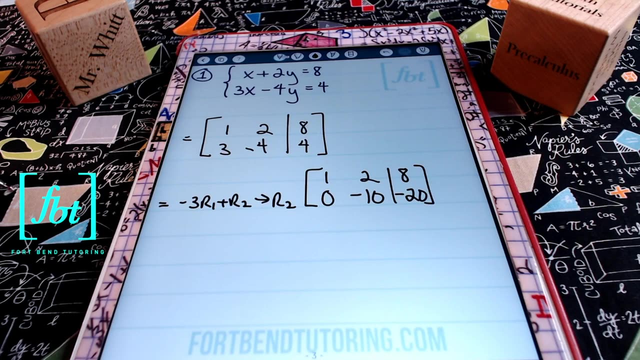 three times eight to get negative 24.. Then, adding negative 24 plus four gives you negative 20.. All right, So remember our main diagonal. this diagonal that contains the one and the negative 10 is where we want every element to be a one, to get it in row echelon form. Currently, what? 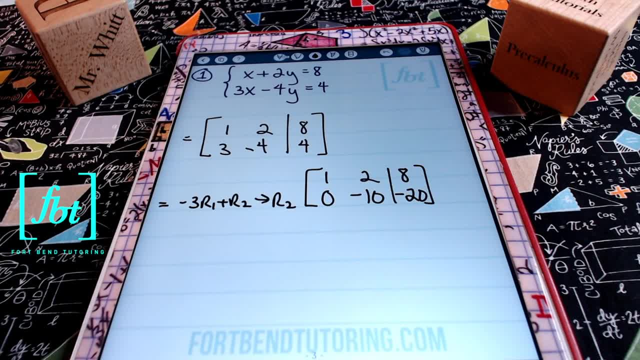 you're looking at is triangular form and technically you could stop right here and rewrite your system using the information that you have here and go ahead and solve your equation. However, to put it in row echelon form, you'll want that second element in the second column, this negative 10 here you'll want it to be. 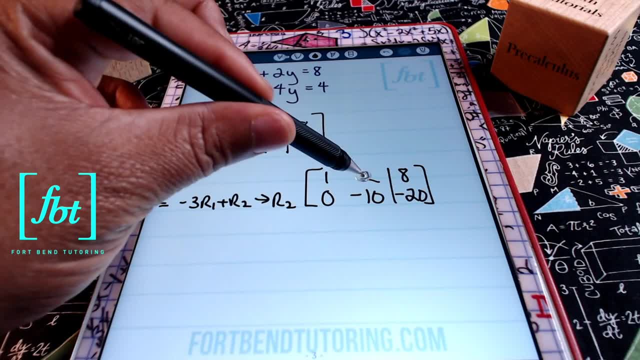 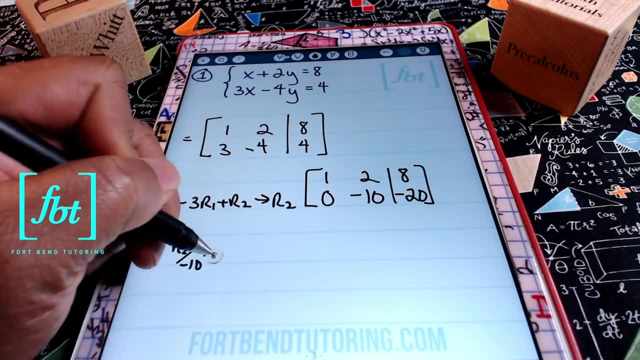 a 1.. So let's do just that. In order to make this negative 10 a 1, my next row operation is to have row 2 divided by negative 10 and then put that result in row 2.. So this is what we'll be doing. 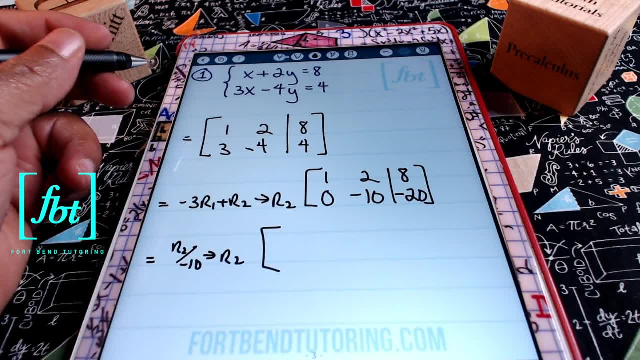 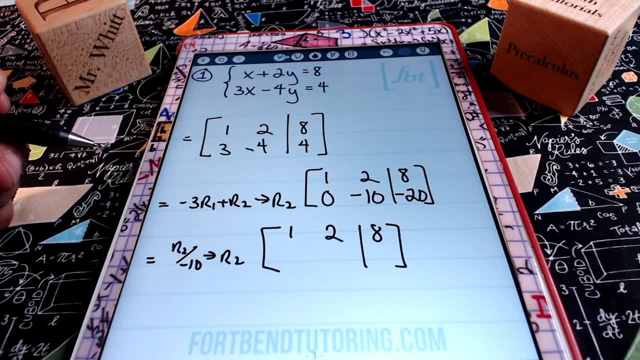 here for our last step. to get it in row echelon form, Go ahead and bring down that first row as 1,, 2, and 8, and then for the second row, remember we're dividing everything by negative 10.. So 0. 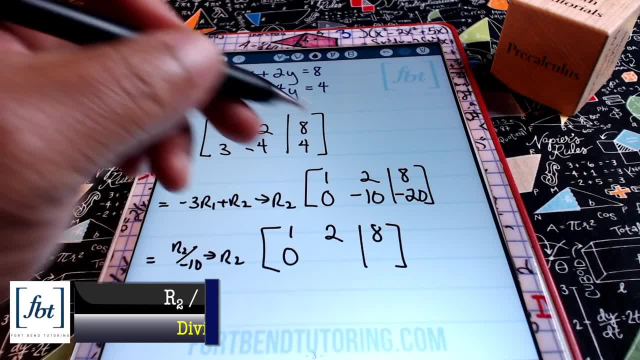 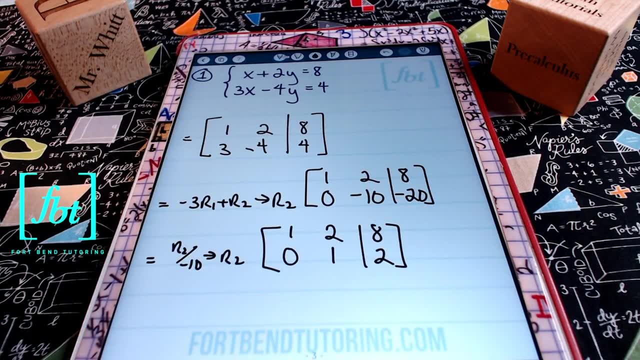 divided by negative 10 is 0 and negative 10. divided by negative 10 is 1 and negative 20 divided by negative 10 is positive 2.. You now have the problem in row echelon form, guys. So this is what we're. 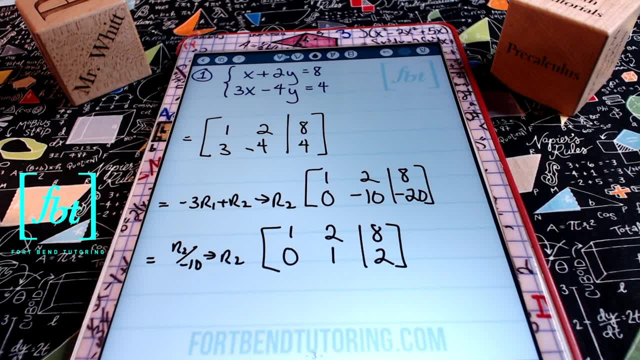 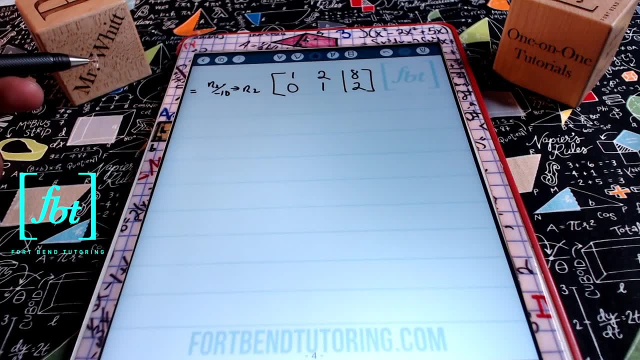 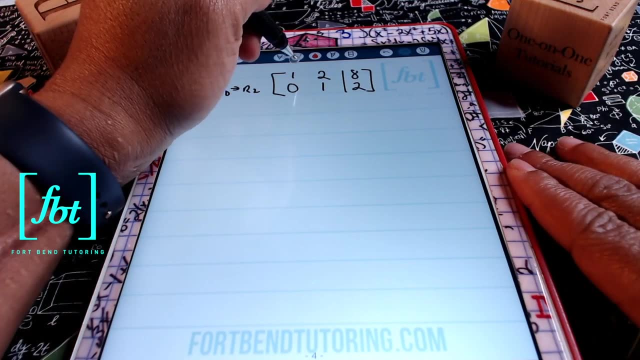 looking for when doing your row echelon form using the Gaussian elimination method. Let's move on to the next page. So remember it's once you have it in row echelon form that we'll go ahead and back, substitute and rewrite our system of equations using the information here. So back, substitute and recall that our first column is for: 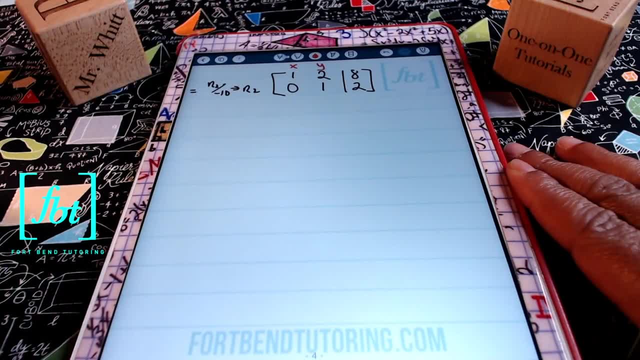 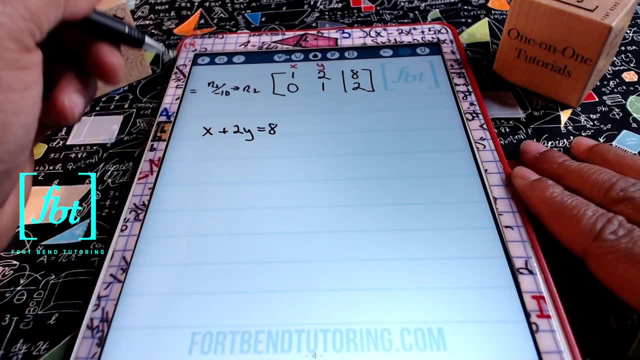 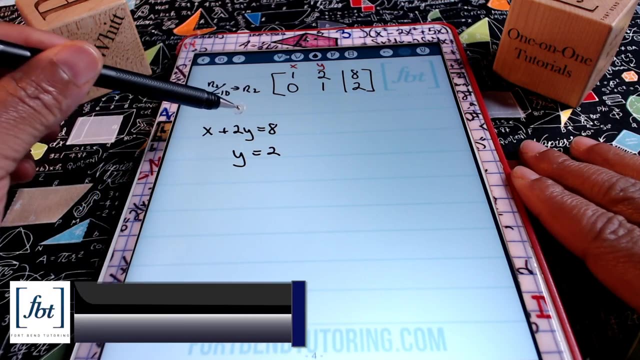 the x variable where the second column is for the y variable. Knowing that, I can rewrite our equations as: x plus 2y equals 8, and the second equation will be y equals 2.. Since we know that the variable y equals a 2, we can use substitution in the first equation to 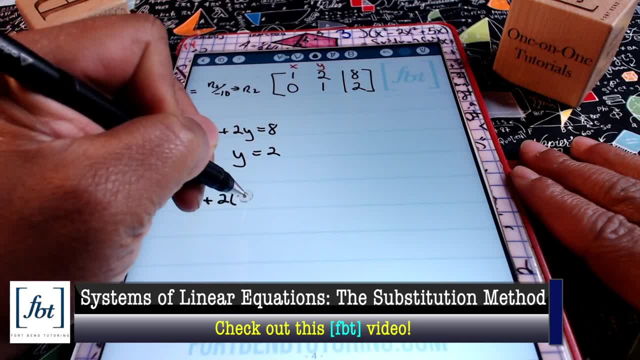 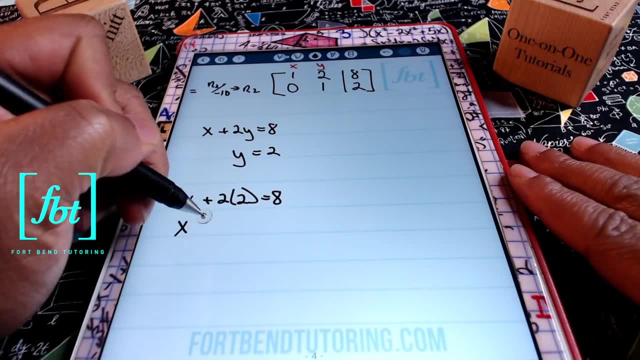 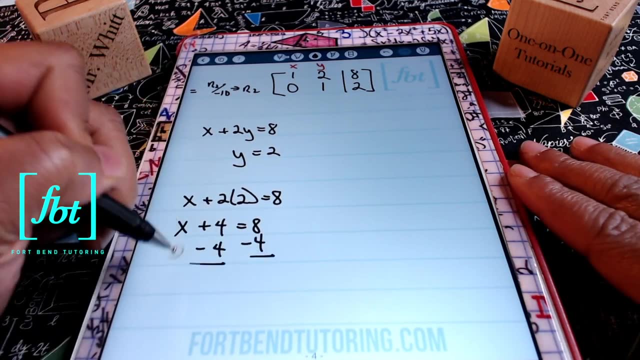 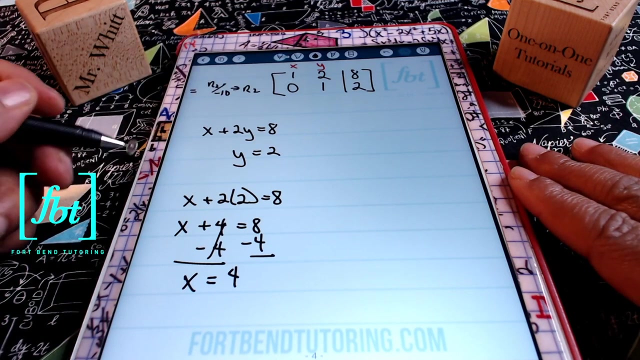 rewrite our system of equations using the information here. So back, substitute and recall that our first column is for the x variable where the second column is for the y variable, Knowing that I can rewrite our equation as: x plus 2 times 2 equals to 8, and from here we'll go ahead and simplify and solve for x. So this gives us x plus 4 equals 8, and then, solving for x, you'll be subtracting 4 to both sides and you'll end up with x being equal to positive 4.. Now that we have our answer for both x and y, your solution set will be 4 and 2.. Red boxes: 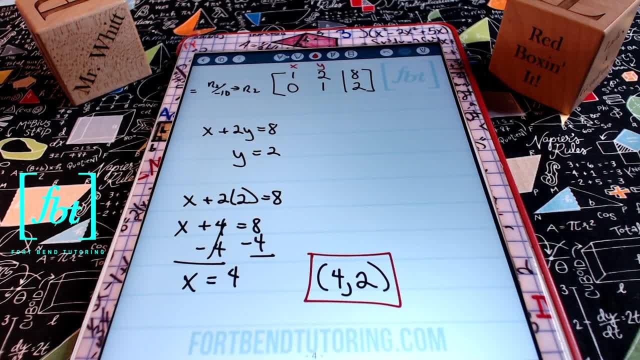 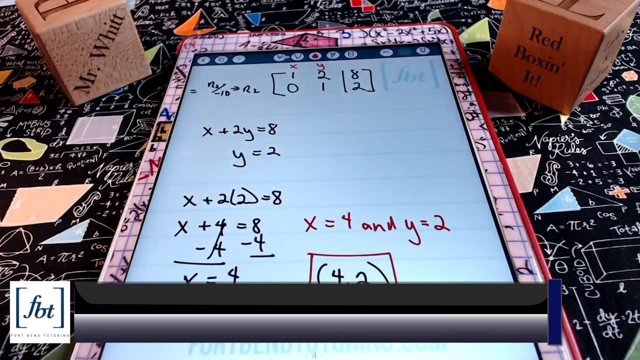 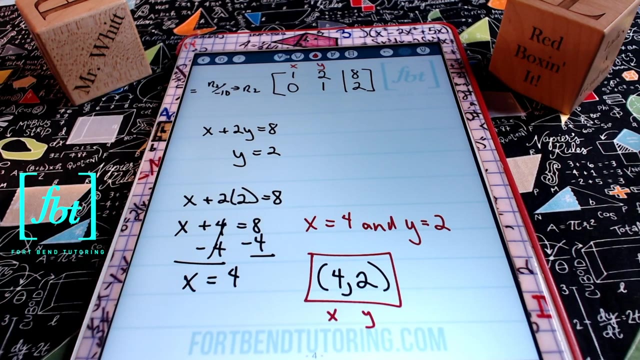 That's right people. So you can write your answer as an ordered pair, or you can expand this, knowing that the first value in the ordered pair is x, knowing that the second value in the ordered pair is y, and simply have x equals to 4 and y equals to 2.. Done and done people, Just like that. Alright, so most of your instructors will want the answer to be as an ordered pair in this case. If you have more than two variables- let's say you have three variables involved in your system- You can write your answer as an ordered pair, or you can expand this, knowing that the first value in the ordered pair is x, knowing that the second value in the ordered pair is y, and simply have x equals to 4 and y equals to 2.. Done and done people, Just like that. Alright, so most of your instructors will want the answer to be as an ordered pair in this case. If you have more than two variables- let's say you have three variables involved in your system- You can write your answer as an ordered pair, or you can expand this, knowing that the first value in the 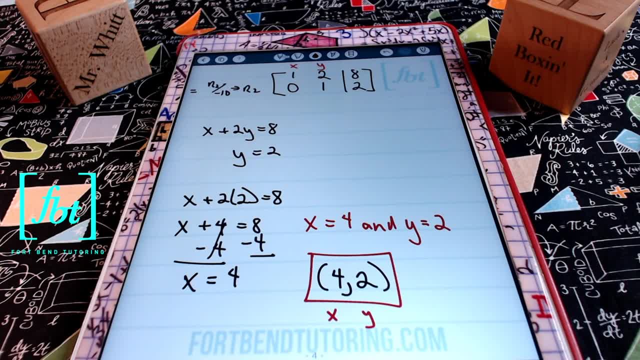 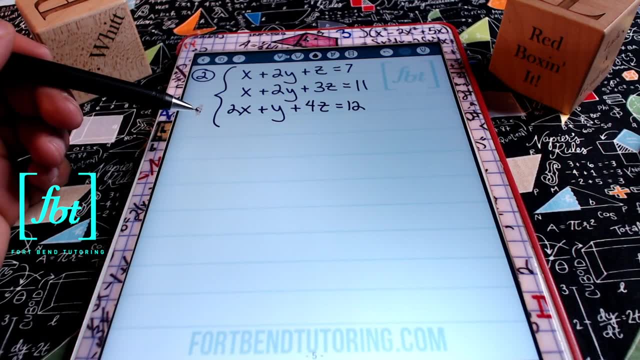 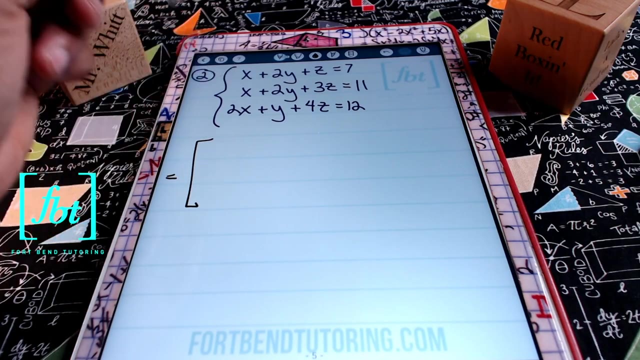 system of equations, you'll write your answer as an ordered triple. So that concludes problem number one. Let's check out problem number two. And in problem number two, notice that we have three equations with three variables. So in this case we'll end up with an additional row and column when we're setting up our augmented matrix. Alright, so let's see what that looks like. We're going to set up our augmented matrix using the coefficients, once again from the system of equations. You'll have one, two. 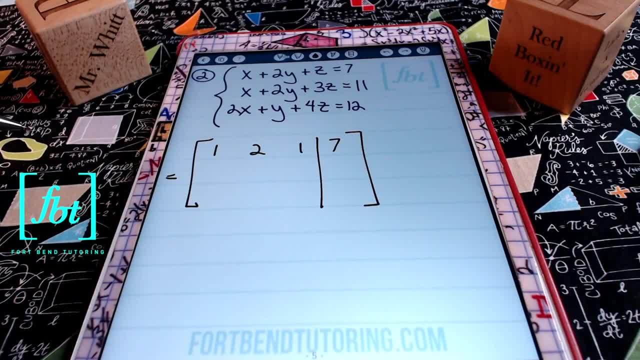 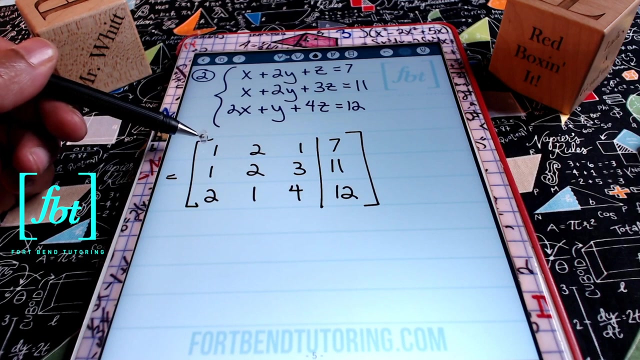 three and then eleven. In the third row you'll have two, one, four and twelve. So recall that our goal is to put this in row echelon form. We want the main diagonal right here that currently has one, two and four. We want those values in that main diagonal to be. 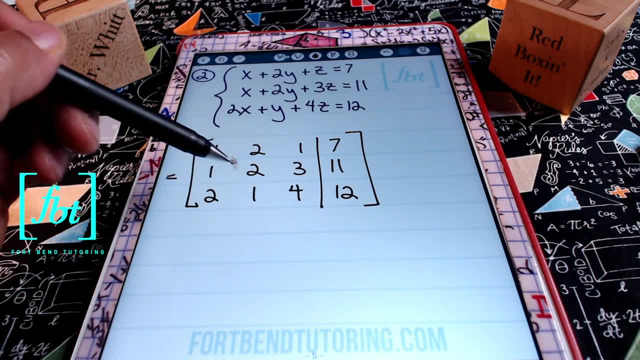 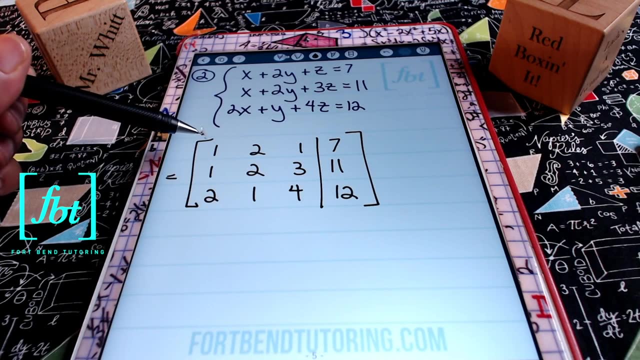 ones. We want the values underneath the main diagonal to be zeros in order to put it in row echelon form. So what I prefer to do, guys, is focus on one column at a time. So I'll be focusing on this first column, making sure that that first element in the first row is one and it is, and then making zeros underneath that one. So that means that this second row's first element of one here has got to go. I need it to be a zero. 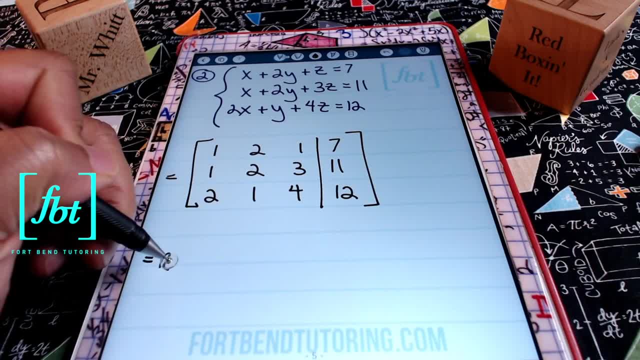 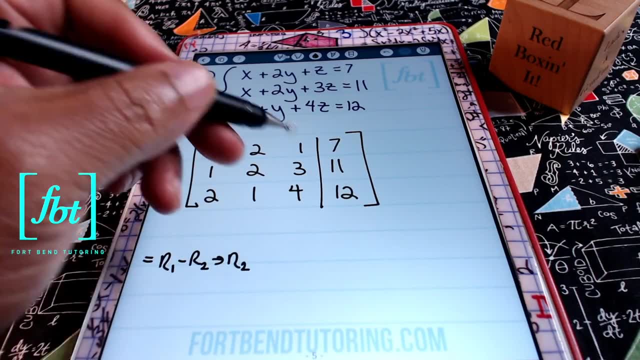 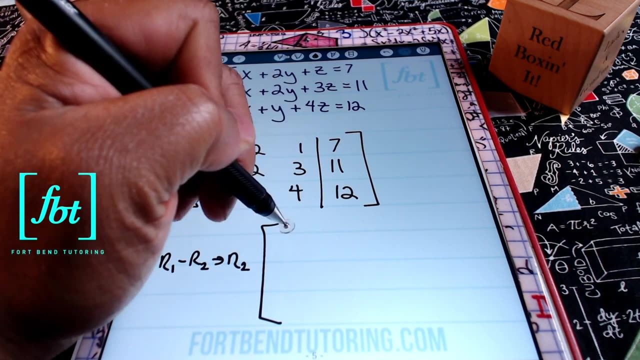 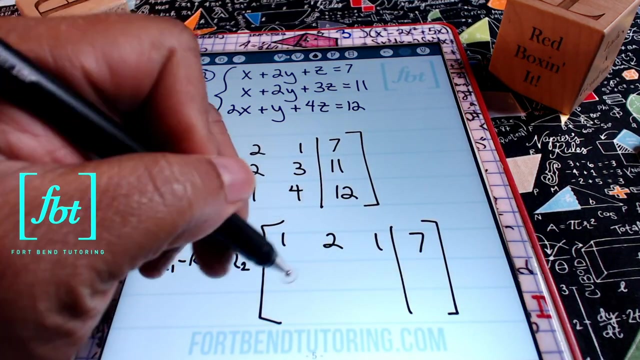 So I'm going to have as my row operation row one minus row two and putting the result in row two. Okay, just like this. So, that being the case, I know that the first row and the third row are going to be unchanged. So I'll be bringing down this one, two, one and seven in the first row And in the third row, I'll be bringing down the two, one, four and twelve in the third row. 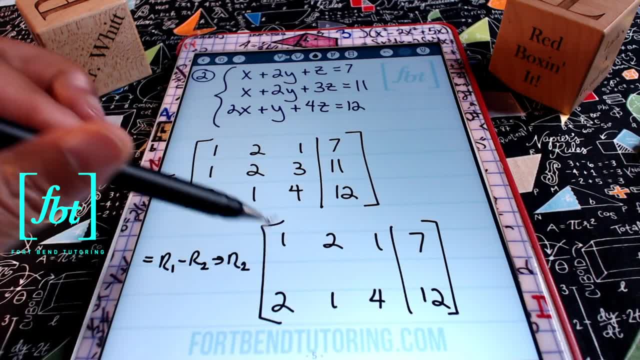 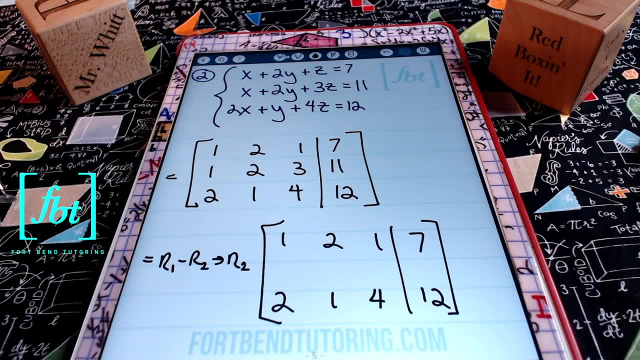 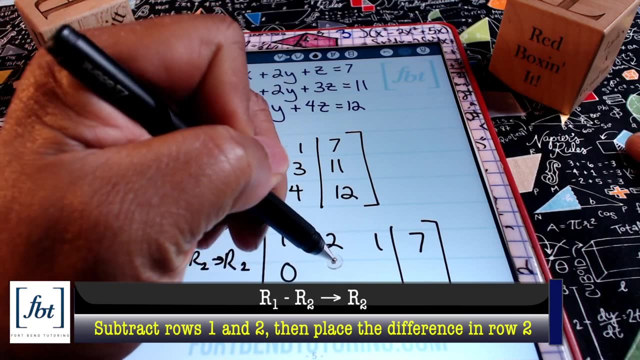 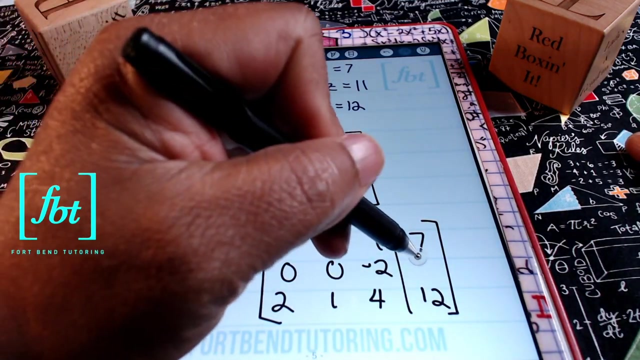 What I will be changing is the second row, knowing that I'll be subtracting these two rows here. or you can say that I'll be adding the opposite of row two to row one, So carrying this operation out, I'll have one minus one is zero, I'll have two minus two is zero, I'll have one minus three is negative two, and I'll have seven minus eleven is negative four. All right, So this is what we have so far In our next step. 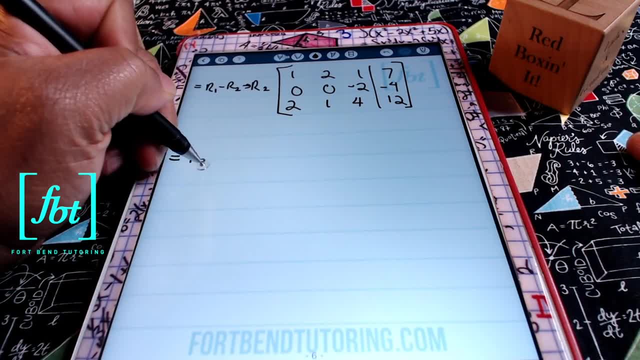 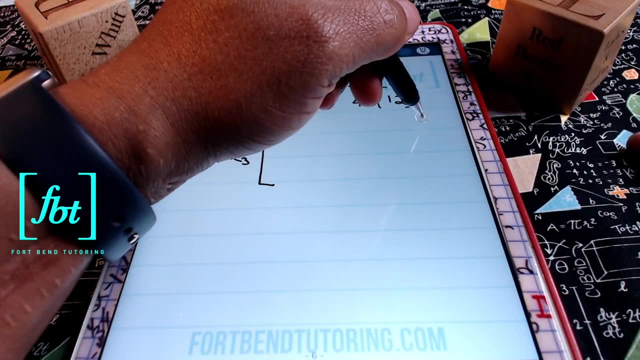 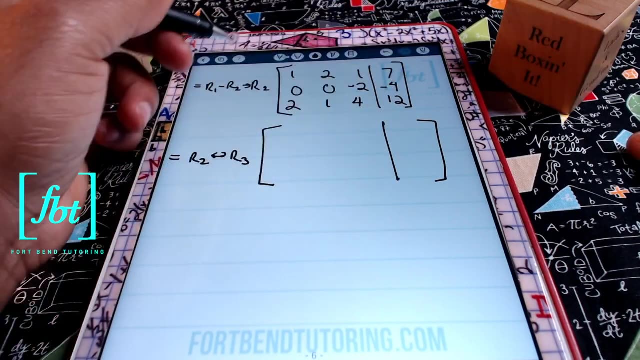 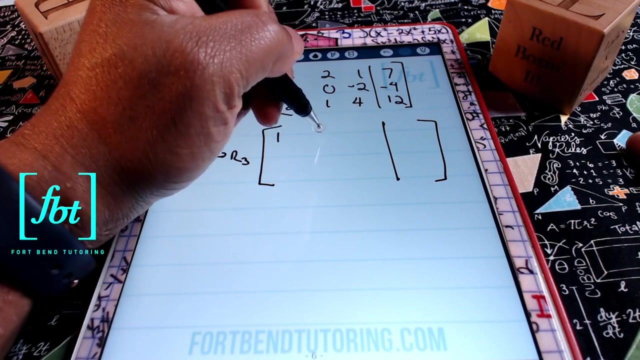 I'm going to show that I'll be swapping out row two with row three. The reason why I want to do this, guys, is because I want to keep in mind that I want this main diagonal here to have coefficients of one down the main diagonal, And it's going to be a lot easier for me to make that happen if I swap out the second and third row. So we're going to be bringing down the first row as it is, this one, two, one and seven- And then by swapping out the 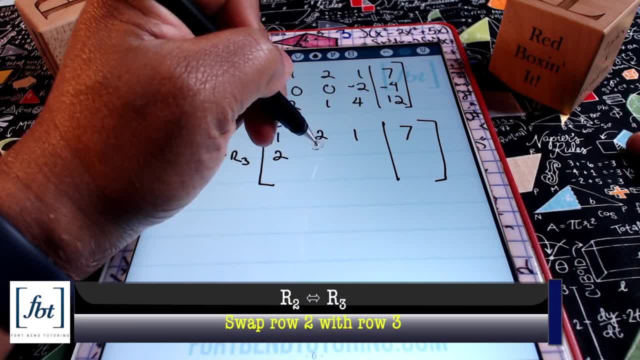 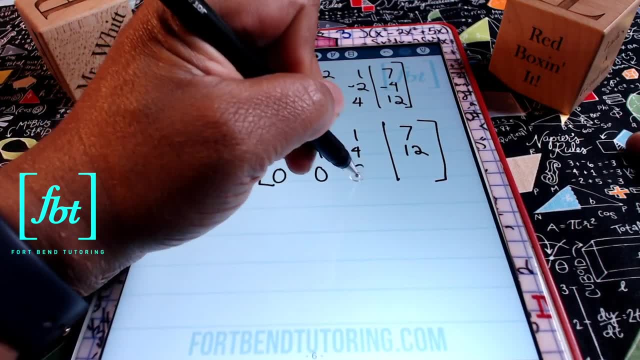 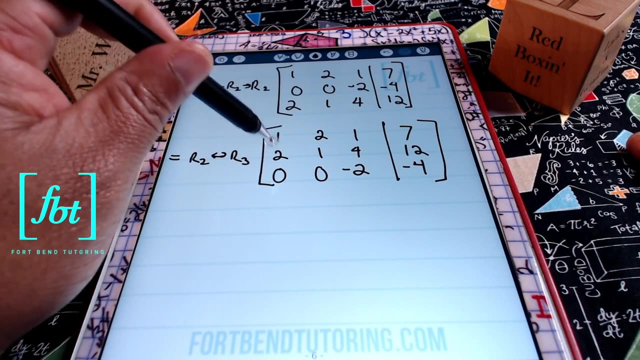 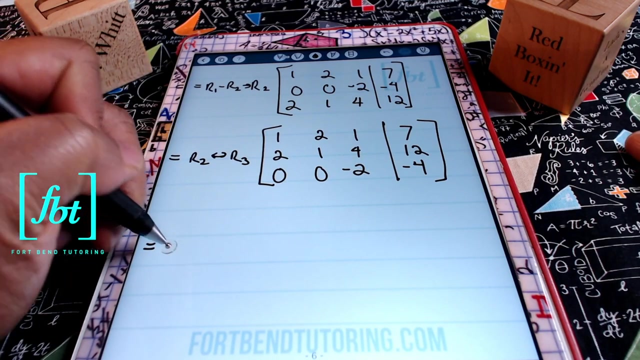 second and the third rows, I'm going to end up with two, one, four, twelve, While the third row will now be zero, zero, negative two, negative four. So the next thing I'll be doing is I'll be creating a zero right here for that first element in the second row, And the way I'm going to do that is I'm going to use the following row operation: I'm going to have negative two times row one plus row two, and then put that result. 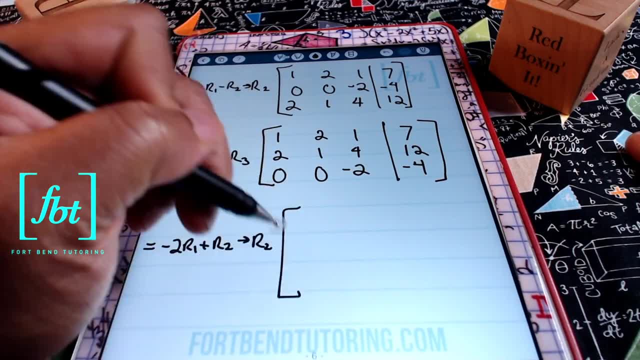 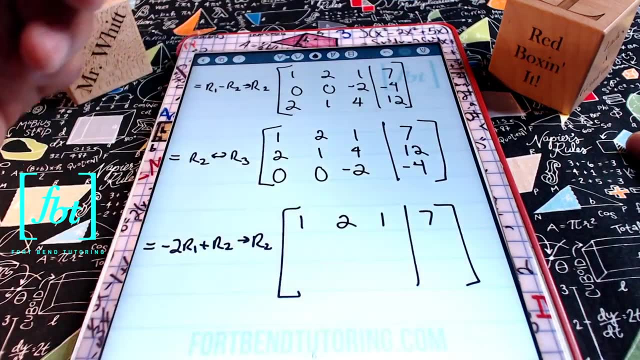 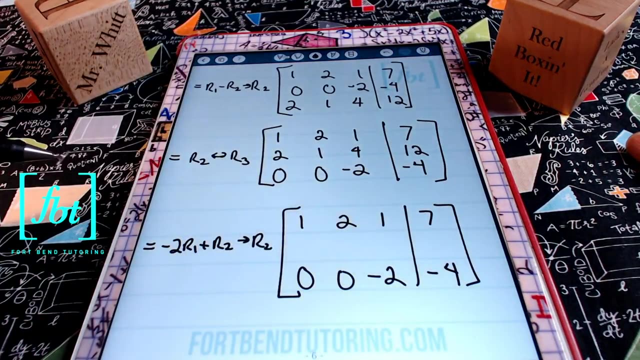 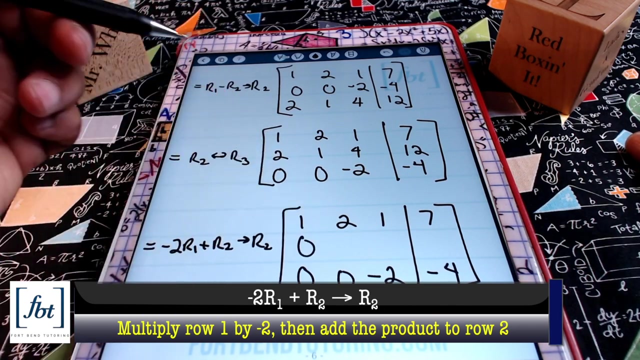 And row two. So that means that we now have row one remaining the same, again One, two, one and seven here, guys. And then the third row will stay the same: Zero, zero, negative two, negative four. And then I'm going to have negative two times one gives me negative two. Negative two plus two gives me zero. Then, multiplying negative two times two gives me negative four. Negative four plus. 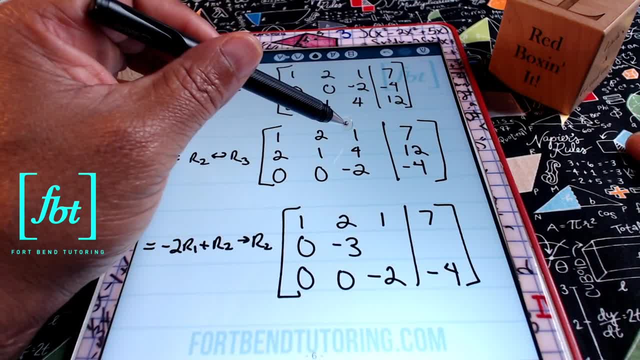 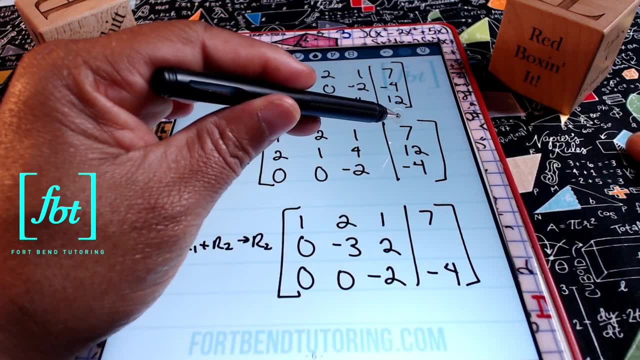 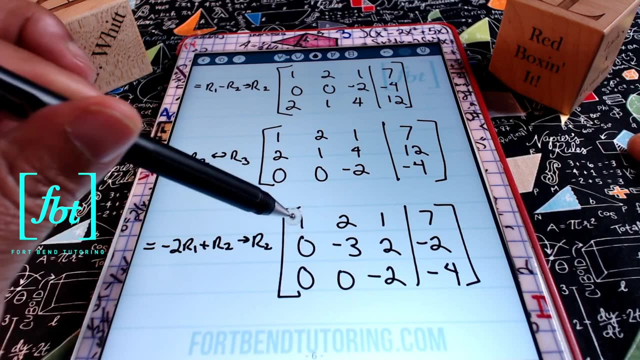 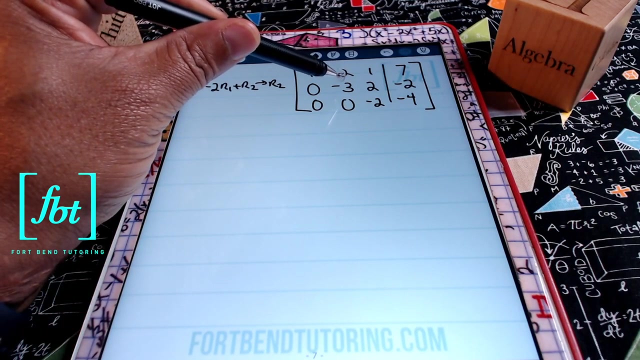 one gives me negative three, And then negative two times one gives me negative two. Negative two plus four is positive two, And then I'll have negative two times seven, which is negative fourteen. Negative fourteen plus twelve is negative two, And we have our resultant row. after our row operation here, Staying consistent, our next step is to make this negative three a one. So what I'll do then is I'm going to take row two and divide it by negative three. 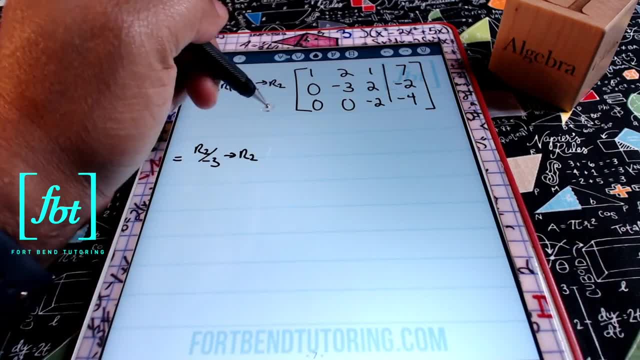 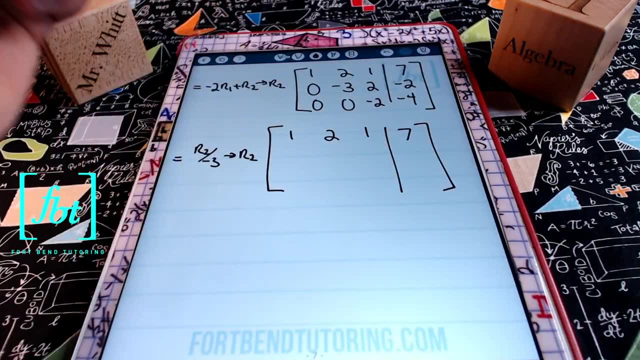 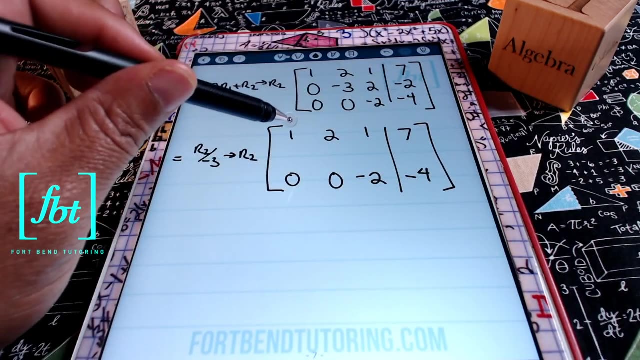 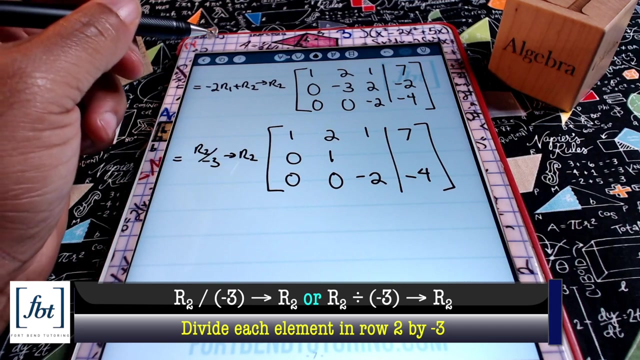 Putting the result in row two. So what this will look like is the first row remain the same, One, two, one and seven, And I'm going to go ahead and write out my third row, knowing that it won't be changed in this step here. Then, focusing on the second row: Zero divided by negative three is still zero. Negative three divided by negative three is one. Two divided by negative three is negative two thirds. And negative two divided by negative three is positive two. 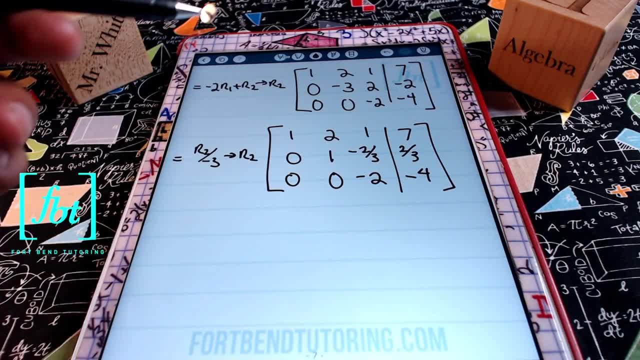 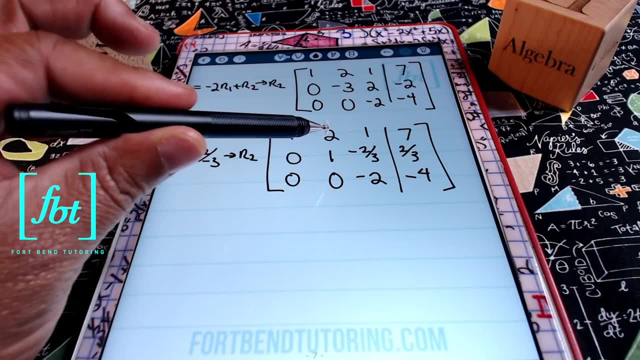 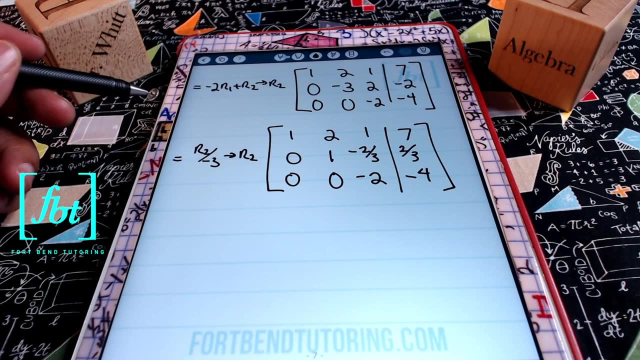 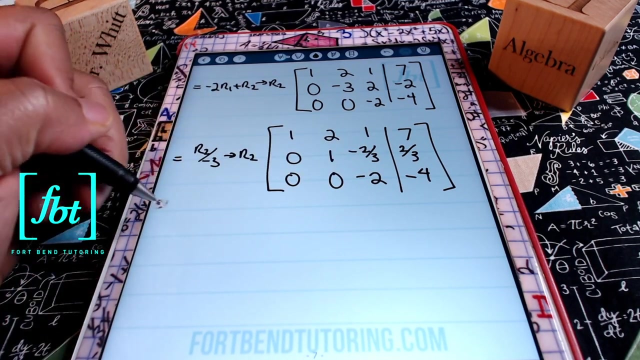 So this is what I end up with here, after dividing each and every element in row two by negative three. Remember, the purpose in doing so was to make sure that I ended up with a positive one on my main diagonal here. The last step that I'll need to do in order to put this matrix into row echelon form is to make the third row, third columns element a positive one. We can do that by dividing by negative two, So I'll have row three divided by negative two. 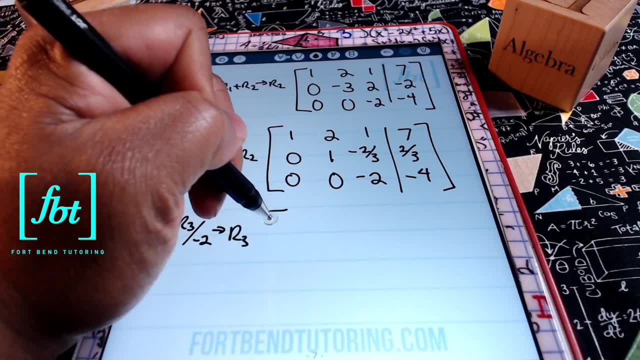 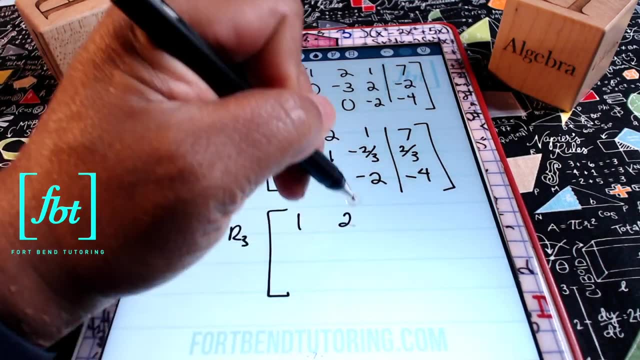 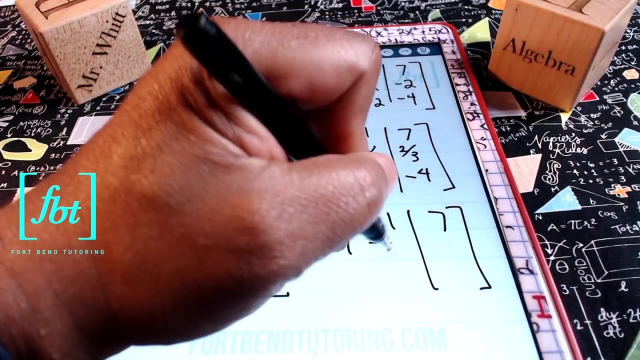 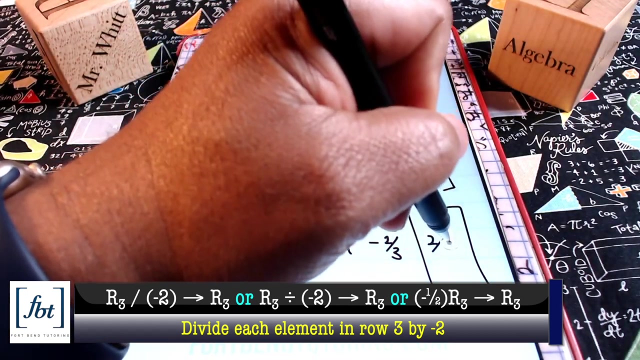 Placing the result in row three. So this is going to be my last step in order to put the matrix into row echelon form. So I'm going to bring down row one as one, two, one and seven. Then I'll have zero, one, negative two thirds as well as positive two thirds. I hate the two there, Let's fix the two. This is a better two. There we go. Then, in the third row, we'll be dividing each and every element by negative two. So zero divided by negative three is positive two. 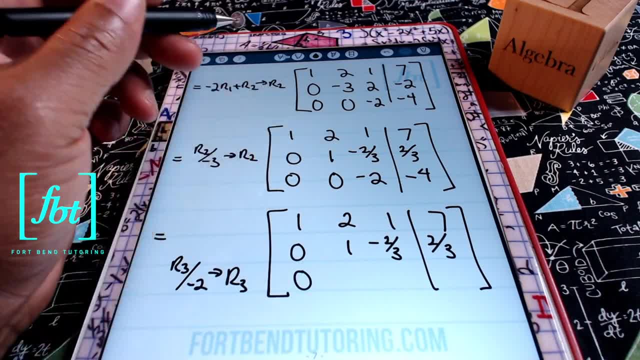 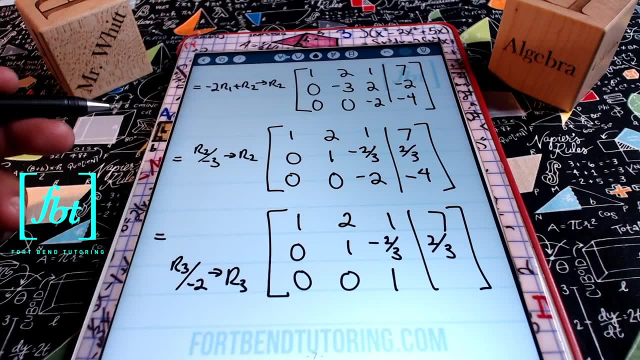 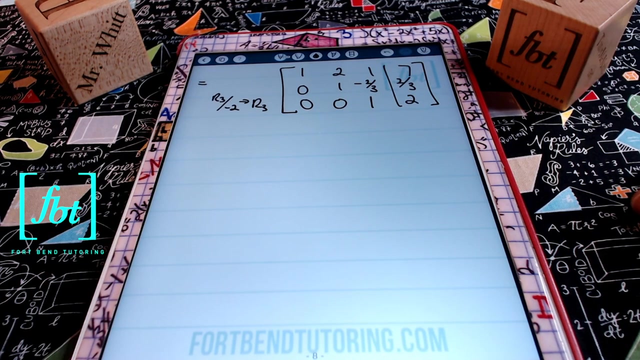 Zero divided by negative two is zero. Zero divided by negative two is zero once again. And then negative two divided by negative two is positive one, And negative four divided by negative two gives you two. There you have it. So now we have row echelon form guys with ones in the main diagonal, zeros underneath the main diagonal, And the next step is to back substitute. Continue on the process. We're going to be now back substituting into a system of equations, So I can rewrite this. 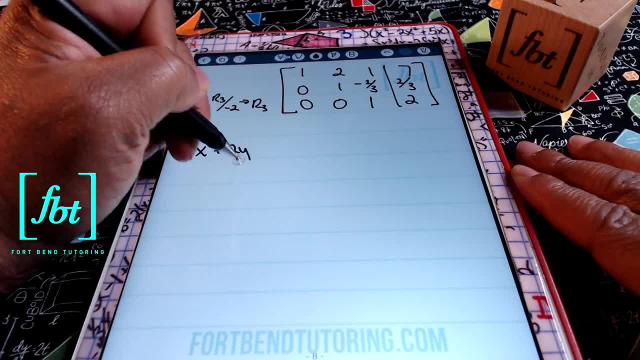 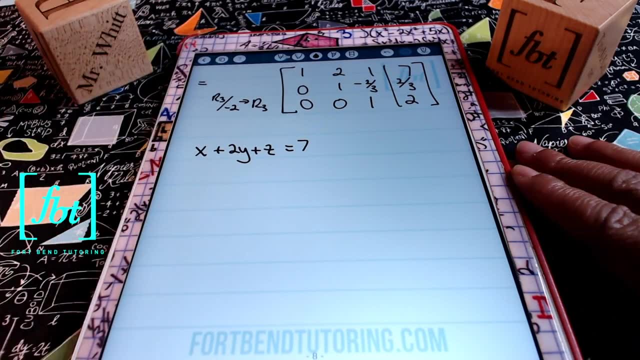 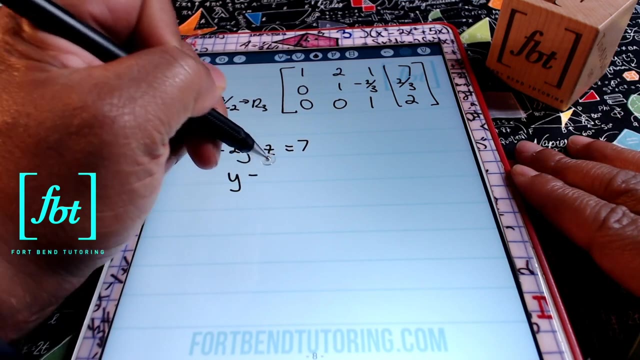 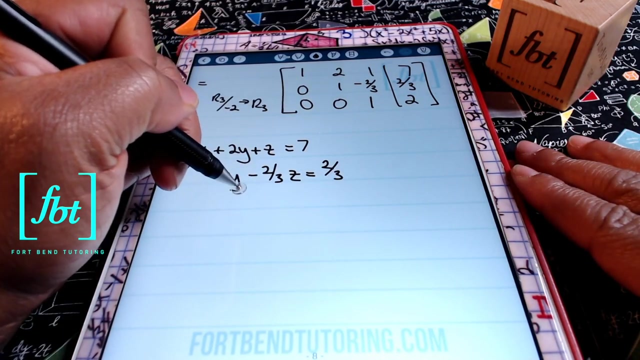 I can rewrite this as x plus two, y plus z equals seven. Then in the second equation, because this first term is zero, that means your coefficient on x is zero and you don't have to write zero x. You can simply write this as one y minus two thirds, z equals two thirds. And then for your last equation, you'll have z equals to two, And this will be your simplified system, written from your 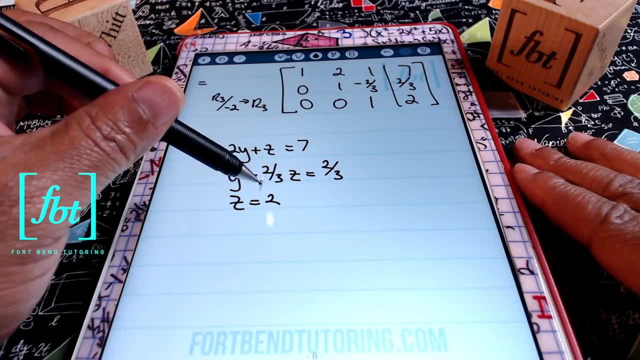 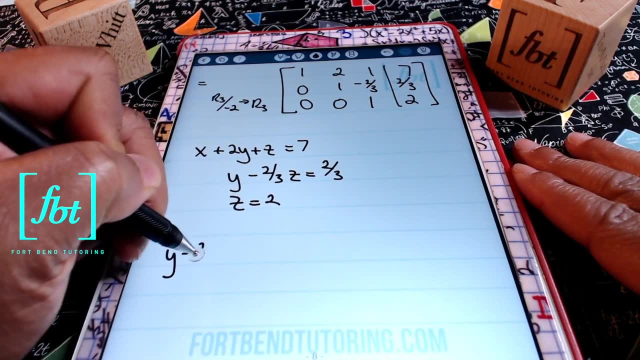 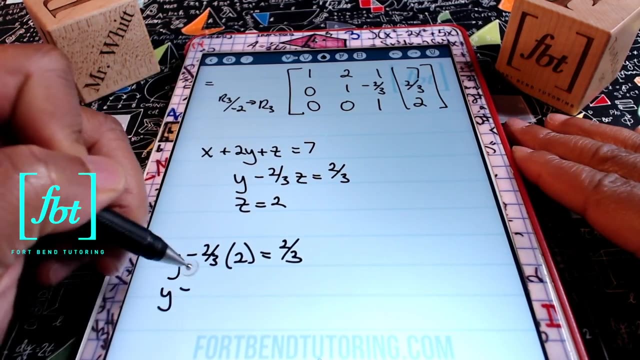 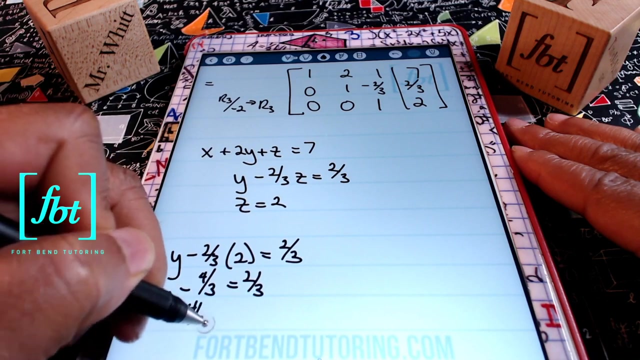 row echelon form. So since I know that z equals to two, now I can go ahead and plug that in to the second equation. So I'll have y minus two thirds times two equals to two thirds. From here we'll have y minus four thirds equals two thirds. So I'm going to be adding four thirds to both sides And that gives me y equals. 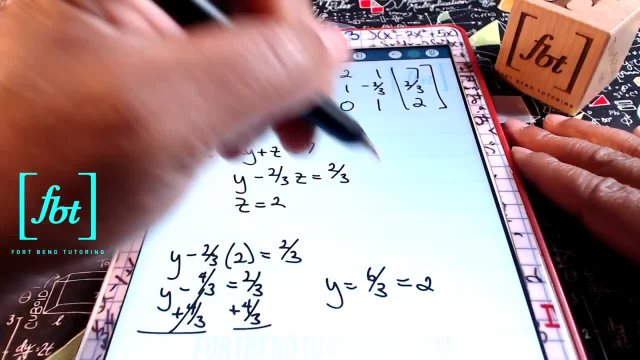 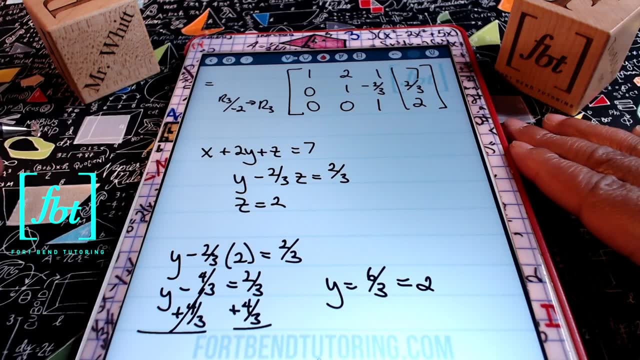 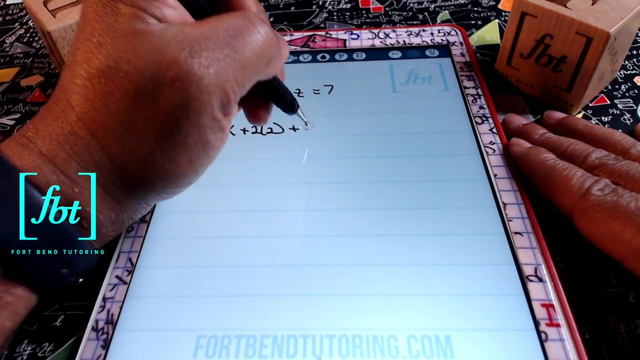 six thirds. When I simplify six thirds, I'll get two. So for now I know that z equals to two and y equals to two as well. So finally, we'll be plugging in z equals to two and y equals to two into this first equation from our system. So now that we know what y and z is, we'll be plugging it in to get x plus two times two plus two equals seven. Multiplying two times two gives you four, right. 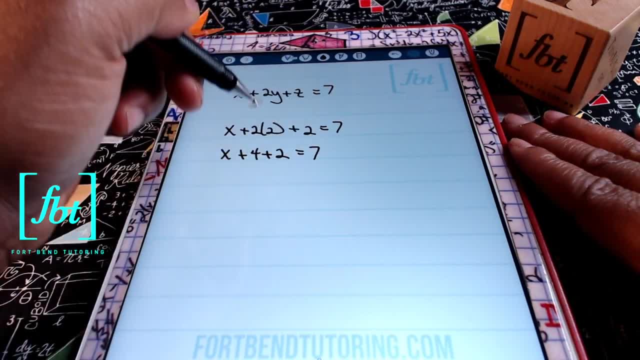 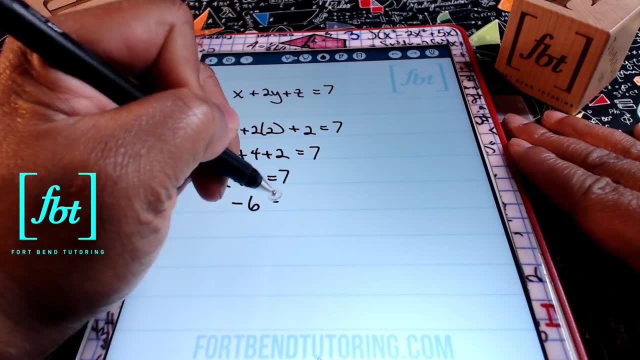 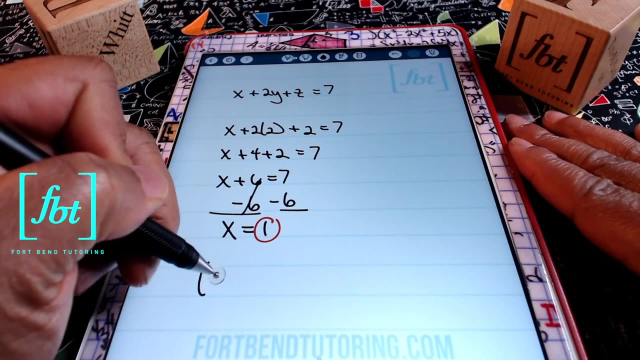 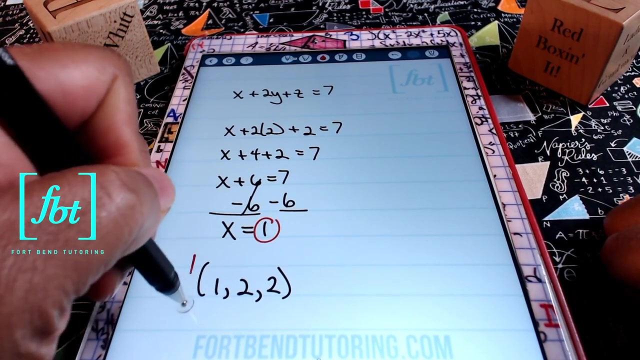 And we'll have: x plus four plus two equals seven. Combining our terms on the left side of the equation we'll have: four plus two gives us six. And then finally, subtracting six to both sides of the equation, we'll find that x equals to one. Therefore, our solution, written as an order triple, is going to be one, two, two. And this is our answer, Red box, it. That's right, guys. So now that we know that our value of x equals to one, our value of y is two. 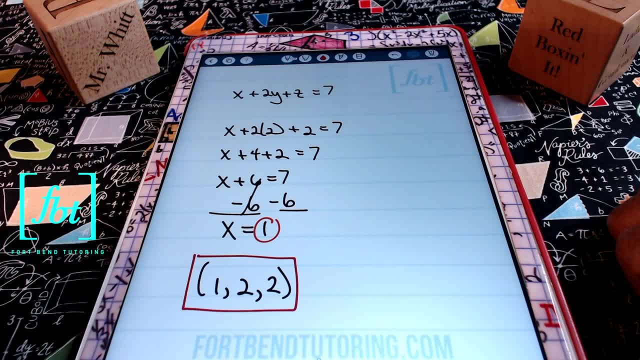 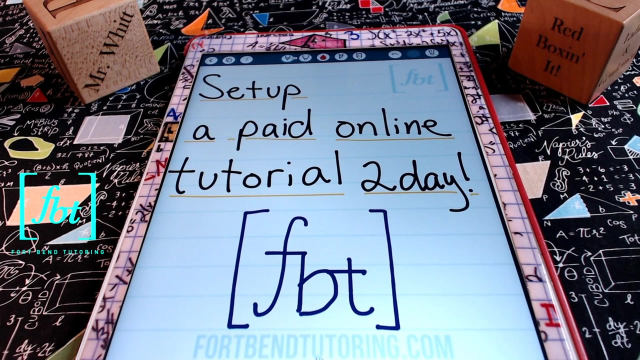 And our value of z is two. This is the order triple, which is your answer. Once again, you could expand this by saying x equals to one, y equals to two and z equals to two, But this is a preferred and standard way of writing your solution as well. All right, That was problem number two. All right, So I want to remind you guys that you could set up a paid online tutorial today with me, Mr Witt and Fort Bend tutoring by going to our Web site, Fort Bend tutoring dot com. 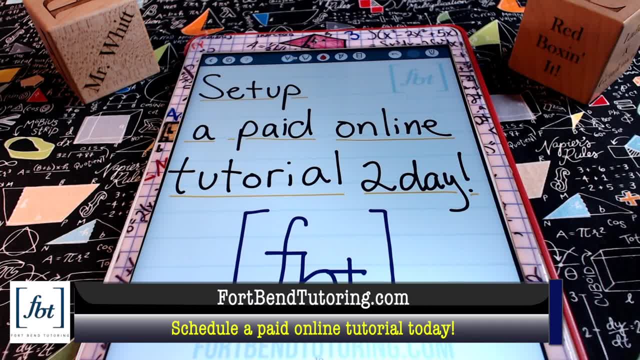 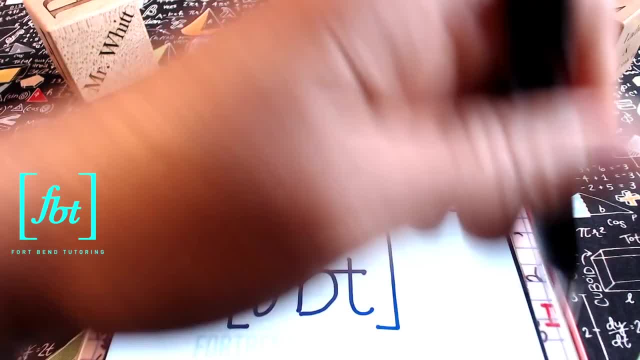 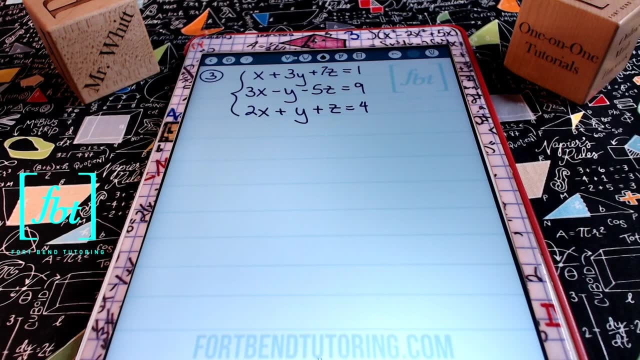 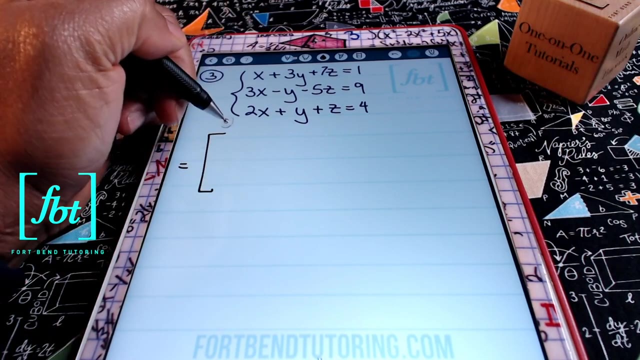 There you'll find links and resources to different math material, as well as links to our merchandise. All right, So let's go ahead and get back to business with problem number three. All right, With problem number three, we have another system with three equations and three variables. We know that our first step is to rewrite this as an augmented matrix, So that's exactly what we're going to do. All right, So that means that I have coefficients one, three, seven, as well as one. 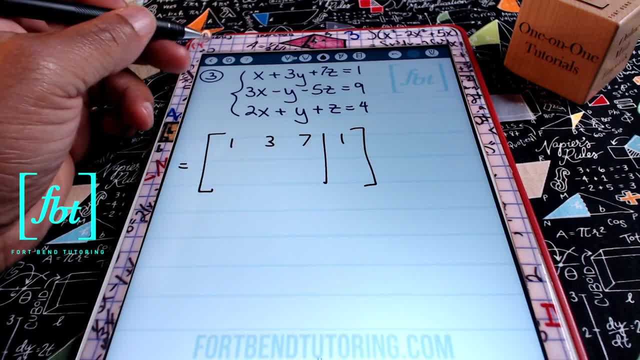 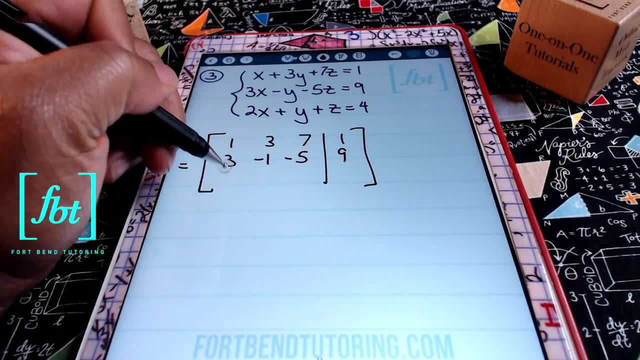 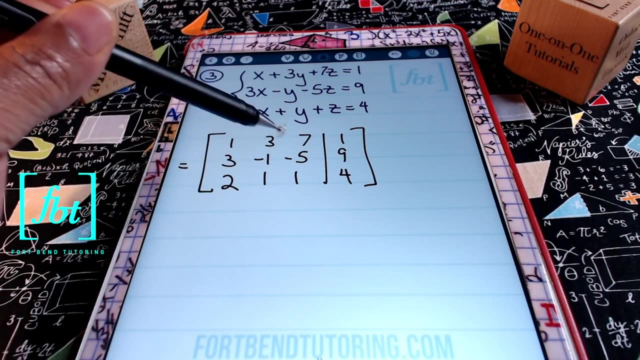 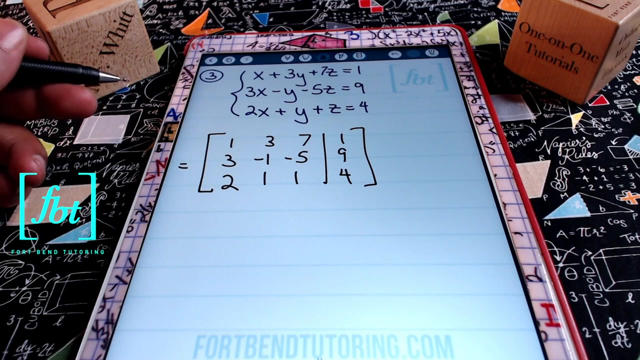 On the right side of our augmented matrix we have in the second row three negative one negative five and nine, And then finally we'll have two, one, one and four. So we'll be keeping in mind that we want this main diagonal to be filled with ones with zeros underneath the ones. OK, So that means in my first step here, after writing the augmented matrix, I'm going to focus on getting zeros in that first column, underneath that first row. 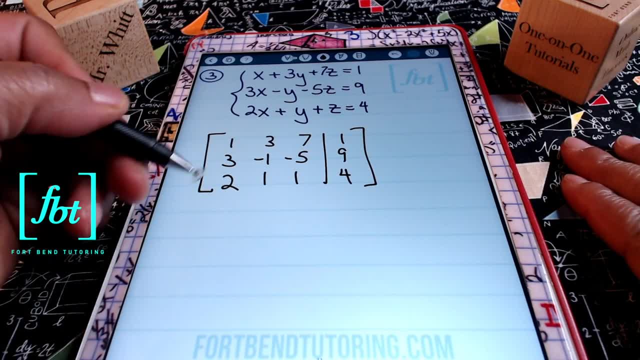 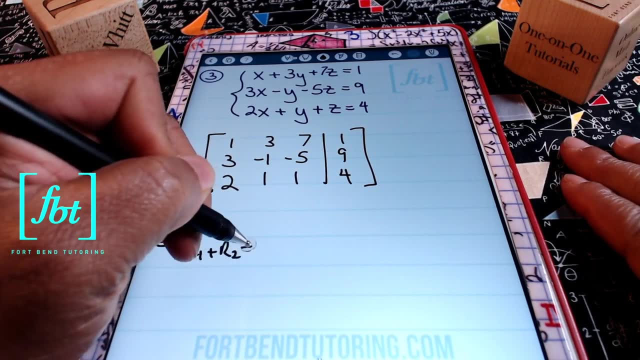 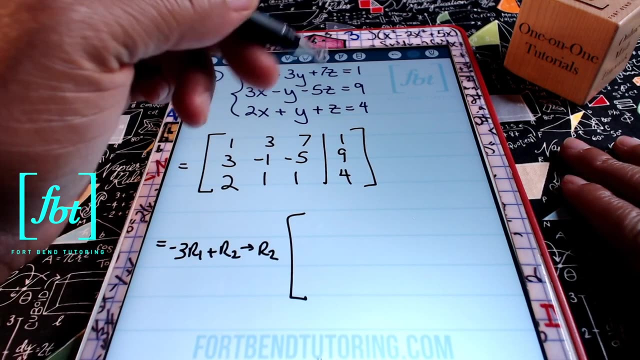 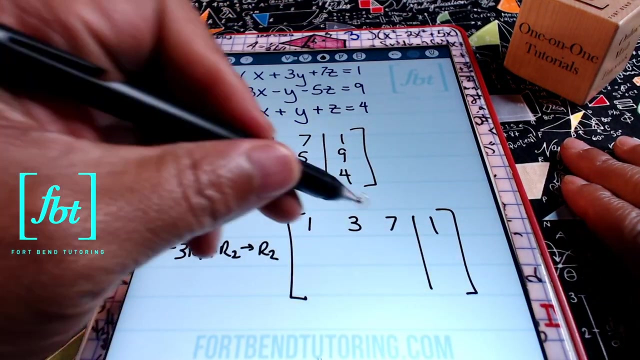 So I'm going to do the following row operation: I'm going to have negative three times, row one plus row two and putting the result in row two. From here I know that my first and third rows are going to go unchanged, So I'll just bring those down. We'll have one, three, seven and one in the first row, and in the third row we'll have two, one, one and four. Then, following our 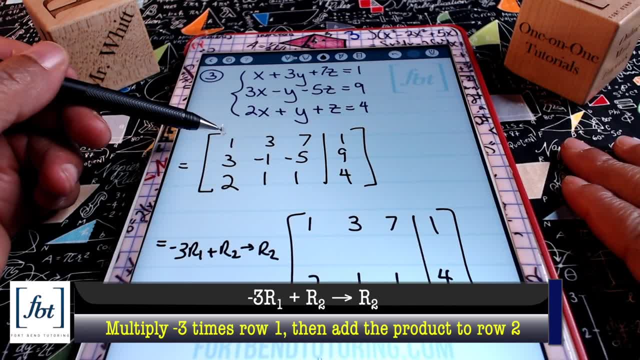 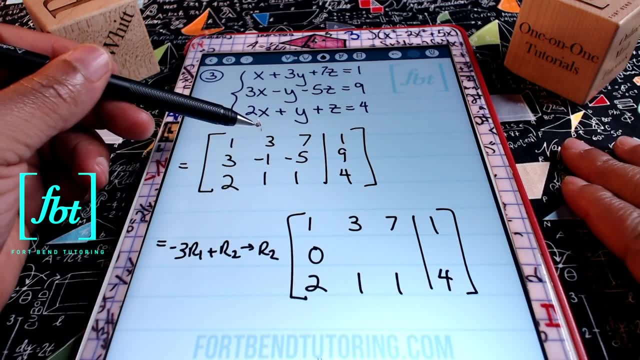 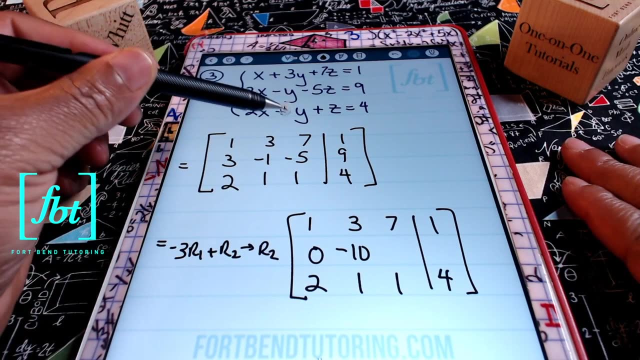 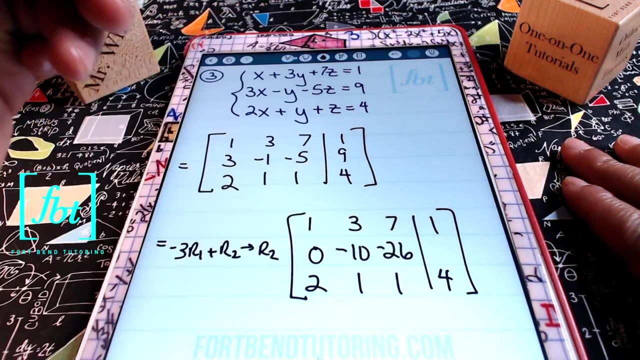 row operation, I'll have negative three times one gives me negative three, and then negative three plus three gives me zero. here, Moving on to the next element, we'll have negative three times three gives me negative nine. negative nine and negative one give me negative ten. Then I'll have negative three times seven gives me negative twenty one. negative twenty one and negative five give me negative twenty six, and then negative three times one is negative three. negative three plus nine gives me positive twenty six. 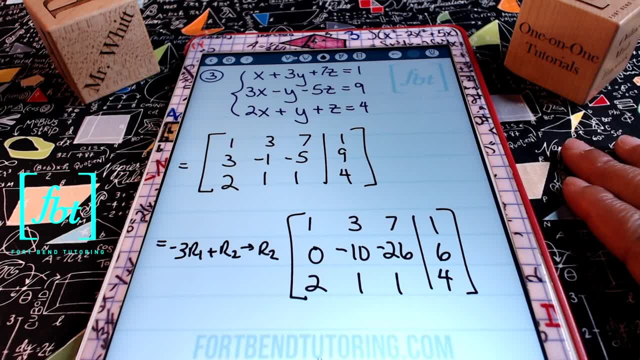 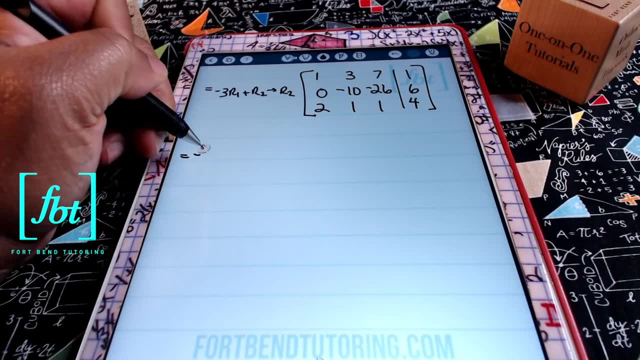 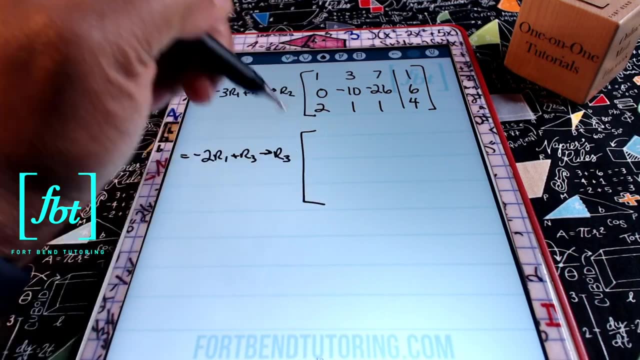 positive six. And this is what I have now for my new row two. Our next step is to create a zero for the third row, first element. That means I'll be doing the following row operation: I'm going to have negative two, row one plus row three, putting the result in row three. So it'll look. 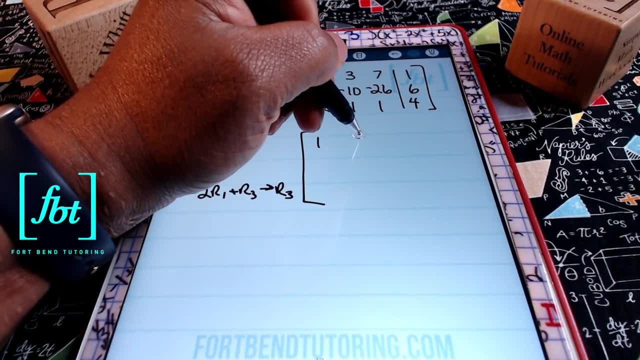 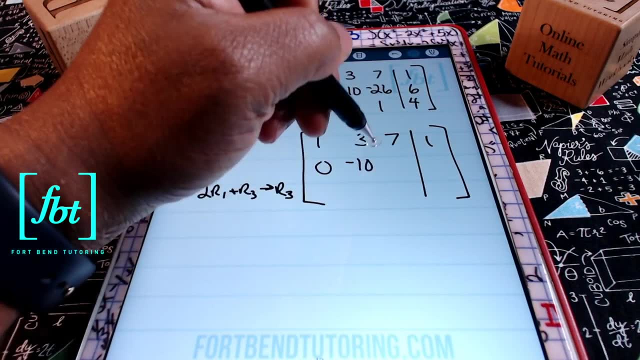 like this: This first row will remain the same. We'll have one, three, seven and one here. The second row remains the same. We have zero, negative 10, negative 26, and six. However, the third row. 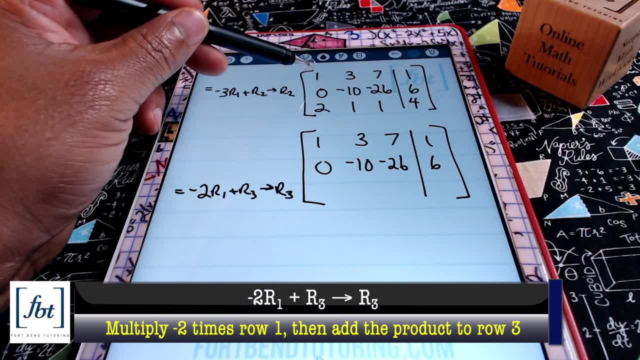 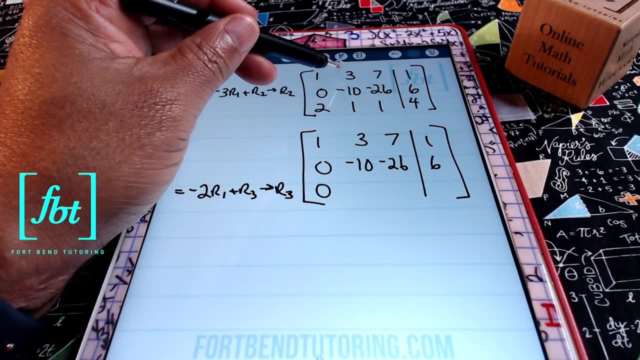 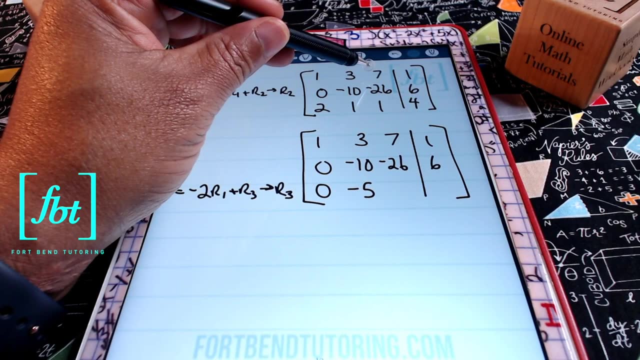 will first multiply negative two times one to get negative two. Negative two plus two gives us zero. Then, multiplying negative two times three, you'll have negative six. Negative six plus one gives you negative five. And then negative two times seven gives you negative 14.. Negative 14 plus one gives 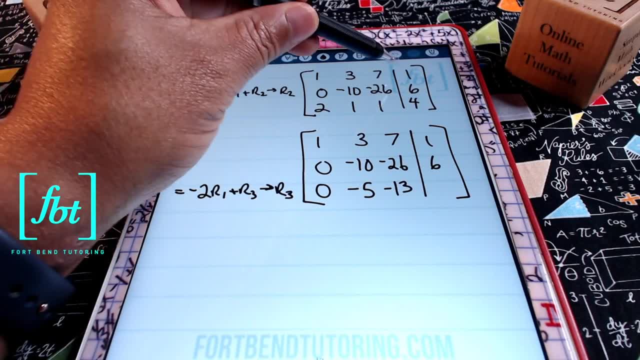 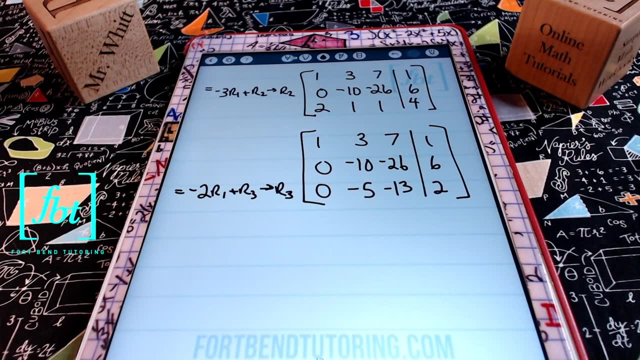 you negative 13.. And then negative two times one is negative, two Negative two plus four gives me two. So this is going to be our new third row for our row equivalent matrix. The next thing I want to do is I want to create 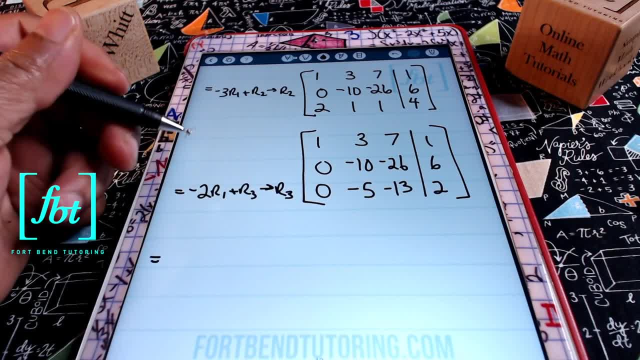 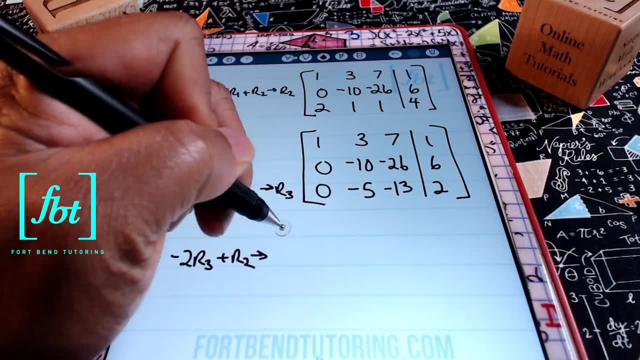 a zero where this negative five is. So I'm going to be doing the following: I'm going to have negative two, row three plus row two, placing the result in row three. What does that mean for me? That means that my first and second 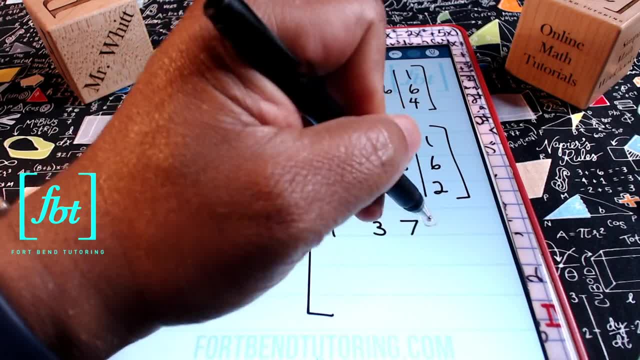 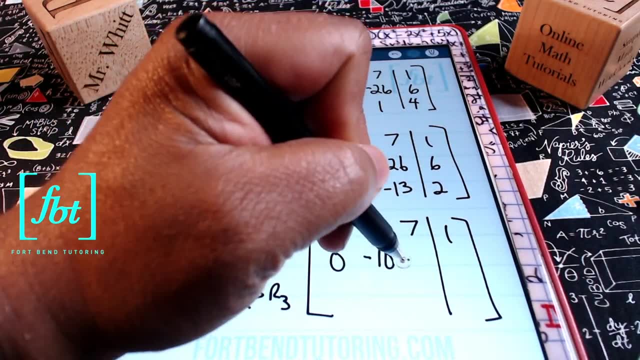 rows will remain the same. I'll have one, three, seven and one for that first row, Then for the second row we'll have zero, negative 10, negative 26, and six, And then finally to get our third row. 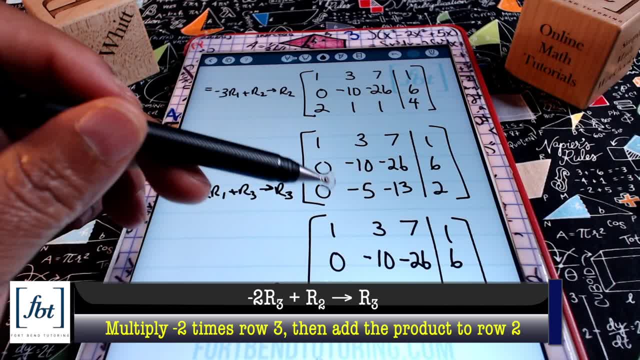 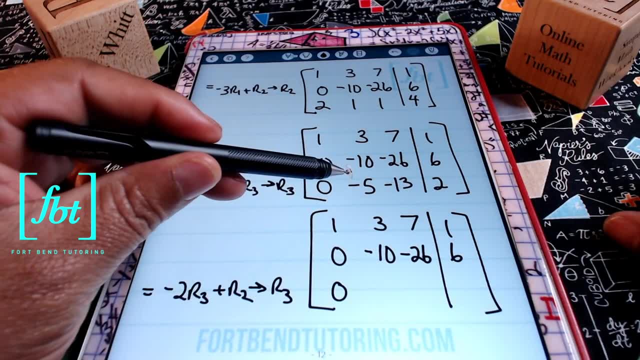 we're going to be multiplying row three times negative two and then adding it to row two, So we'll have negative two times zero plus zero gives you zero. Then negative two times negative. five is 10.. 10 and negative 10 combined. 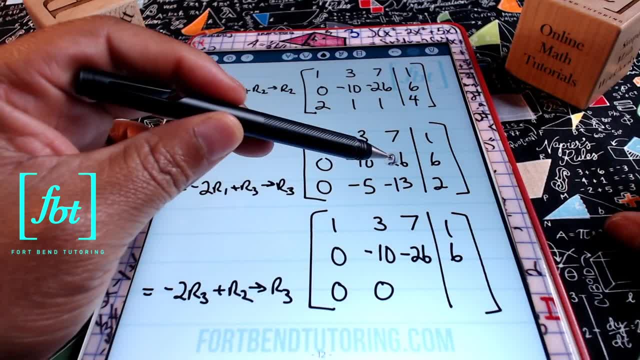 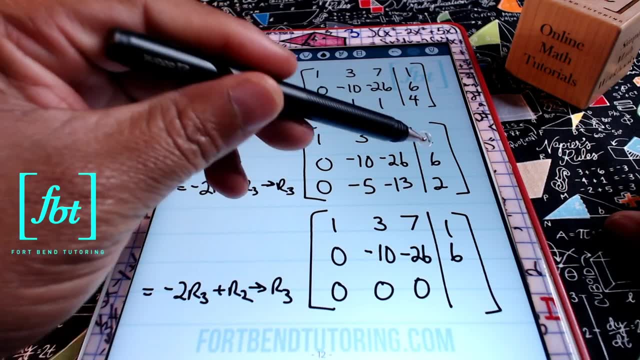 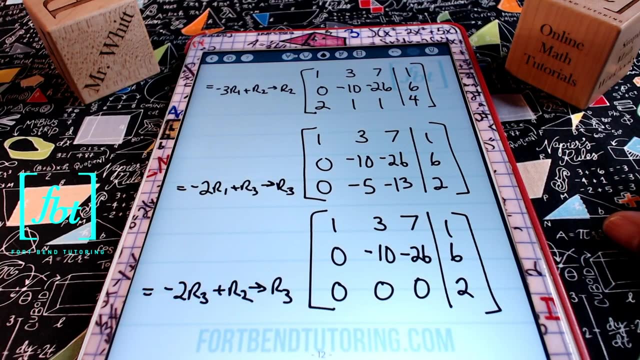 To give you zero. Multiplying negative two times negative 13,, you'll have 26.. 26 and negative 26 gives you zero. Then, multiplying negative two times two gives you negative four. Negative four plus six gives you positive two. It's at this point we're going to stop. The reason why we're stopping is: 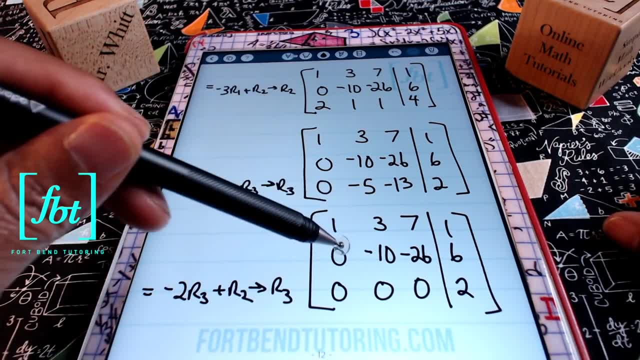 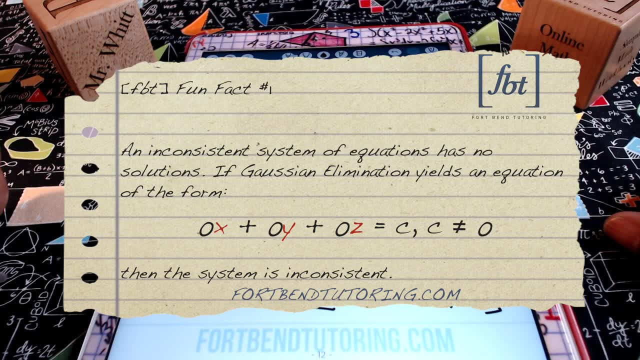 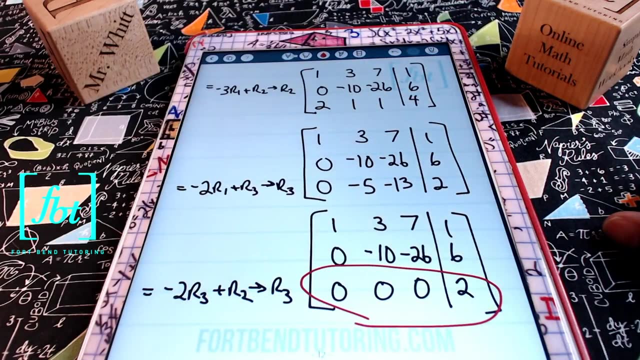 because anytime your Gaussian elimination yields an equation in the form of 000, with a non-zero number, well, in that case you're going to end up with an inconsistent system, which means there's no solution to this system. So, due to this equation right here, due to this zero X plus zero Y plus zero Z equals to two. 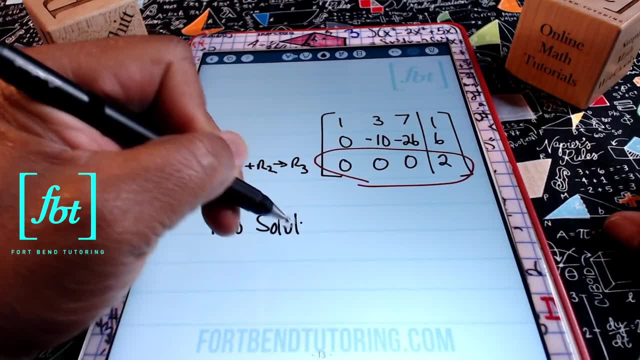 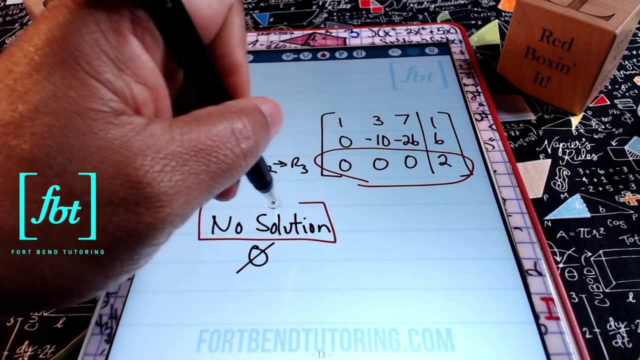 the answer is no solution, Just like this, guys. Or you can say: it's the empty set, Okay, Red box it, people, There you go. So this system has no solution. Done and done, And once again it's called an inconsistent system. 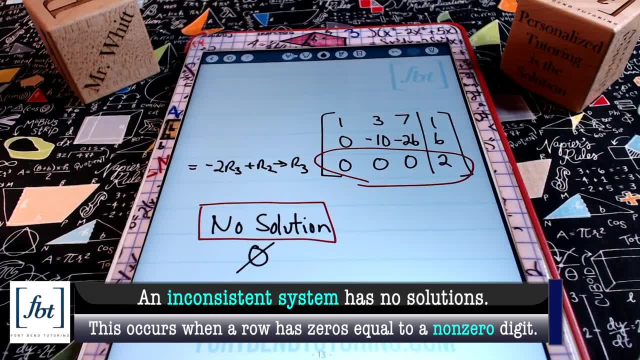 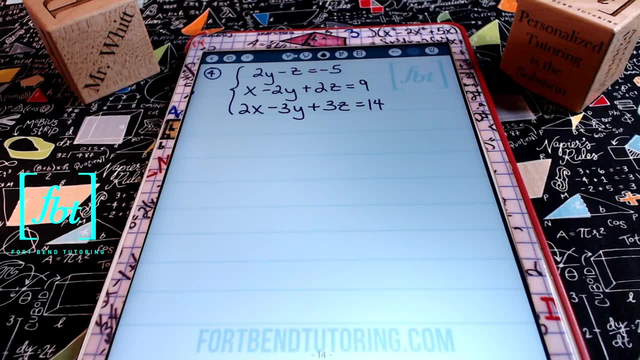 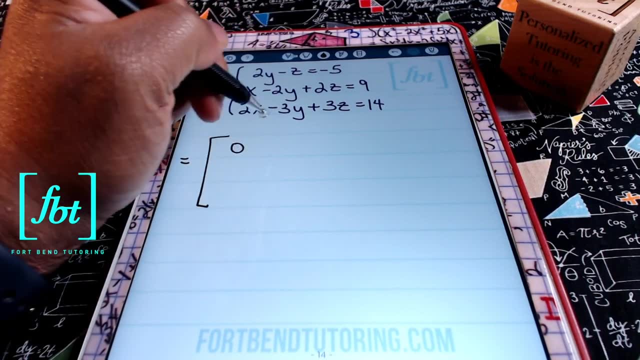 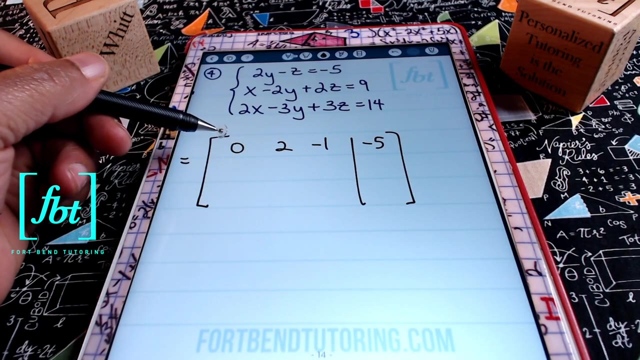 It is the system of equations that has no solution. Moving on to problem number four, In problem four we once again have a three equation, three variable system. So let's begin with our augmented matrix. So what we'll end up with is 0, 2, negative 1 and negative 5.. Notice that we did not have an X term. 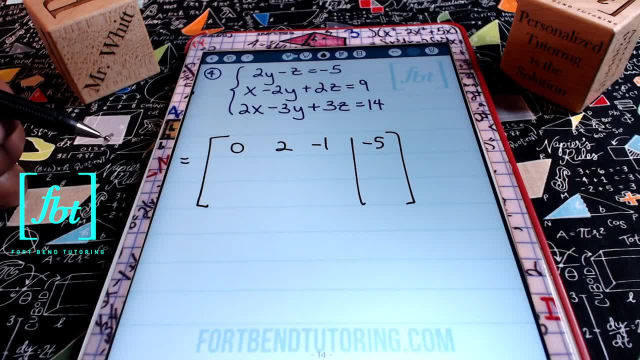 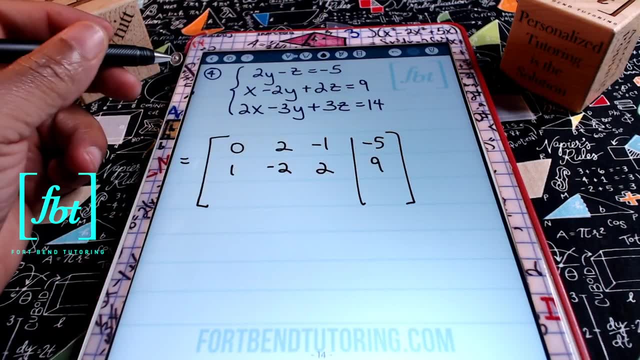 in that first equation. That's why I put zero as its coefficient. Then in the second row, have 1, negative, 2,, 2, and 9.. The third row will have 2, negative, 3,, 3, and 14.. And with this setup, 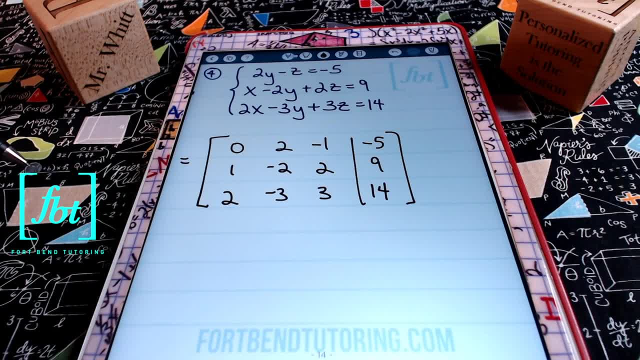 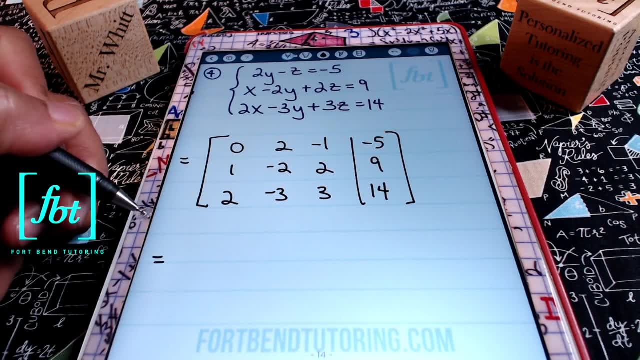 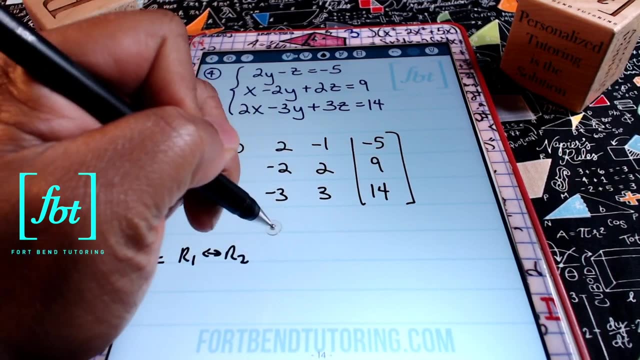 guys, we're going to go ahead and solve this system, knowing that we want our main diagonal to have ones with zeros underneath that main diagonal. So I'll begin with the following row operation. I'm going to start with swapping out row 1 with row 2.. That's going to be my first move. 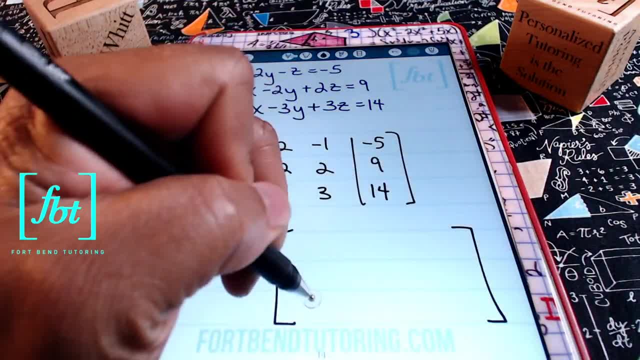 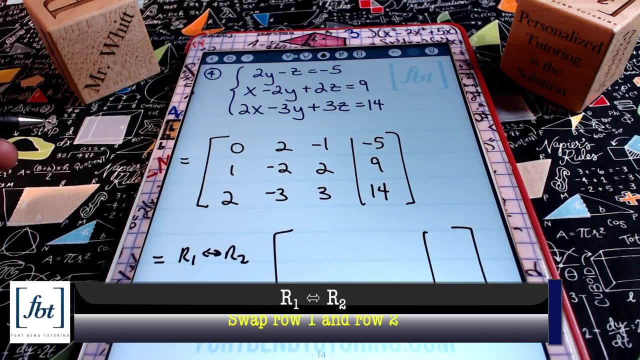 That means that row 3 will remain the same. You'll have 2, negative 3,, 3, with 14 on the right side of our augmented matrix here. Then our new first row will be 1, negative 2,, 2, and 9.. 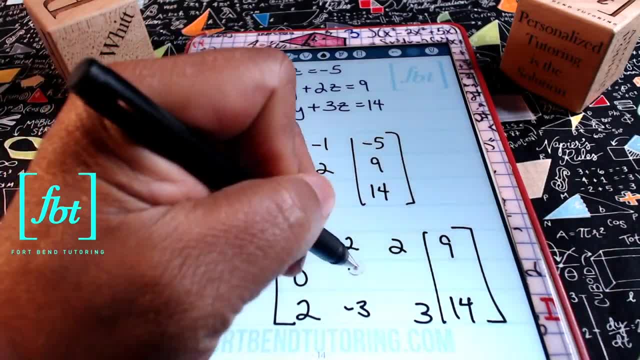 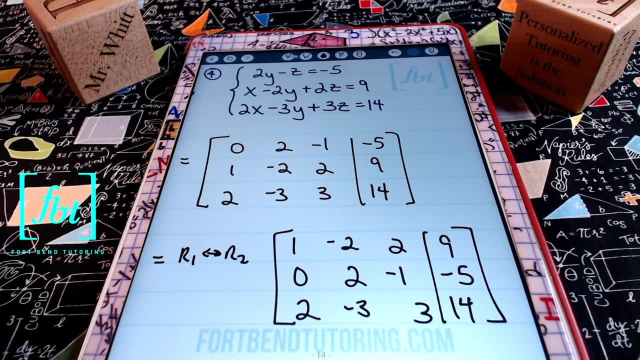 Where our new second row will be 0,, 2, negative 1, and 9.. And this is going to be our row equivalent matrix that we have thus far. With our next step, I'll want this 2 to become a 0.. So my row operation is going to be: 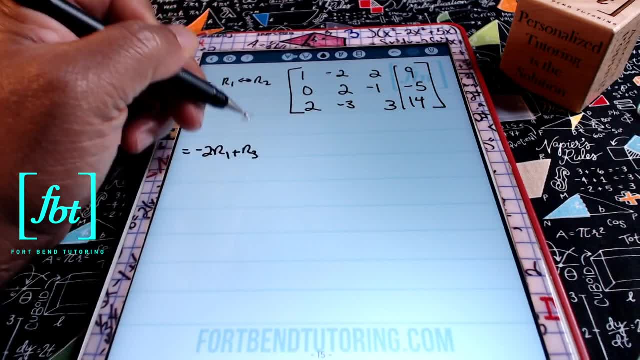 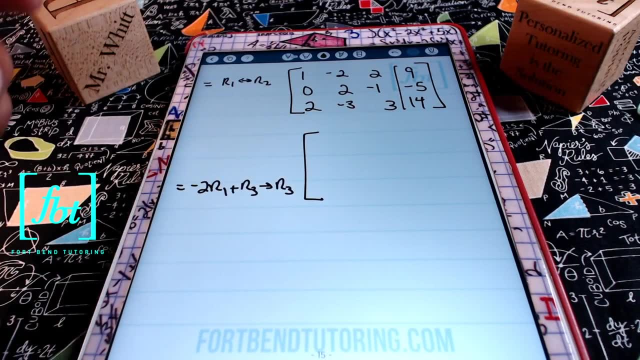 negative 2, row 1, plus row 3.. Putting the result in row 3.. So from here, my first two rows will remain the same, So that means that I'll bring down 1, negative 2,, 2, and 9.. 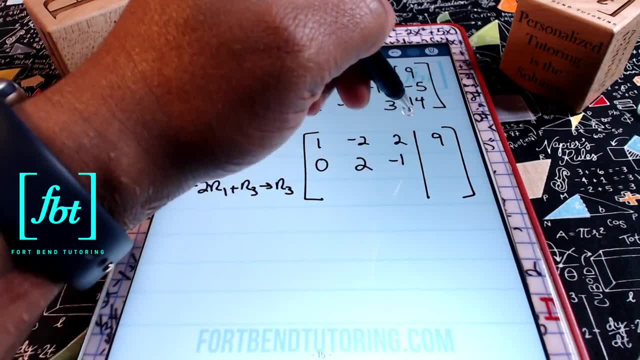 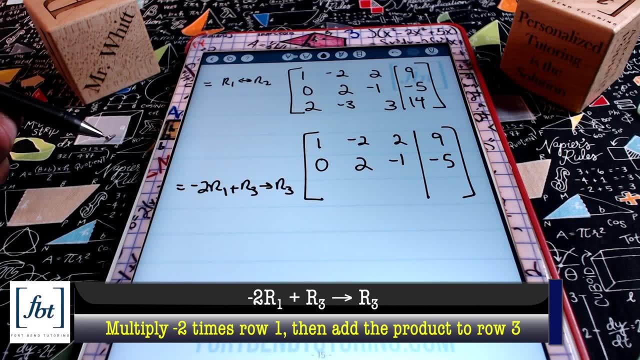 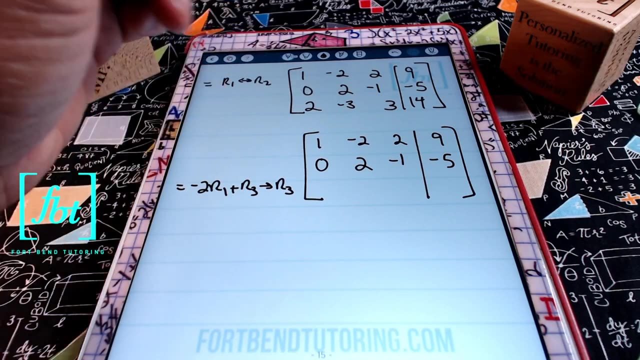 As well as 0,, 2, negative 1, negative 5.. For this third row, however, we'll multiply negative 2 times row 1, then add that to row 3, and then write the result in row 3.. So negative 2 times 1 is negative 2.. Negative 2 plus 2 gives me 0.. 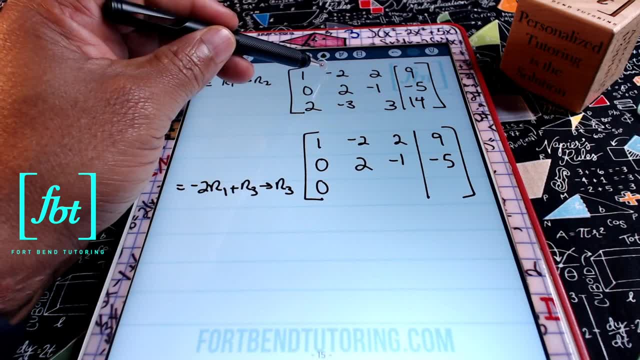 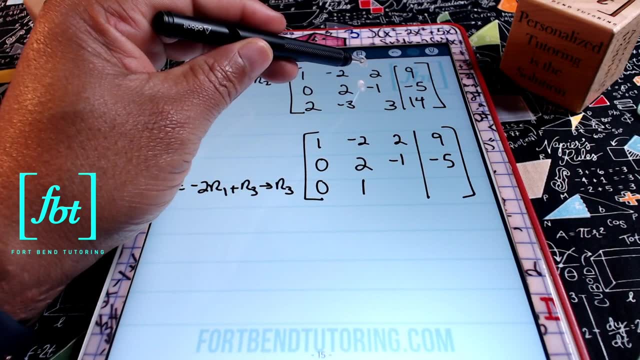 Then multiply negative 2 times negative 2 to give me positive 4. Positive 4 and negative 3 combine to give me positive 1. Then we'll have negative 2 times 2, that's negative 4. Negative 4 plus 3 gives me. 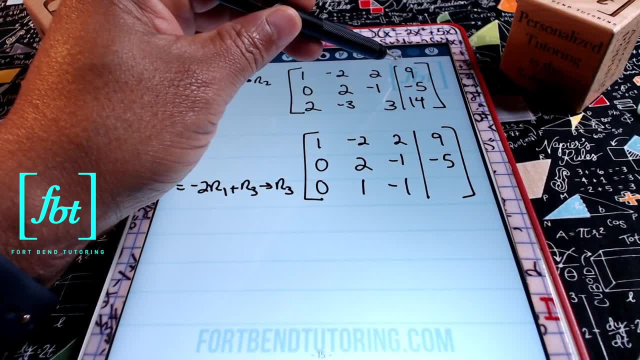 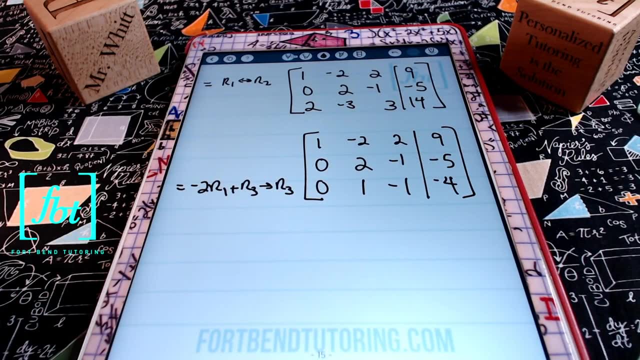 negative 1, and then we'll have negative 2 times. 9 is negative, 18 negative 18 and 14 combined to give me negative 4. all right, and this is going to be the resultant matrix after that row operation. the next thing I want is I: 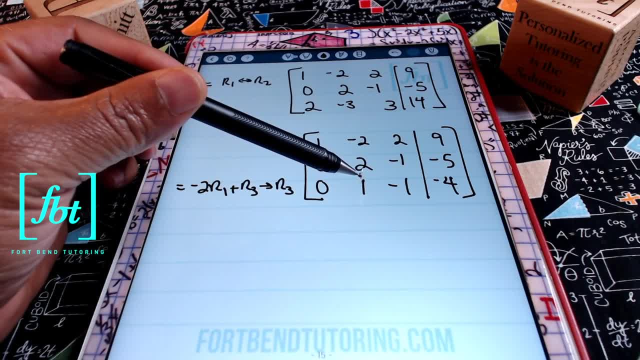 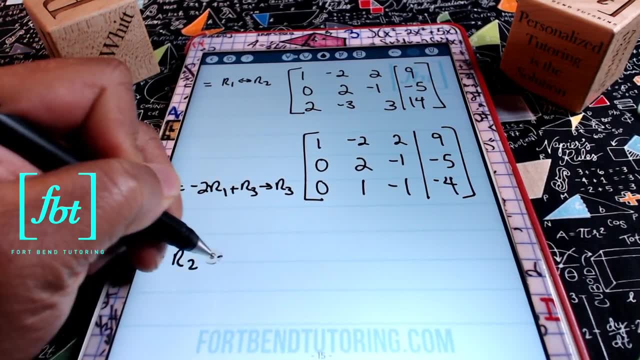 want this term here to be a 1, and it looks like I already have a 1 element right here, so maybe we should swap again. guys, let's go ahead and swap out row 2 and row 3 together. okay, so with this swap, I'm gonna end up with the first row. 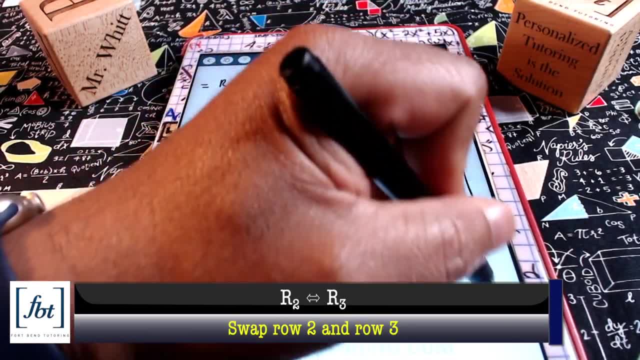 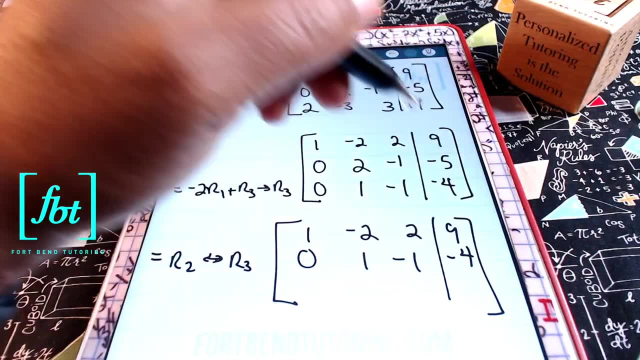 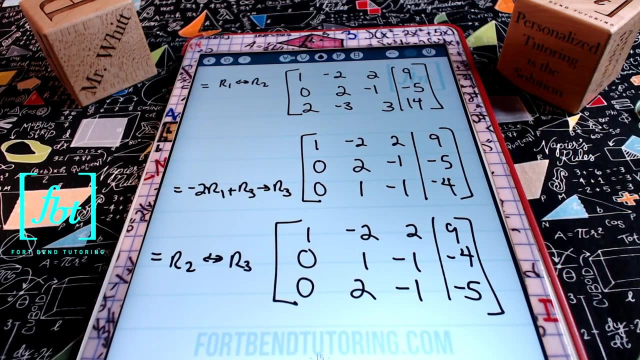 being the same, just like this, and then my second row now being 0, 1, negative 1 and negative 4, while the third row is 0, 2 negative, 1, negative 5. all right, so I don't try to predict too much when I'm doing the Gaussian elimination process. 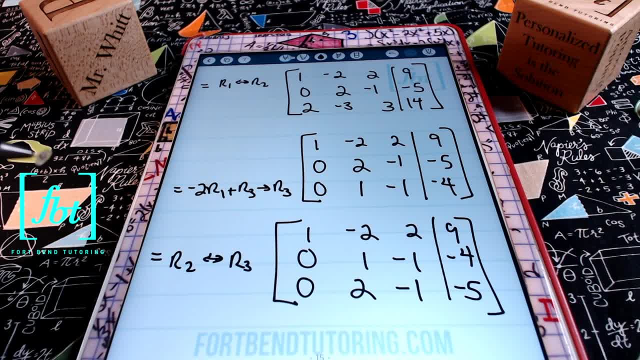 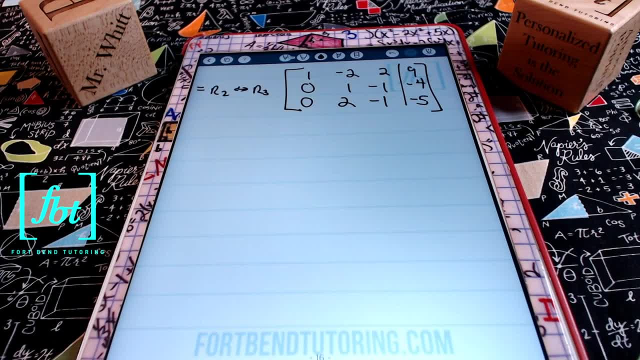 guys, I just take the steps as they come, okay, so I'm going to go ahead and do that, and I'm going to go ahead and do that, and so I just saw that this was going to be a better situation for me as far as getting my main diagonal to be ones. so that's what I wanted from here. I want to. 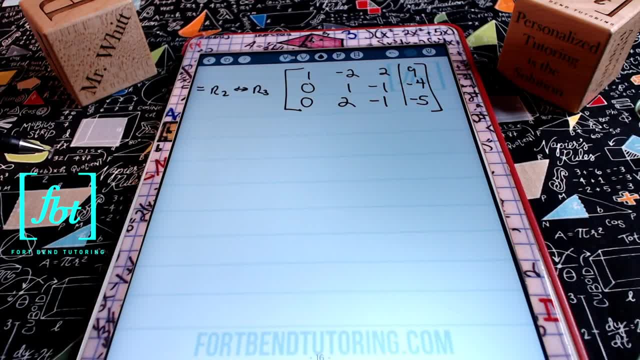 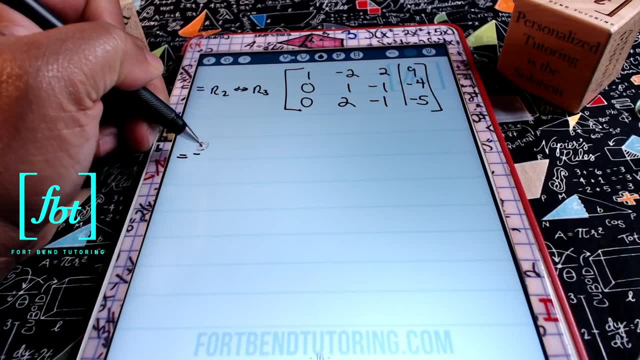 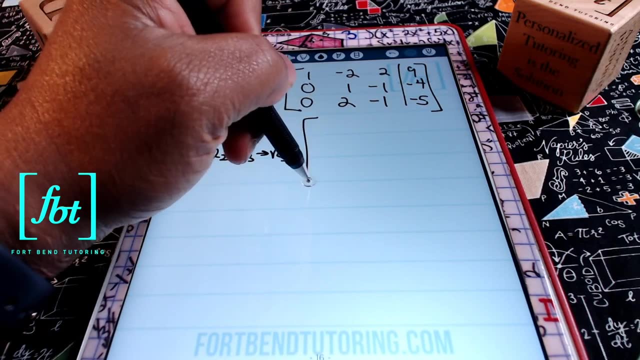 get a 0 right here in the third row, second column, where that 2 is. so the row operation that will help me do that is going to be for me to have negative 2, row 2 plus row 3, putting the result and row 3. so in doing that I'll be bringing 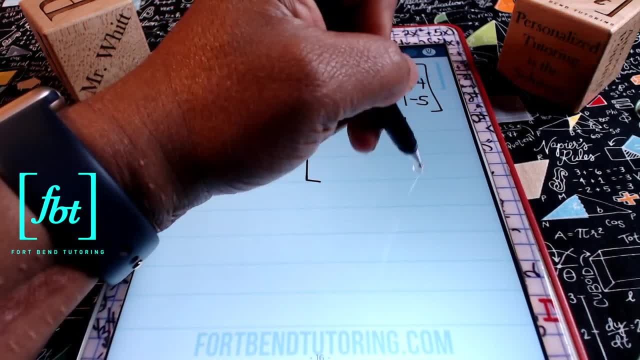 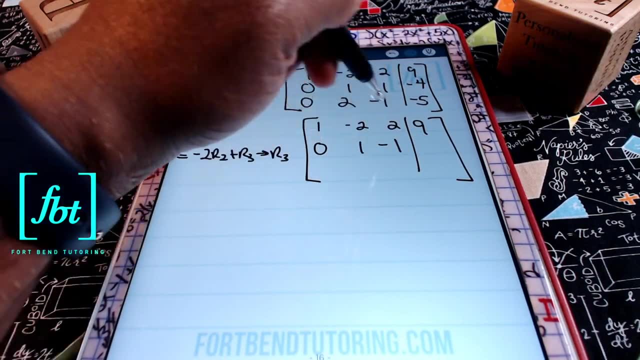 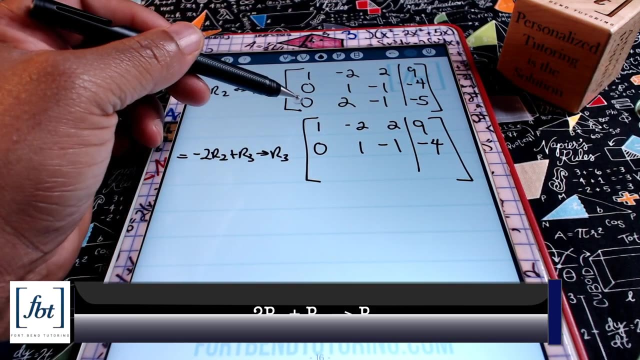 down the first row- 1, negative 2, 2 & 9, and then I'll bring down the second row as 0, 1, negative 1 and negative 4, and then for that third row, I'm going to be multiplying the second row by negative 2, adding it to the third row, so i'll have negative 2 times 0 to. 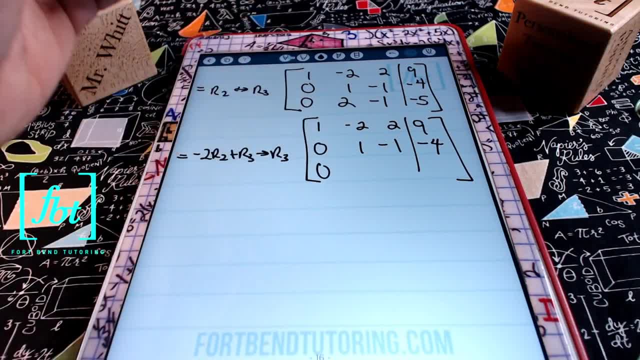 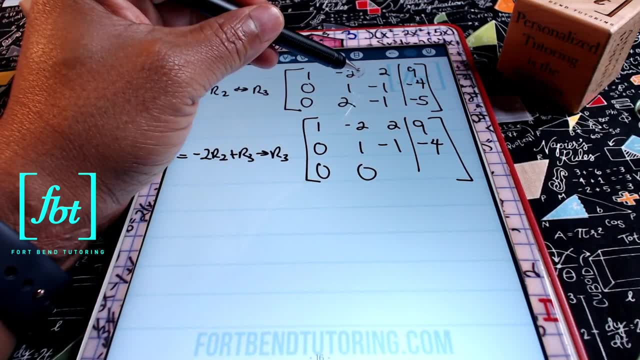 give me 0 and 0 plus 0 is 0. negative 2 times one is negative 2. negative. 2 plus 2 gives me 0 and then Negative 2 times negative, 1 is positive 2.. Positive 2 and negative 1 combine to give me positive 1.. 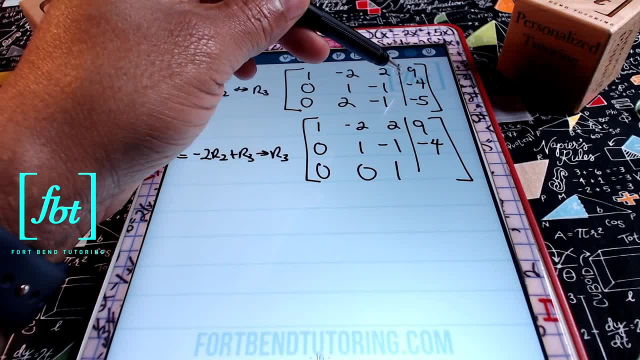 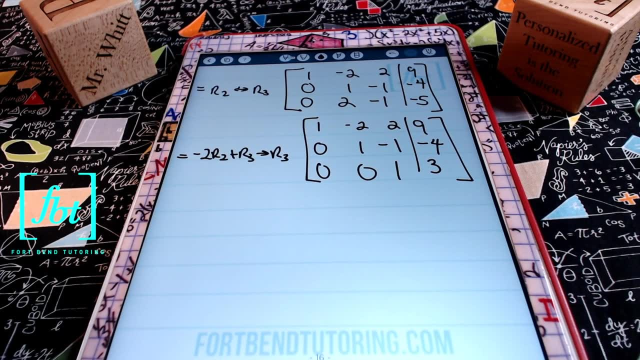 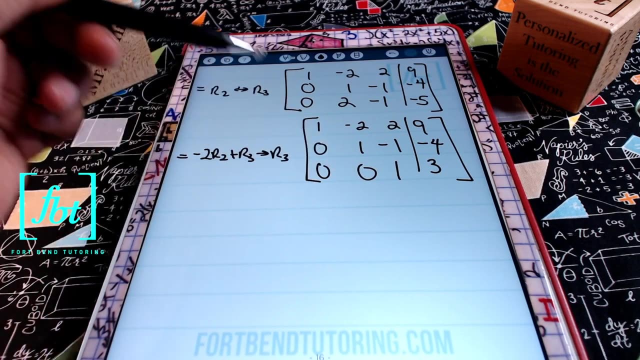 And then finally, negative 2 times negative, 4 is positive 8.. 8 and negative 5 combine to give me positive 3.. And now we have our matrix in row echelon form. Notice how my main diagonal is all 1s and I have 0s underneath that main diagonal. 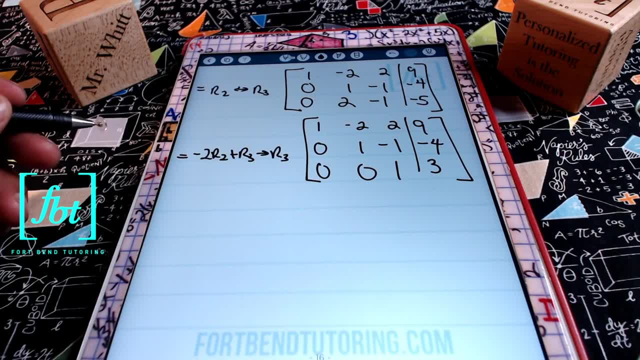 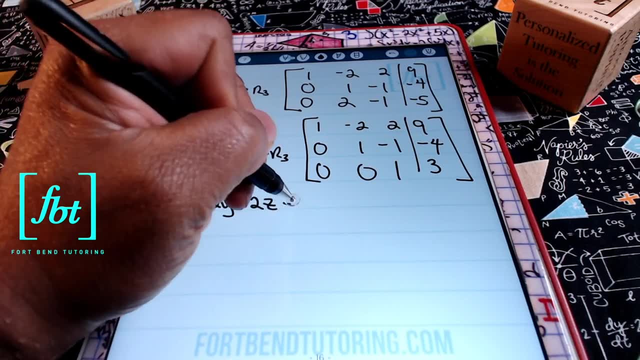 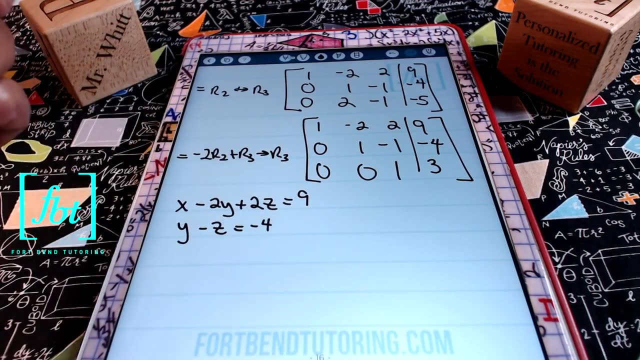 That means that it's time to back substitute guys, So I'll be rewriting my equations as x minus 2y plus 2z equals 9.. While the second equation will be: y minus z equals negative 4.. And finally, the third equation is z equals to 3.. 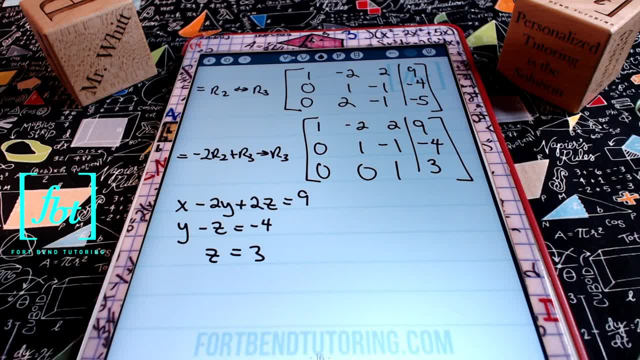 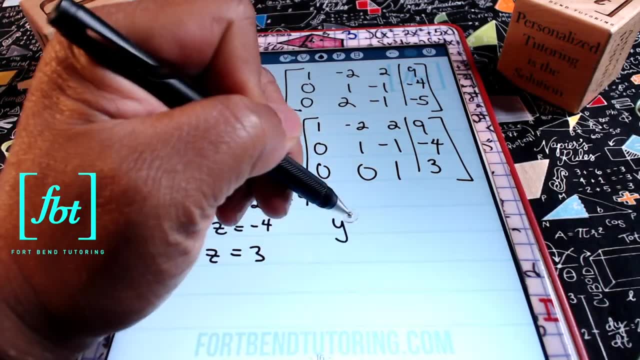 And now, using this simplified system, we can solve for the system of equations much easier. So we already know that our z value is 3, right, And plugging that into the second equation, you'll have y minus 3.. And then we'll have z equals to 3, equals negative 4.. 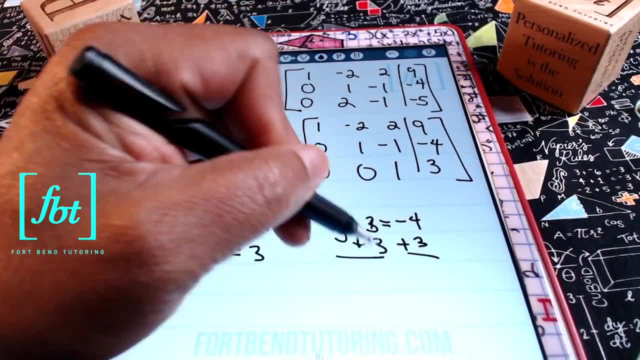 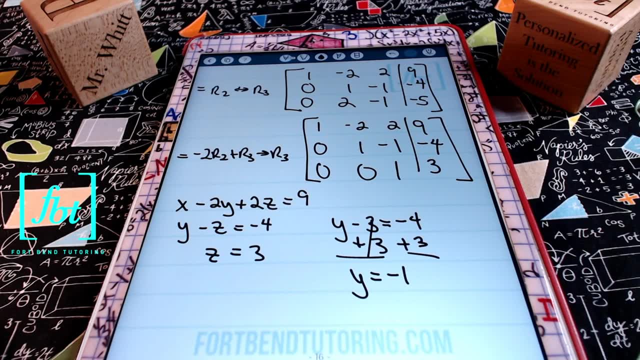 So, in order to solve for y, all you got to do is just add 3 to both sides of the equation. What does that give you? That gives you negative 1, people. So now we have z equals to 3.. We got y equals to negative 1.. 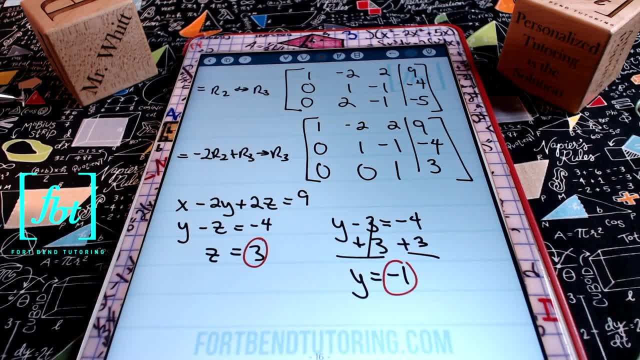 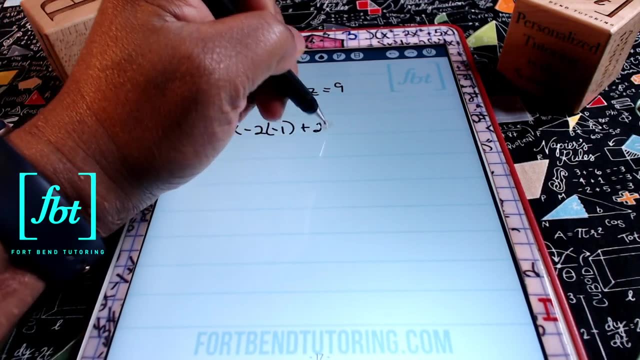 We'll be plugging in these two values into the first equation here. So we'll keep in mind that y equals to negative 1 and z equals to 3 as we plug in those two values into our first equation in our system. So we'll have x minus 2 times negative 1 plus 2 times 3 equals 9.. 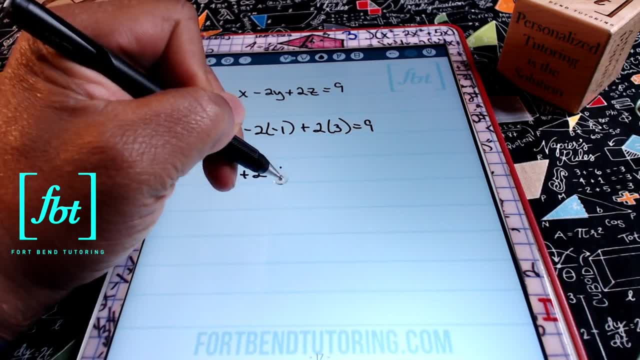 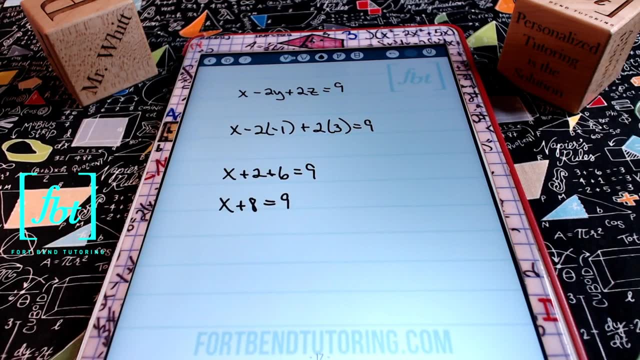 Simplifying, you'll have x plus 2 plus 6 equals to 9.. We know that 2 plus 6 is 8, right, So we'll go ahead and rewrite it as x plus 8 equals 9.. And then, subtracting 8 to both sides, you'll end up with x equals to 1.. 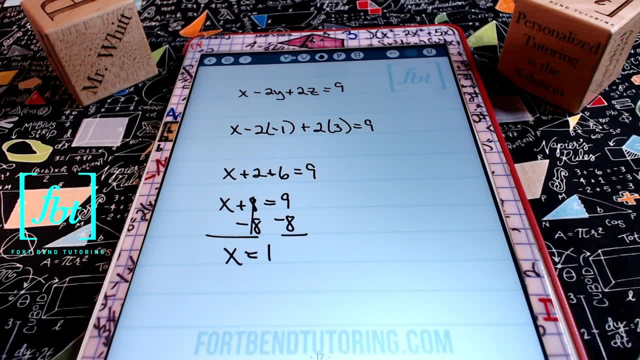 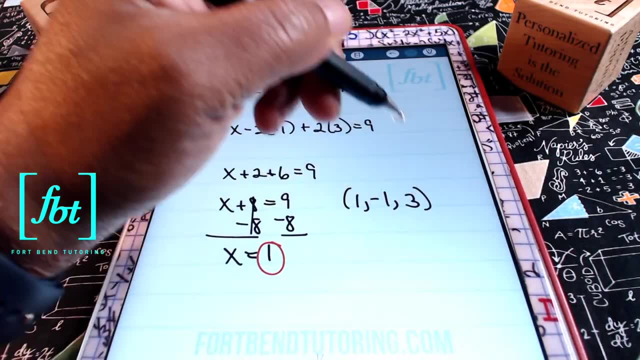 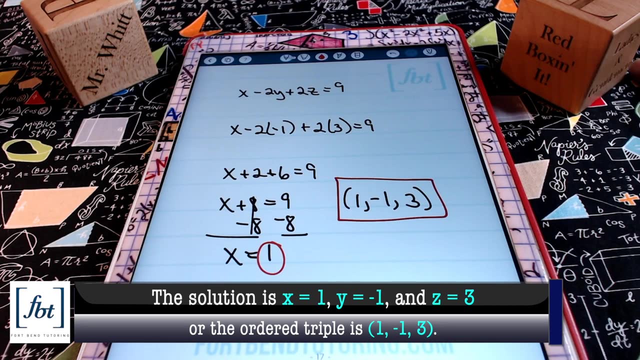 And now you have all three values that you were looking for for your variable. With all the values solved for, we'll have our order triple as 1, negative, 1, and 3.. Red box it people. There you go, and that is your answer for problem number 4.. 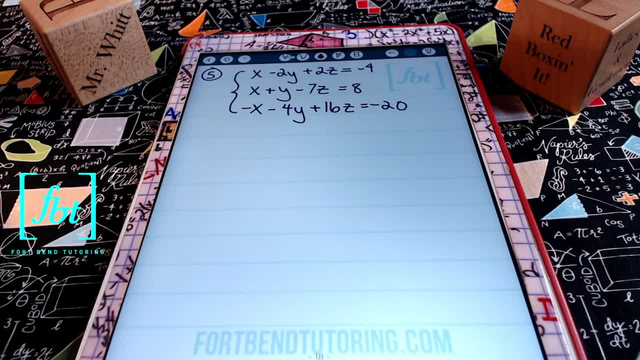 All right, let's check out problem number 5.. In problem number 5, we have once again three equations with three variables. So by now you should start getting familiar with the process. You should know that your first step is to rewrite this system as an augmented matrix. 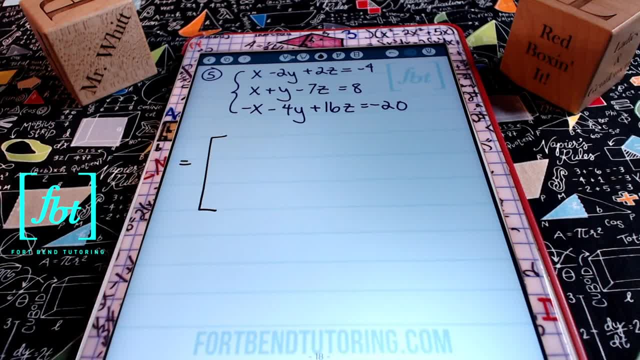 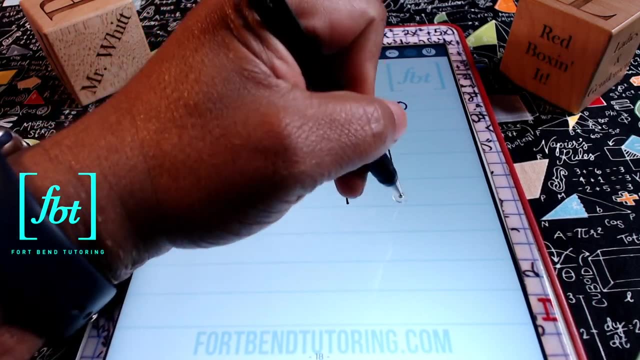 Now I prefer to make videos that have multiple problems in them, guys, so you can start working on the mastery of the concept, not only just to understand what to do, but also how to do it in a consistent manner. So our augmented matrix will be 1, negative 2, 2, negative 4 for the first row. 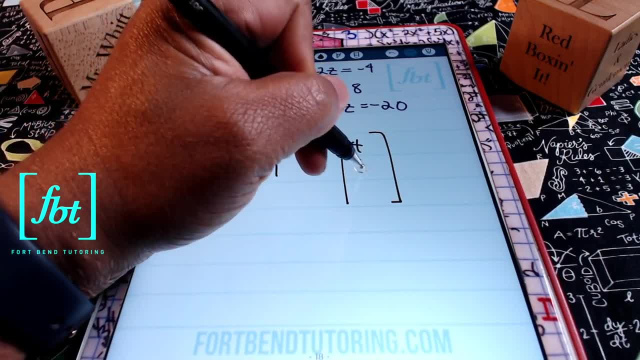 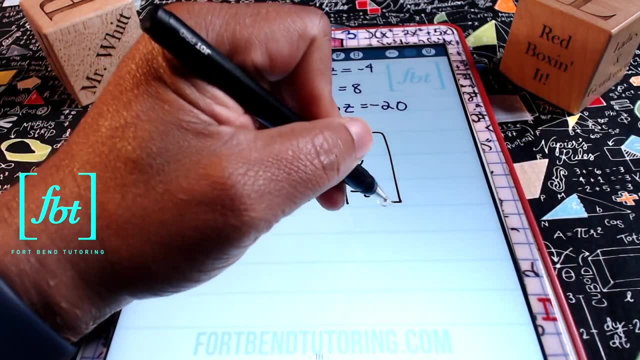 And we'll have 1, 1, negative 7, and 8 for the second row, And finally we have negative 1, negative 4,, 16, and negative 20.. All right, so that completes our augmented matrix. 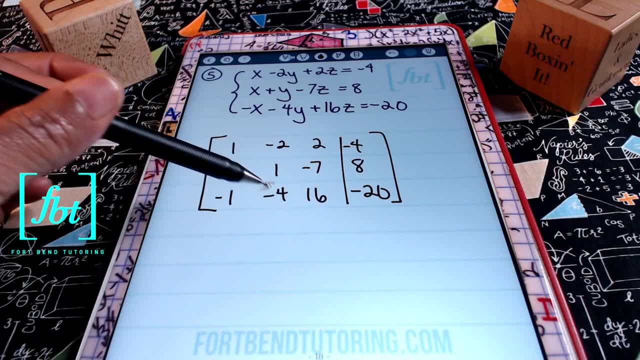 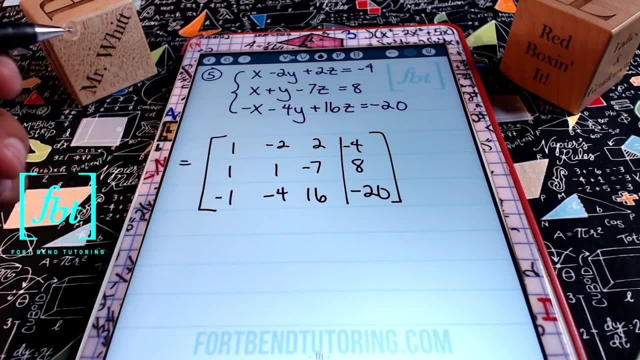 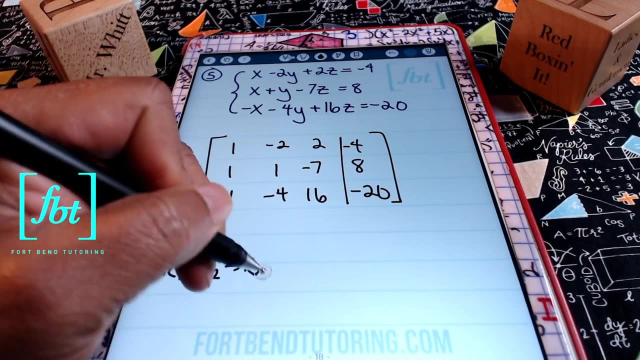 So remember, we want 1s down the main diagonal here, with 0s underneath. So my first focus is to get the 1 in the second row, first column, to become a 0. How do I do that? I'm simply going to say row 1 minus row 2, putting the result in row 2.. 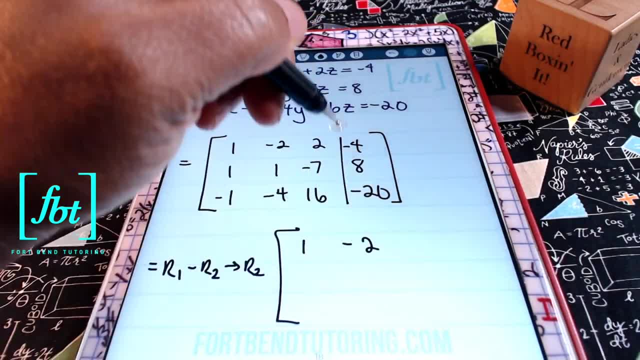 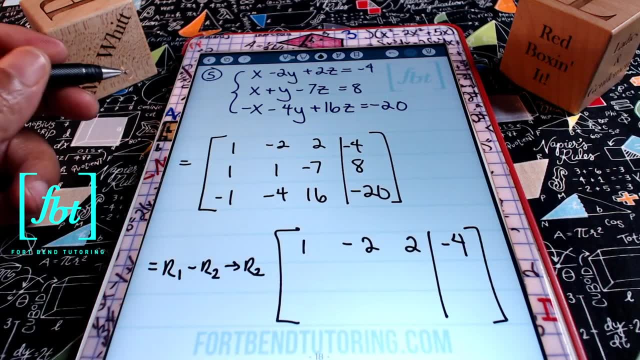 Setting this up. we'll bring down our first row as it is. We have 1, negative 2,, 2, as well as negative 4.. And then you'll bring down the third row, as is Negative 1, negative 4, 16, negative 20.. 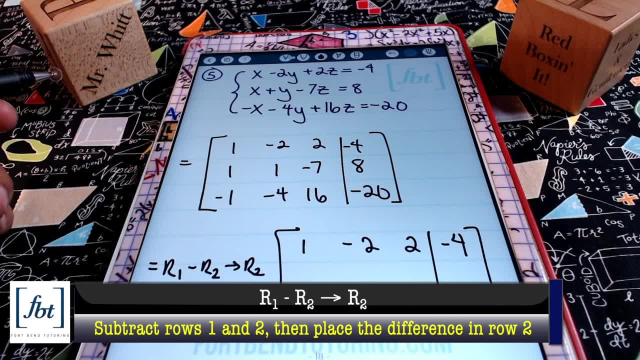 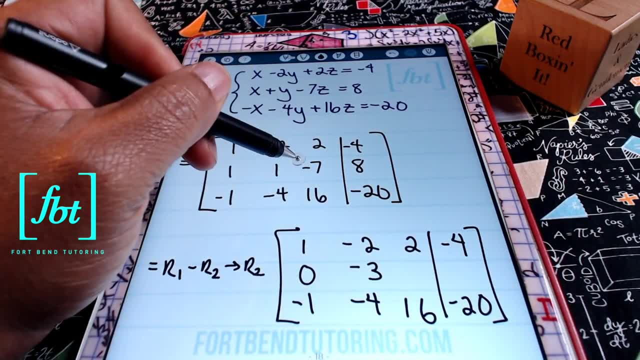 And then, with our second row, we'll be subtracting row 2 from row 1.. So 1 minus 1 gives you 0.. Negative 2 minus 1 gives you negative 3.. 2 minus negative 7 gives you positive 9, guys. 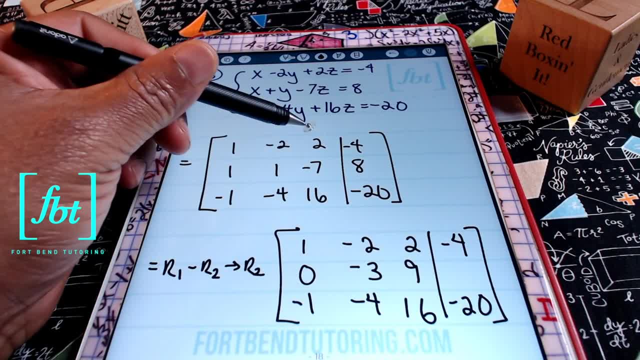 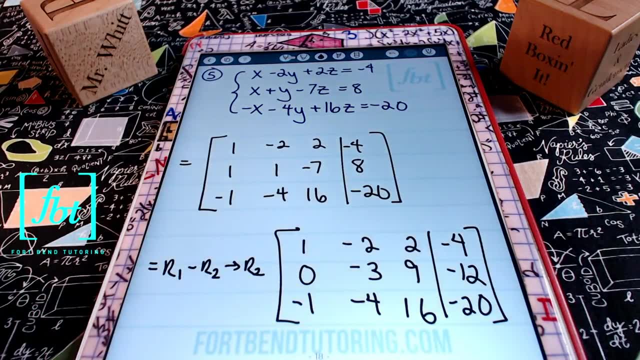 That 2 minus a negative makes it a positive 7. 2 plus 7 is 9. Then you'll have negative 4. Minus 8 gives you negative 12. And this will be our new row equivalent matrix. Okay for our augmented matrix here. 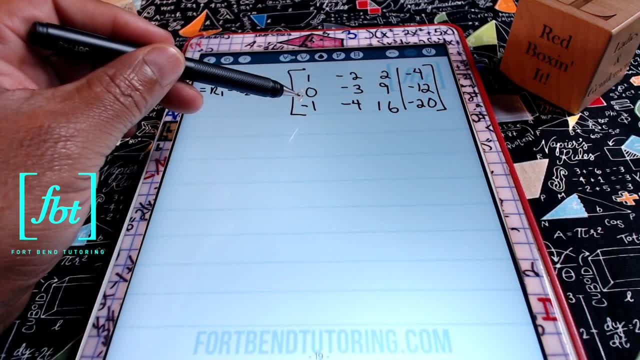 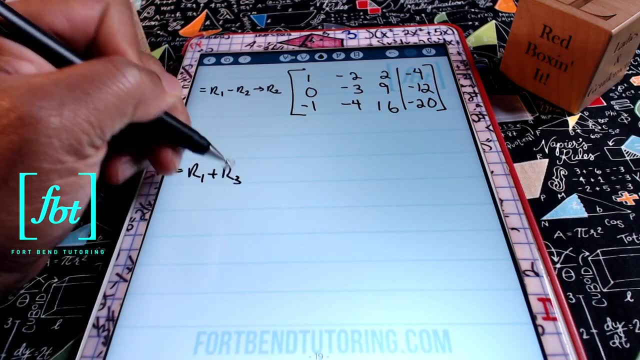 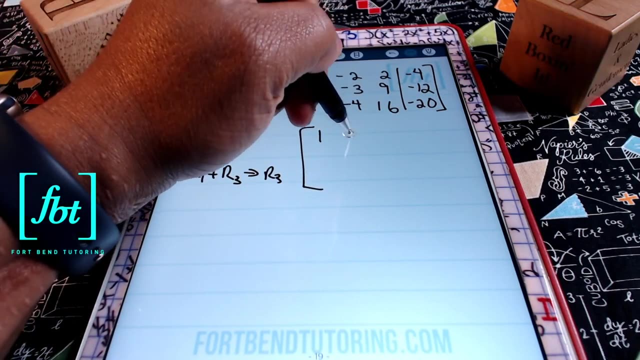 Continuing our process, we'll next want a 0 for the first element in the third row. I can make that happen by adding the first row and the third row together, Putting the result obviously in the third row. So that means I'll be bringing down the first two rows as is. 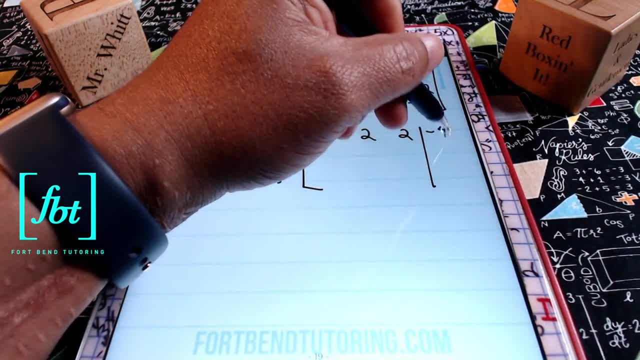 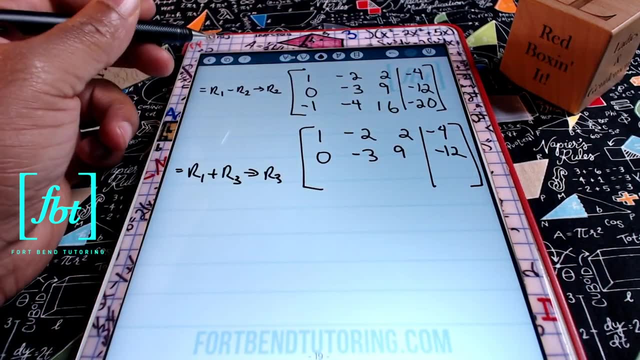 I have 1, negative 2,, 2, and negative 4.. And I also have 0, negative 3,, 9, and negative 12,, as well as 1 plus negative. 1 gives me 0.. Negative 2 plus negative 4 gives me negative 6.. 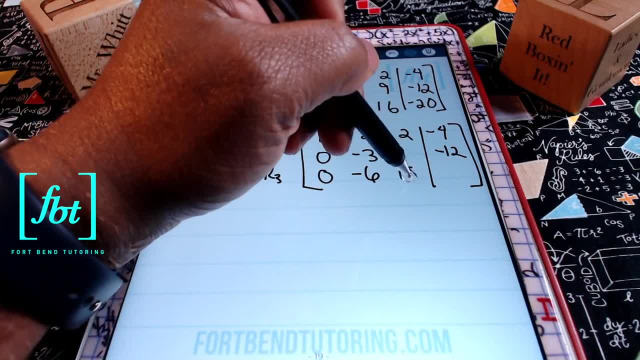 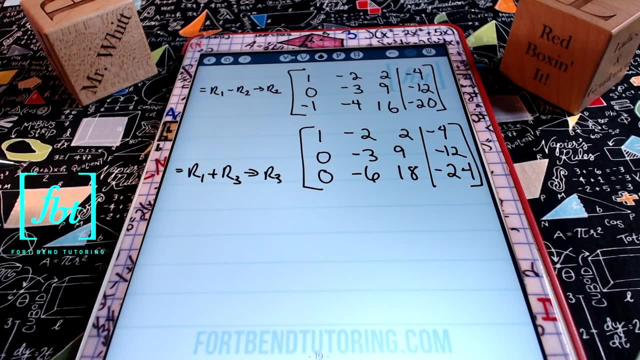 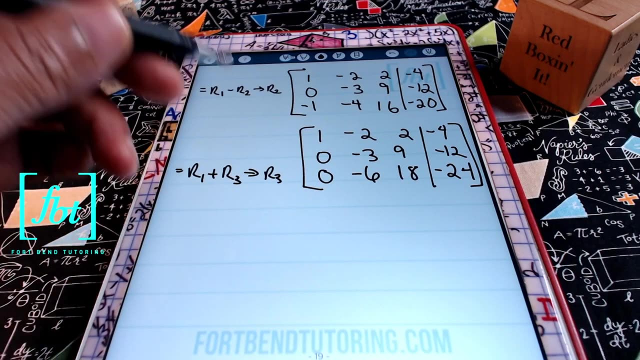 2 plus 16 gives me 18.. And then negative 4 and negative 20 combined to give me negative 24.. And this is my new third row after that row operation. Now, next, we'll want to get a 1 down this main diagonal where the negative 3 is. 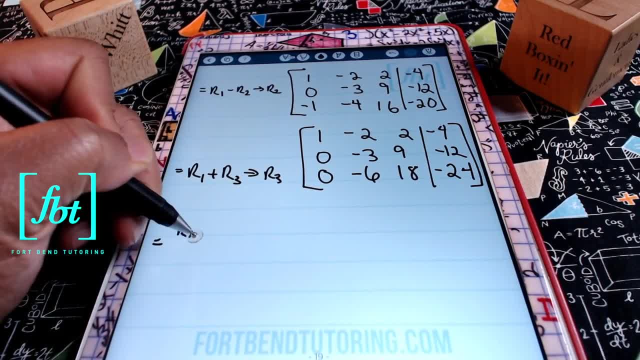 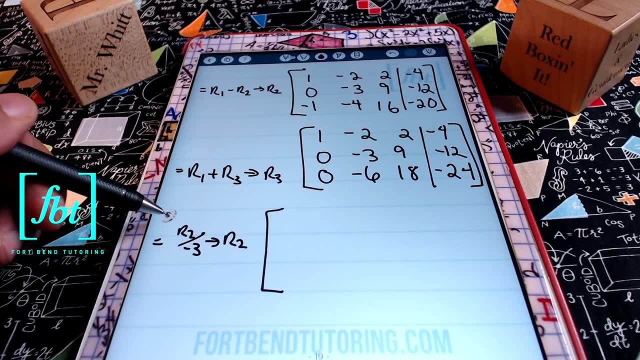 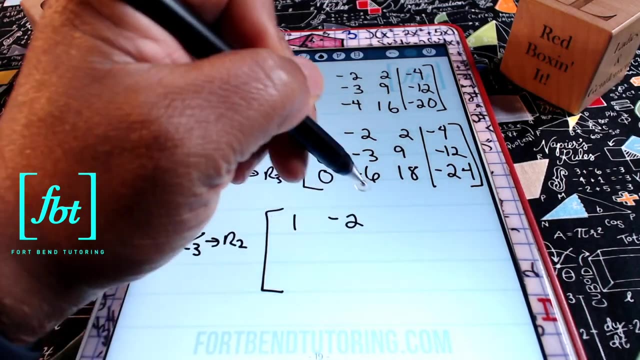 We can easily do that by dividing row 2 by negative 3.. Putting the result in row 2.. So once again, we're going to be dividing row 2 by negative 3 and then putting that result in row 2.. So that means that the first row will remain the same. 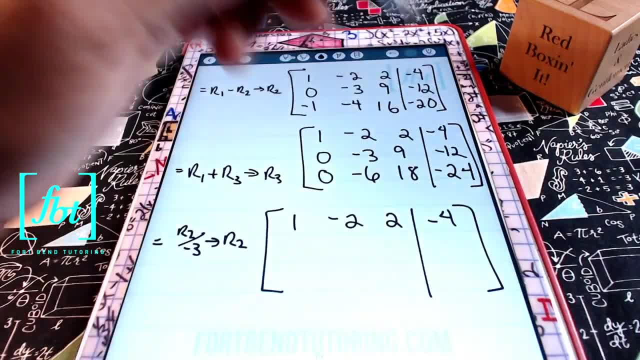 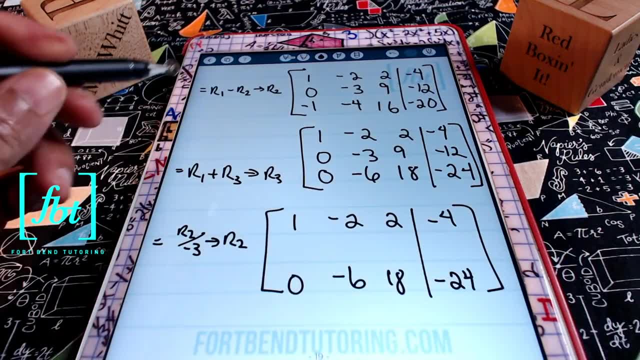 I have 1, negative 2,, 2, as well as negative 4 for that first row. The third row is 0, negative 6, 8.. So I have 18 and negative 24.. And then finally, dividing each of the elements in the second row, I'll have 0 divided by negative, 3 is 0.. 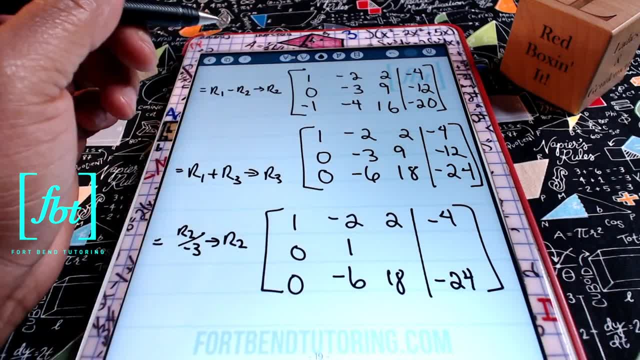 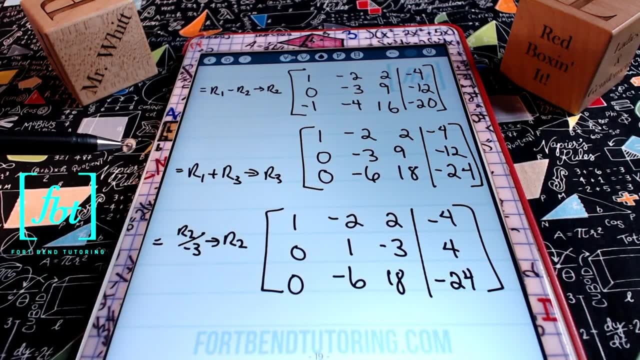 Negative 3 divided by negative 3 is 1.. 9 divided by negative 3 is negative 3.. And negative 12 divided by negative 3 is positive 4.. And this is going to be our row equivalent matrix after that row operation. 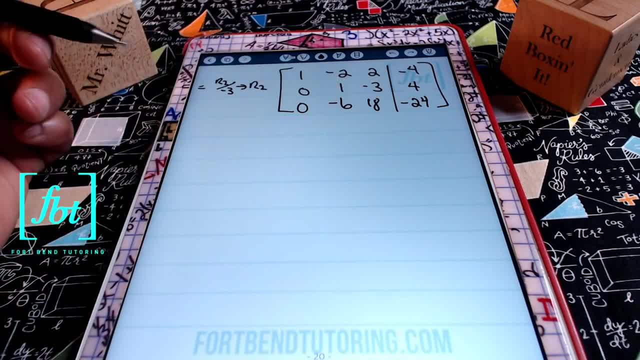 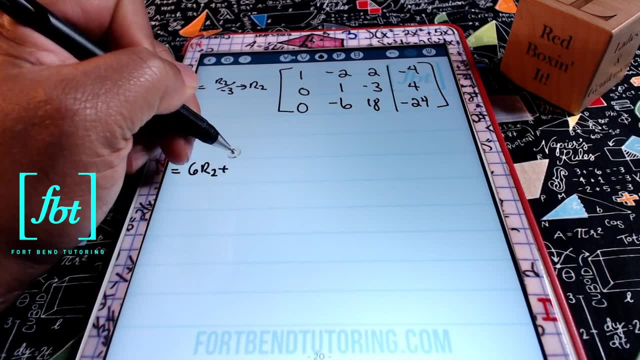 Our next step is to create a 0 where the negative 6 is. We can do that by going ahead and multiplying row 2 by 6.. So if I say 6 times row 2 and then add that to row 3, putting the result in row 3,. 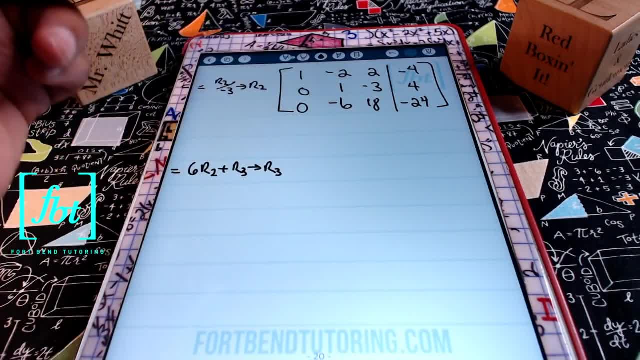 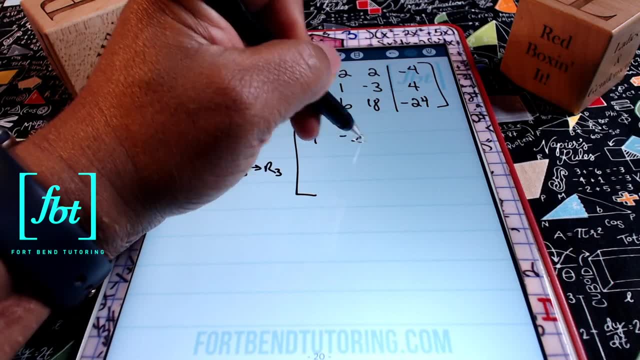 we should get the 0 where that negative 6 element is currently lying. So let's go ahead and check that out. We'll be bringing down the first two rows as is, So I have 1,, negative 2,, 2, as well as negative 4.. 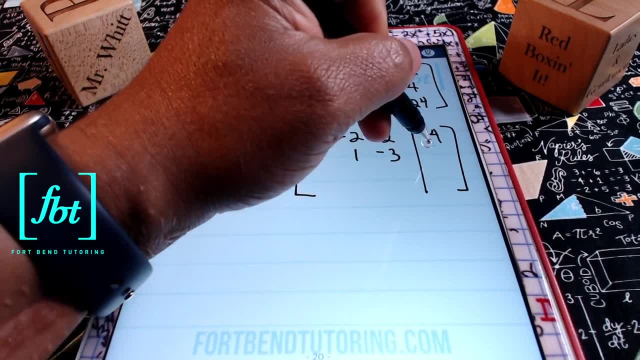 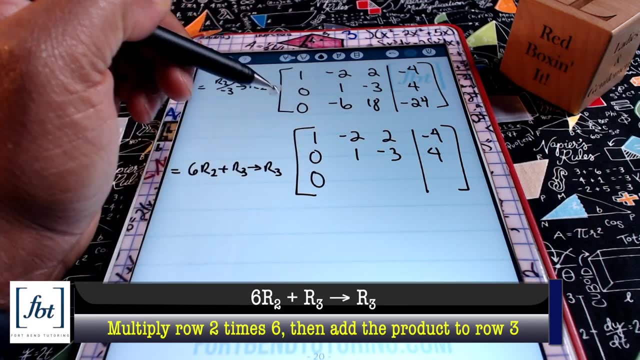 The second row is 0,, 1, negative 3, and 4.. And then, finally, to get our third row we're going to have: 6 times 0 is 0, 0 plus 0 gives us 0.. 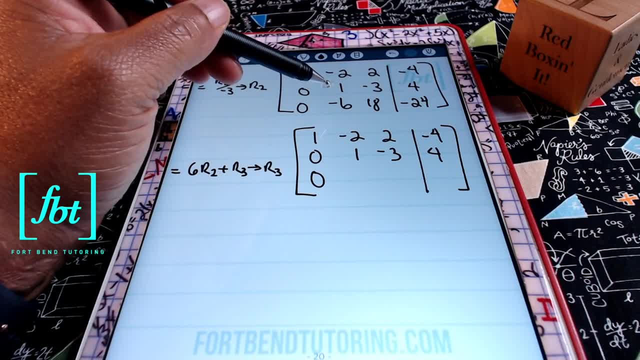 Then 6 times 1 is 6, and 6 and negative 6 combined to give us 0.. Well, that's good. That's what we wanted. Multiplying 6 times negative 3,, you get negative 18.. 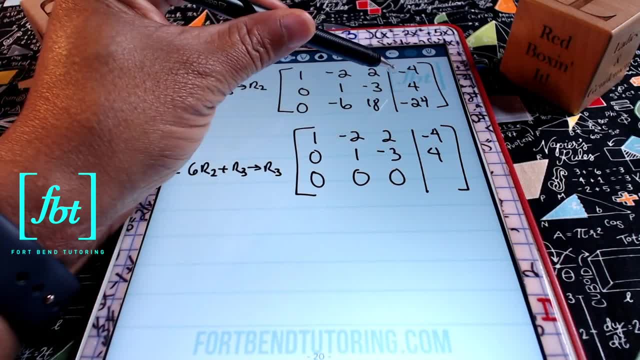 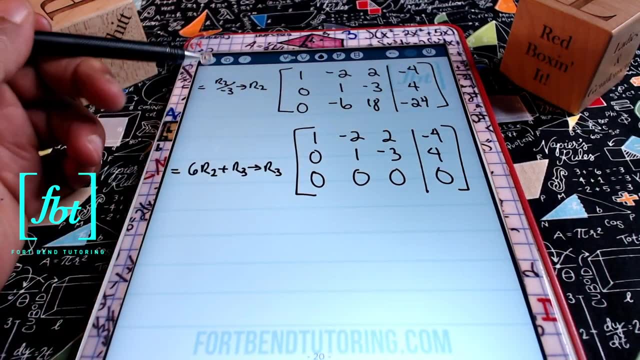 Negative, 18 plus 18 is 0.. And then, multiplying 6 times 4,, you get 24, and 24 plus negative 24 is 0.. Ladies and gentlemen, any time you get a row or an equation where all the coefficients 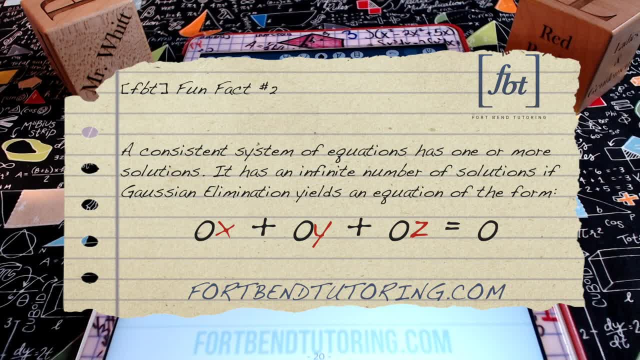 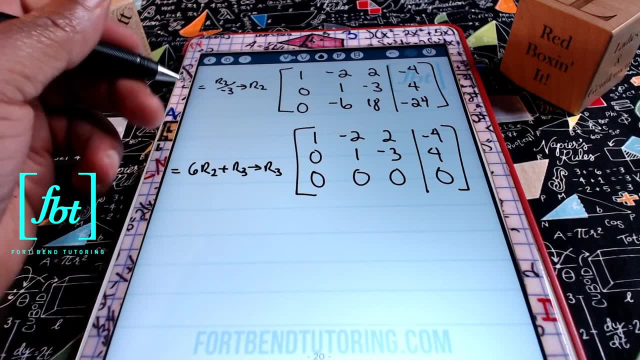 are 0,. you will end up with a consistent system that has an infinite number of solutions. All right, So what you want to do now is you want to go ahead and back. substitute your equation at this point, and you're going to find that you have x minus 2y plus 2z equals. 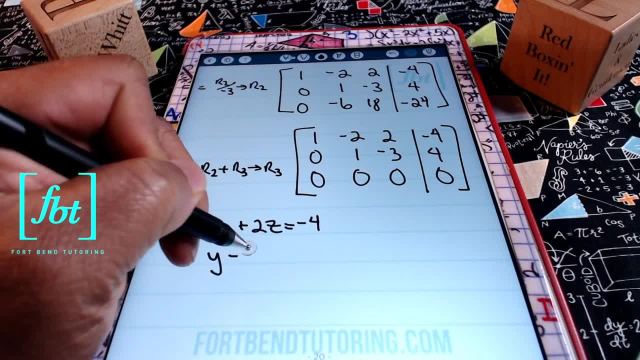 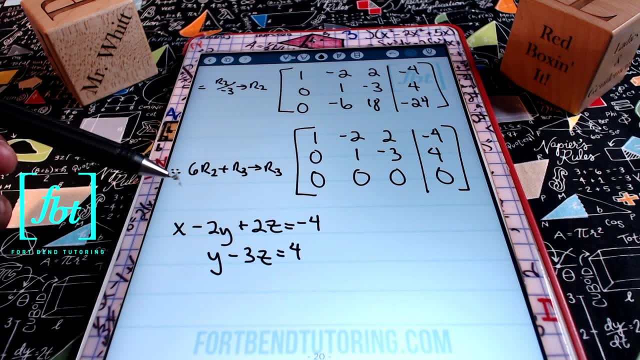 negative 4, while you also have y minus 3z equals to 4.. So what we'll realize is that we still have three unknowns, But because we have a lack of a third, unique equation to find out all three variables is you'll want to write your result. 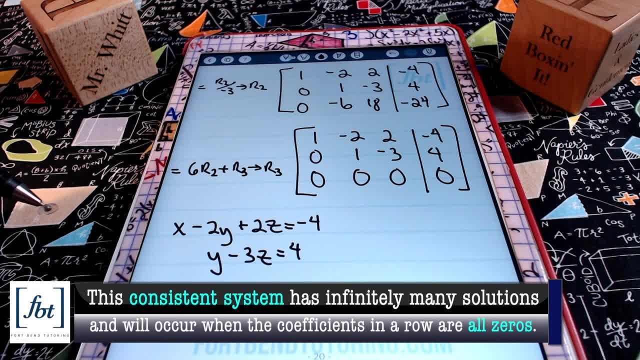 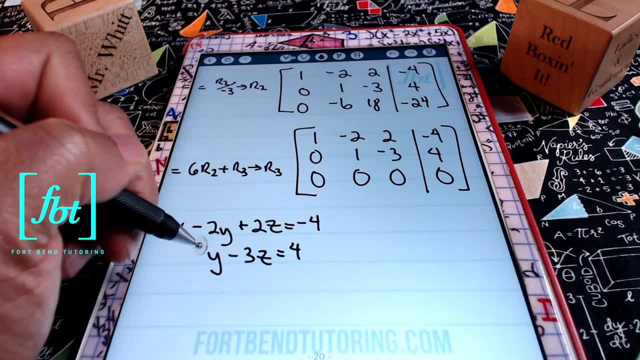 reflecting the fact that one of these values can be any number. So what we're going to do is we're going to end up rewriting each of these equations in terms of z. For instance, to solve for y, all I have to do is add 3z to both sides of the equation. 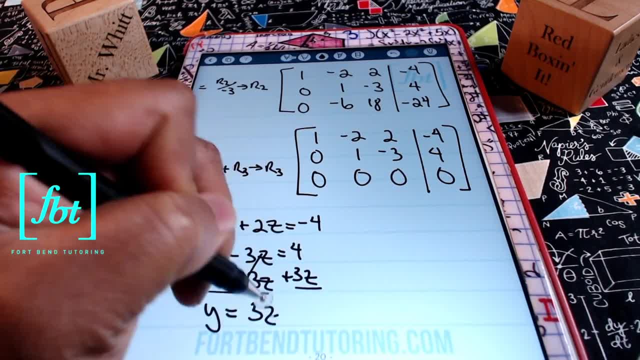 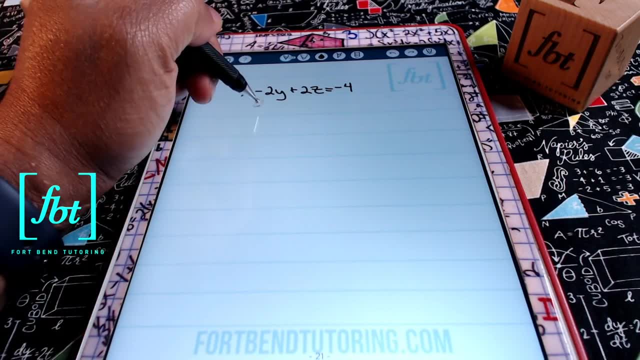 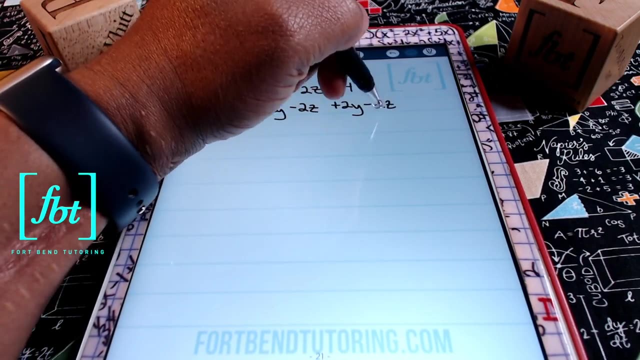 Doing so lets me know that y equals to 3z plus 4.. I'm going to hold on to this value and then solve for x. In solving for x, I'll be adding 2y to both sides of the equation, as well as subtracting 2z to both sides of the equation. 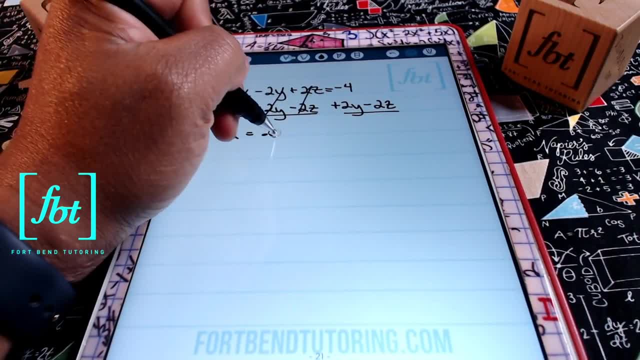 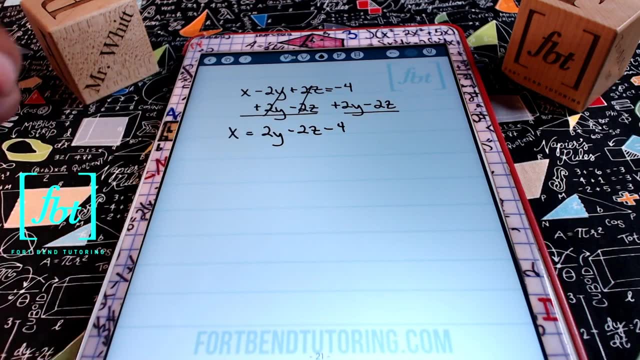 In doing this, I'll have x equals 2y minus 2z minus 4.. However, I'm not done yet, because I know what y is. Remember we said that in the previous step that y was equal to 3z plus 4.. 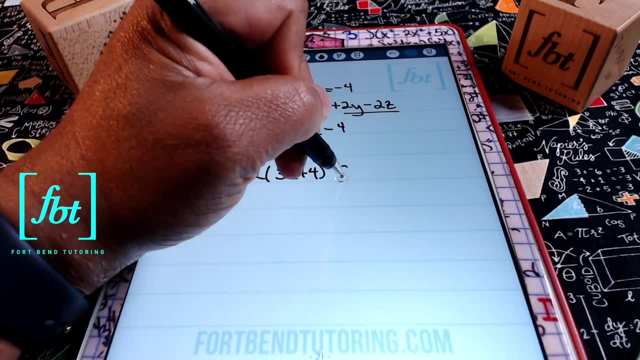 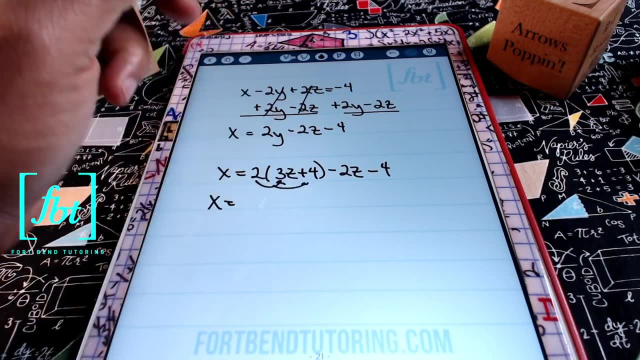 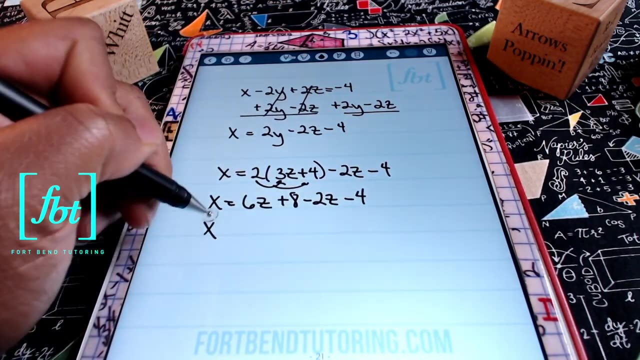 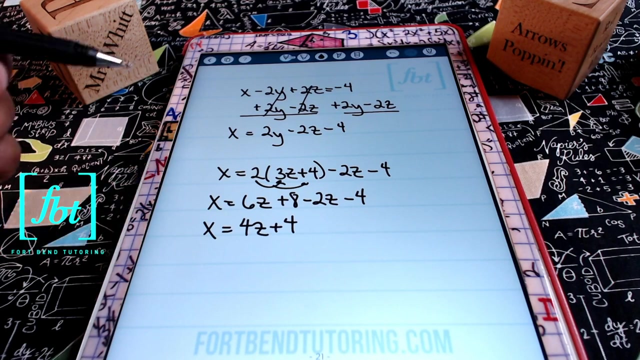 So go ahead and plug that in for your y term simplifying, and I'm going to get my arrows popping. You'll have 6z plus 8 minus 2z minus 4.. This all simplifies to give you 4z plus 4 as your result for x guys. 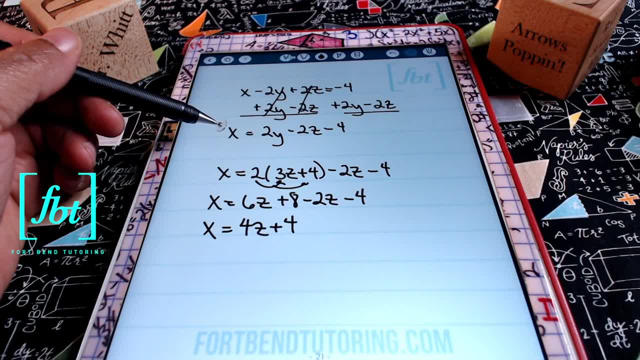 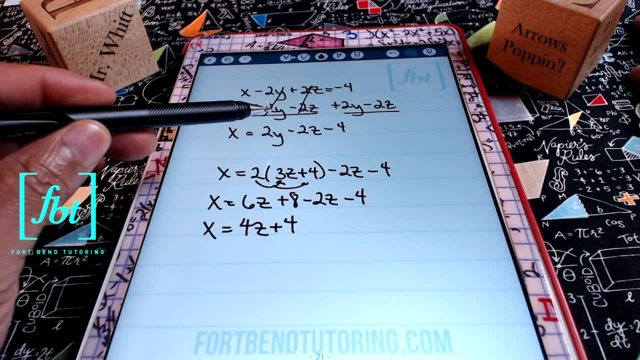 So remember, not only did we isolate the variable x and write our result initially in terms of y and z, because we had determined that all of our solutions were going to be written in terms of z, We then substituted in the value of y that we yielded in our previous step. 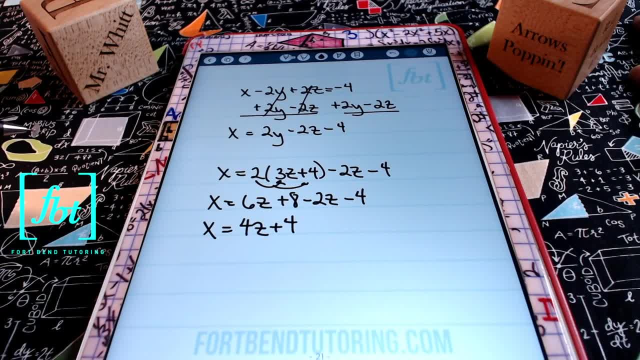 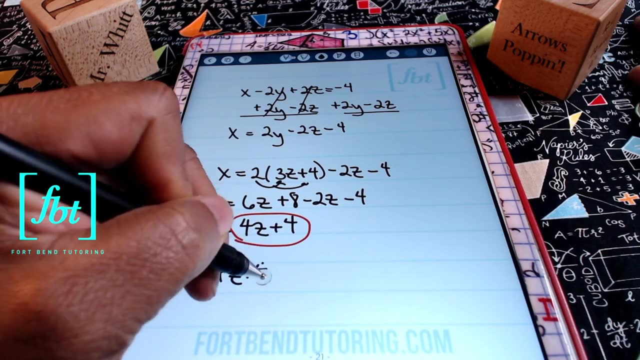 and plugged in that 3z plus 4 in for the variable y. After we distributed and got our arrows popping, we went ahead and combined our light terms and got x equals to 4z plus 4.. With these three values found, now we'll have our answer as 4z plus 4, 3z plus 4z. 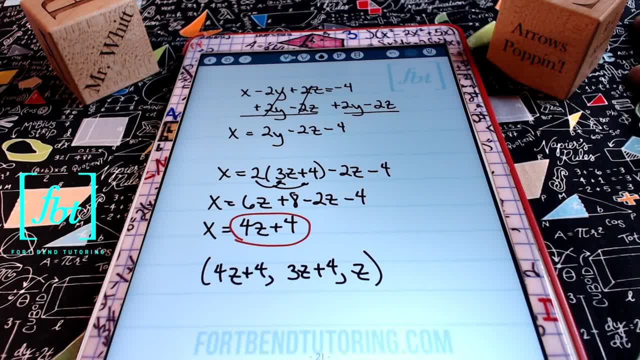 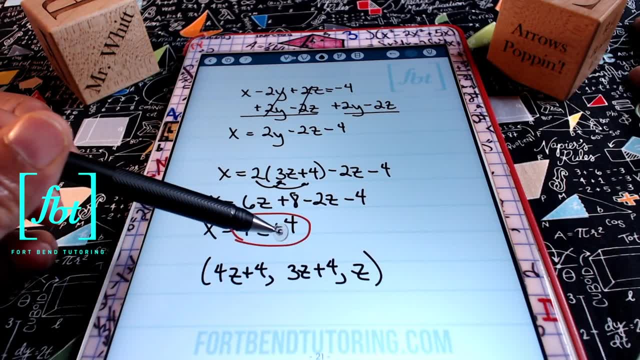 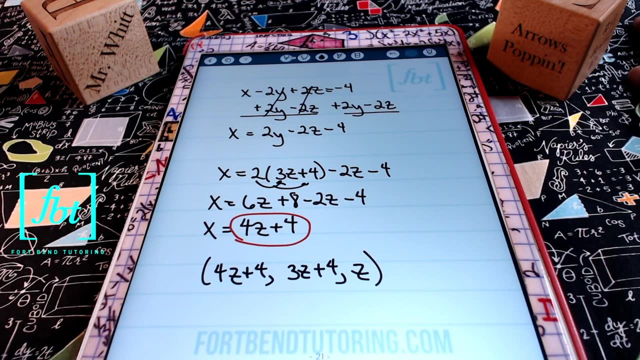 And what this shows is a relationship between the infinite number of solutions- that as long as your x value is 4 times your z value plus 4, and as long as your y value is 3 times your z value plus 4, you will end up with a solution to the original system of equations. 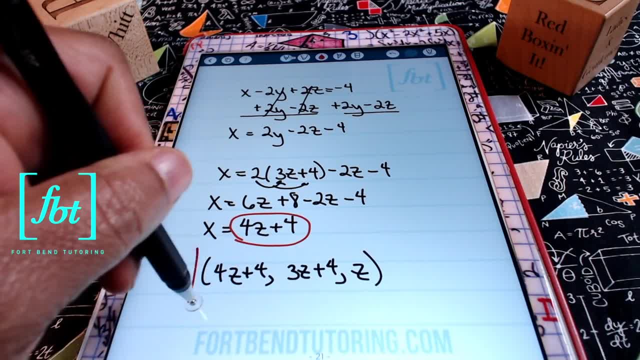 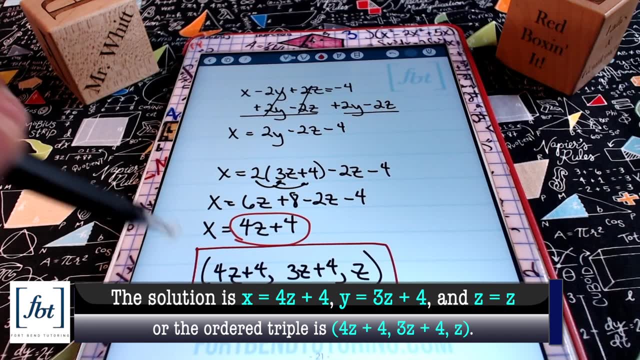 Done and done, Red box it. And that is our answer here for problem number five. So in this problem we had an infinite number of solutions, and that's the way you write it, people. All right, Let's move on to our next example. 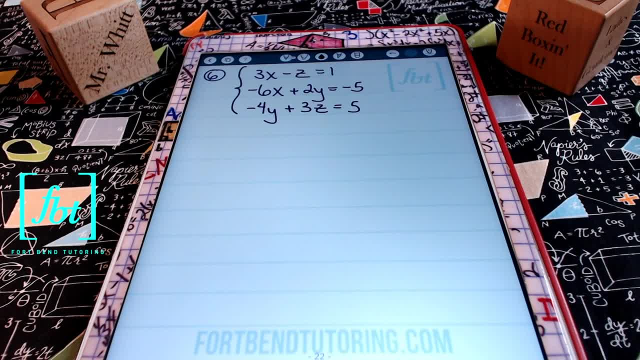 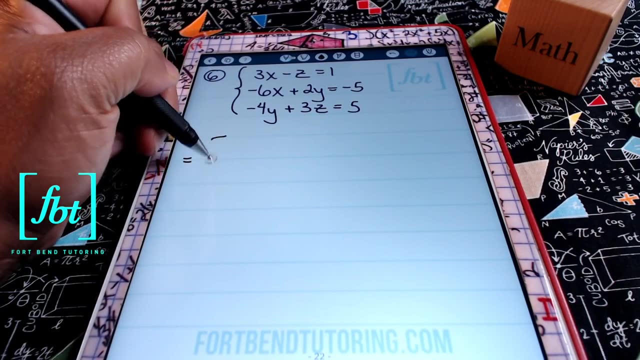 In example six, we once again have three variables in a system of equations here. So we're given three equations. That's a good start, And our first step remains to write our augmented matrix first. So here, writing our augmented matrix, you're going to end up with the following: 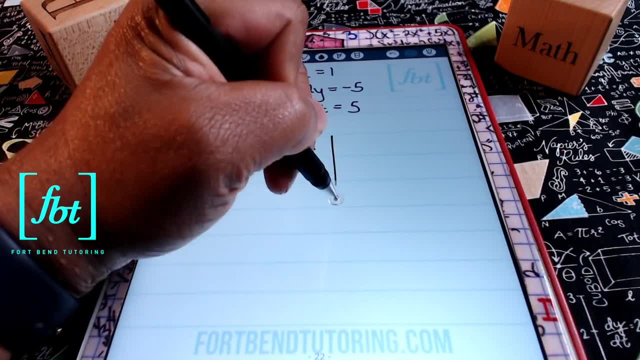 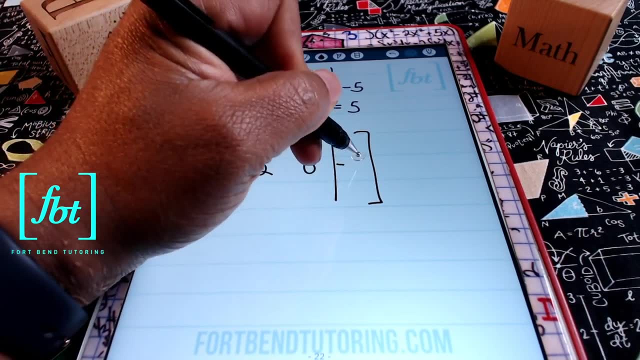 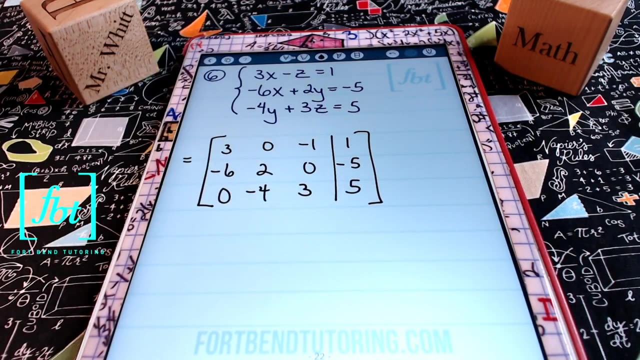 You'll have three zero negative one and one. With your second row, you're going to have negative six, two zero negative five. You'll then have zero negative four, three and positive five, And this is your augmented matrix for problem number six. 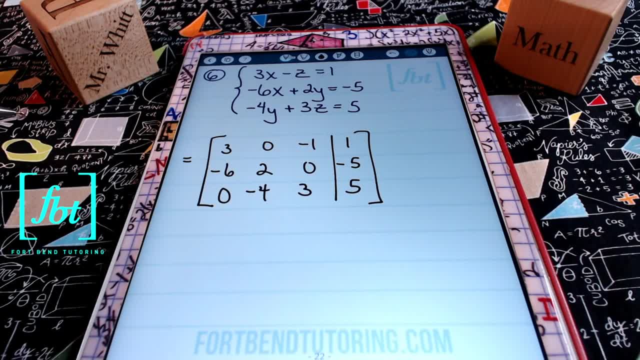 With this problem. I'm sniffing a little drama on the way, So what I'm going to do is I'm going to take advantage of the fact that I know that I'm going to want the second row, first column element to be a zero. 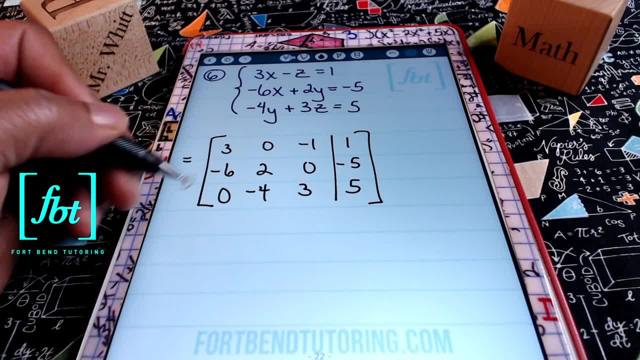 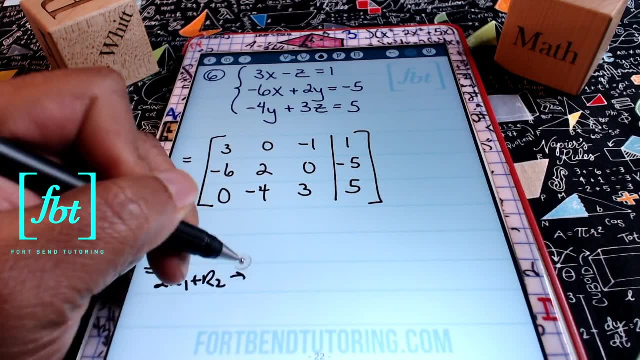 I'm gonna take advantage of the fact that negative six is a multiple of three, So let's go ahead and take care of that first. I'm going to have two times row one plus row two, writing the result in row two. Let's do that, guys. 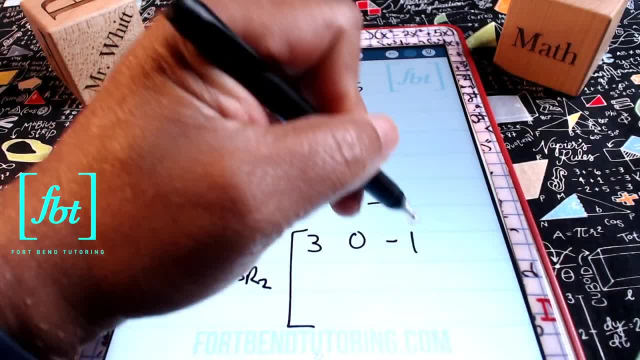 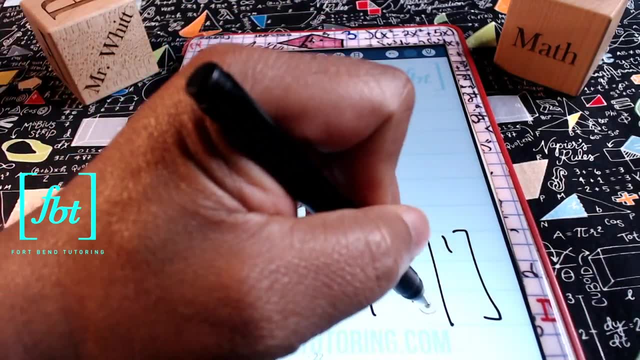 That means that the first row will remain the same, All right, and then the last row remains the same. So we have zero negative four, three and five, And then finally, in order to get the new second row, I'll be multiplying two times. 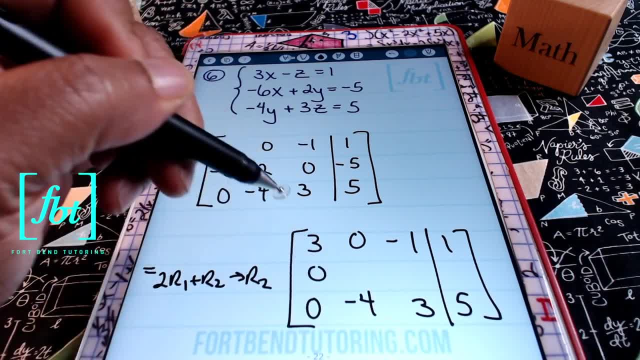 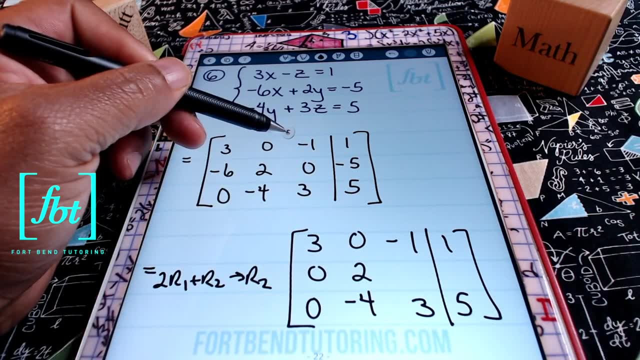 three to get six and six and negative six combined to give me zero. Then I'll be multiplying two times zero to give me zero, and zero plus two is two. I'll also have two times negative. one is negative, two Negative. two plus zero is negative two. 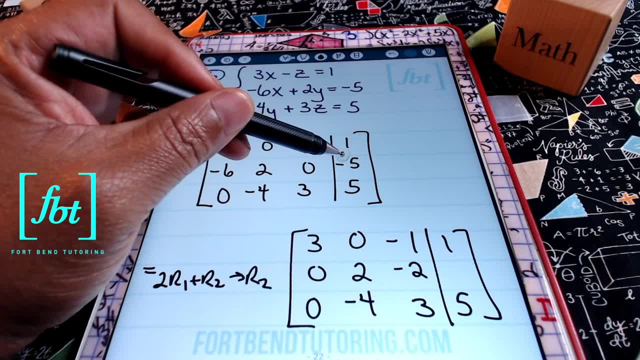 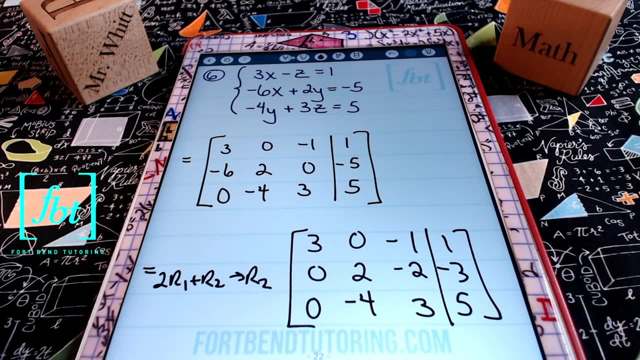 And then I'll have two times: one is two and then two, and negative five give me negative three. So this is going to be what I end up with after that first row operation. The next thing I want to do is I want to take advantage of the fact that negative four is a multiple of two. 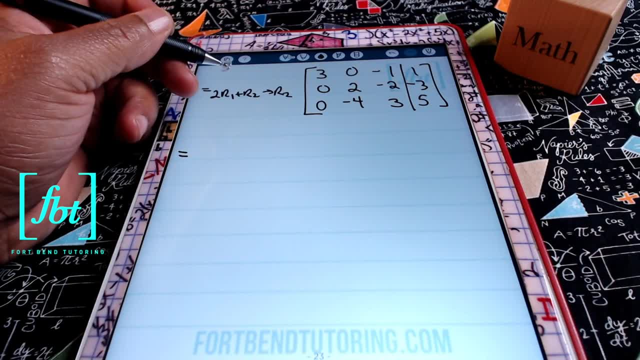 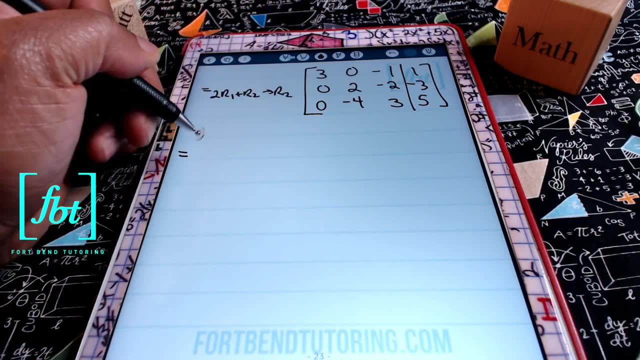 So, just trying to ease this problem, I'm going to take advantage of this process because, like I said, I was smelling drama on the way, so I'm going to try to take advantage of some of these opportunities as I come across them. 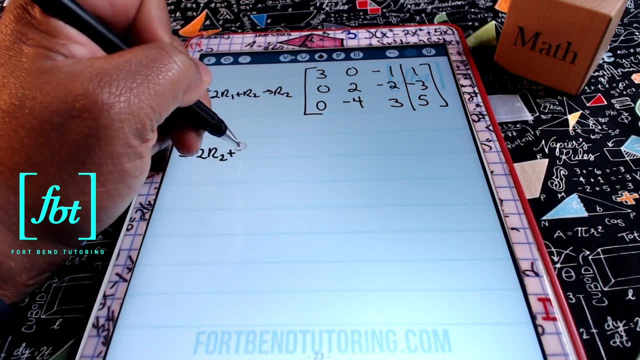 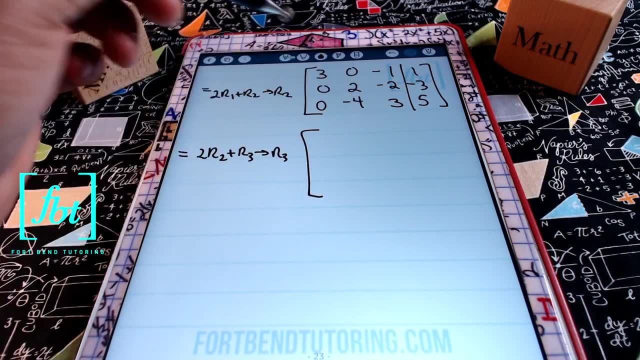 So what I'm going to do with my next one is I'm going to say two times row two plus row three, putting the result in row three. All right guys, this is going to be able to give me a zero down here. 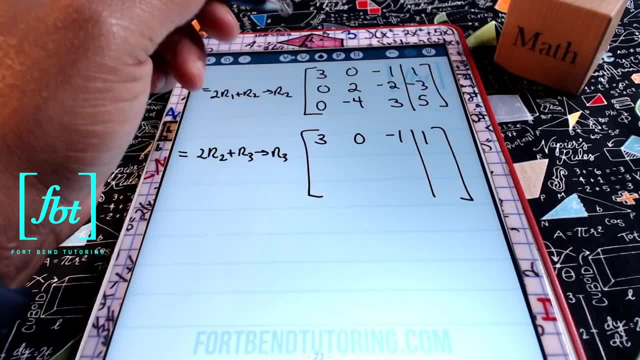 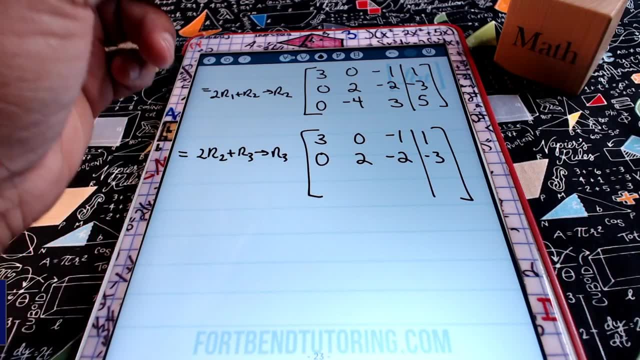 So I'll have three zero negative one and one, as well as zero, two negative, three Negative two negative three, as well as. with this third row, you'll be multiplying two times zero plus zero to give me zero. 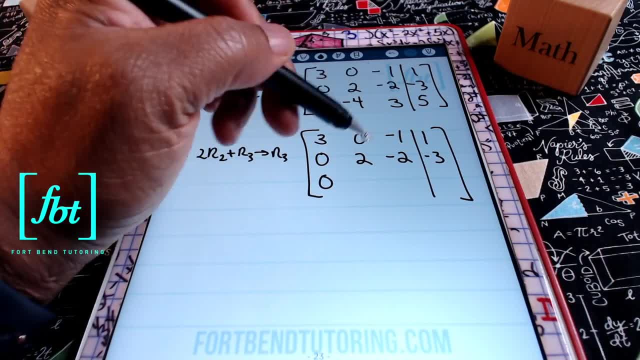 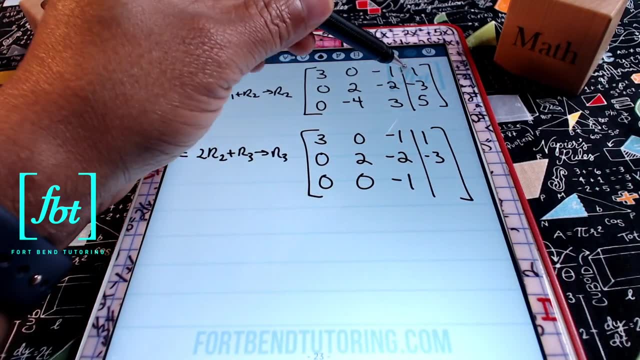 Then two times two is four. four and negative four give me zero. Then two times negative. two is negative four. Negative four plus three gives me negative one And finally we'll have two times negative. three is negative six. Negative. six plus five gives me negative one. 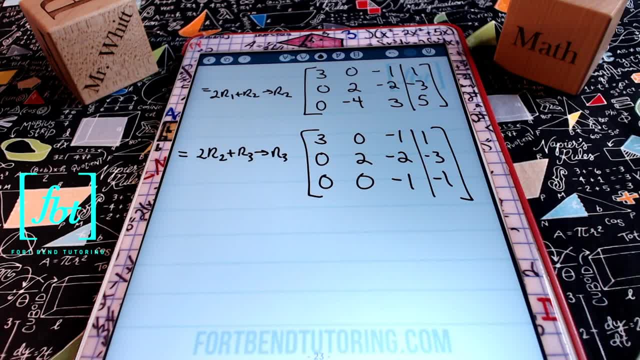 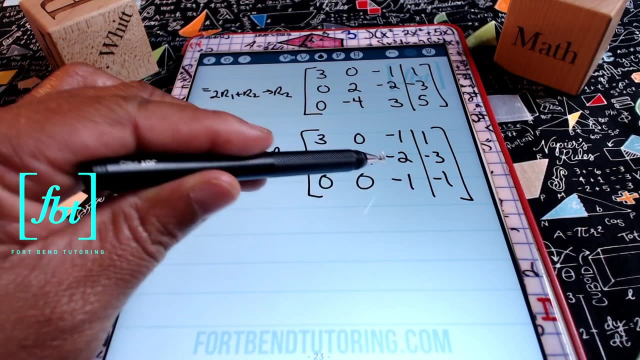 And this is what we have thus far, guys. OK, Now, technically we have a triangular form here. We could just back substitute at this point and solve the system. However, this is not row echelon form. Row echelon form demands that this main diagonal has ones as the coefficients there. 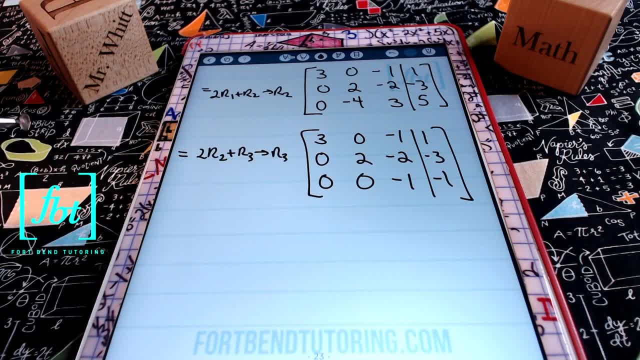 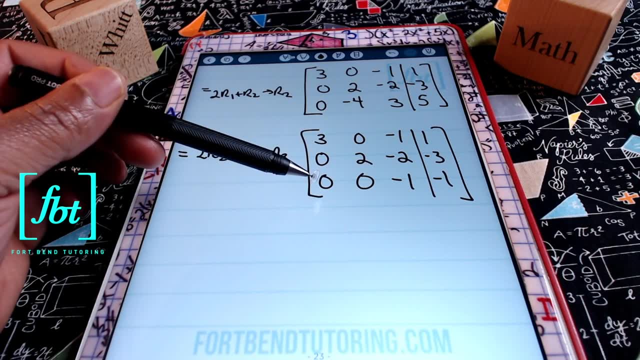 All right? Currently it is not So. that means, in order to make this the case, we'll need to divide everything in row one by three. You'll need to divide everything in row two by two. You'll need to divide everything in row three by negative one. 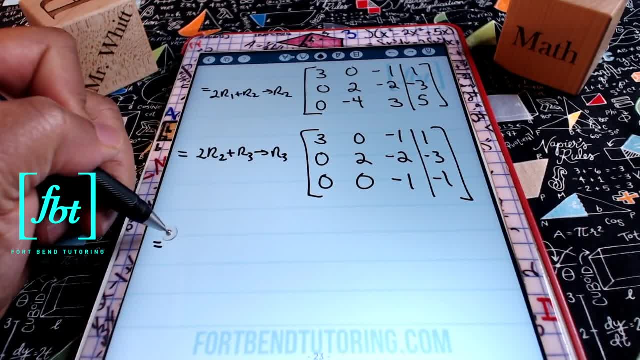 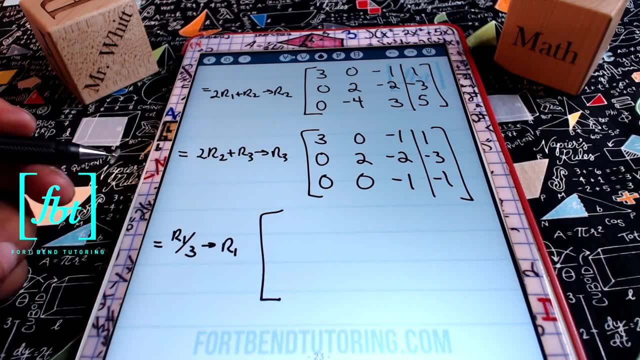 And that's what we'll do. So in our next step, I'm going to have row one divided by three, placing the result in row one. Let's check it out, guys. First I bring down my other two rows, as those will be unchanged. 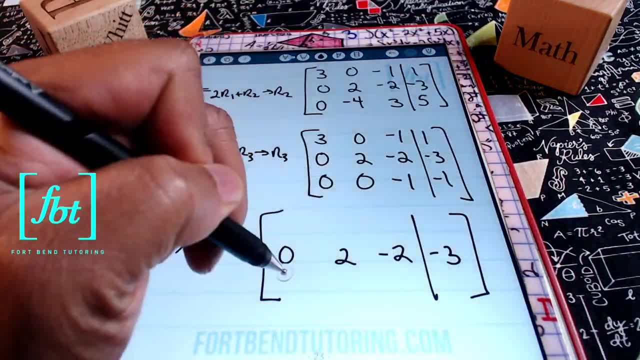 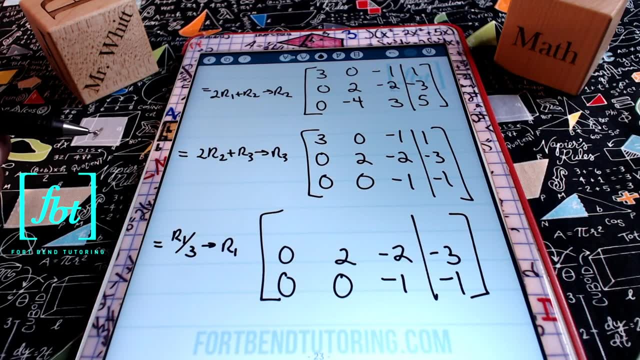 All right, And this just calms me in my process- guys, just bringing down the rows that I don't have to mess with. OK, so now I can put all my focus in the row that does need to change And we'll be going through each of the elements in row one, dividing by three. 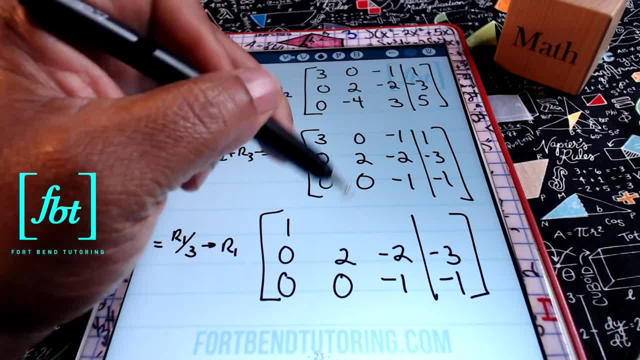 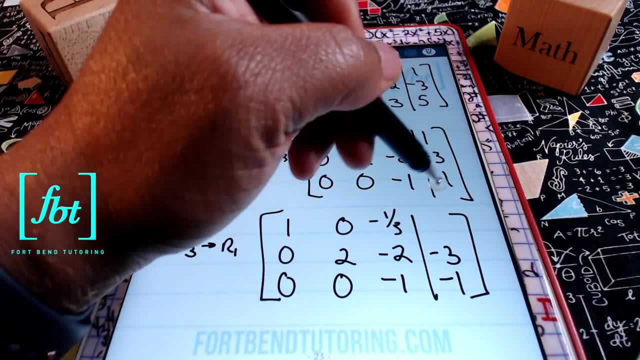 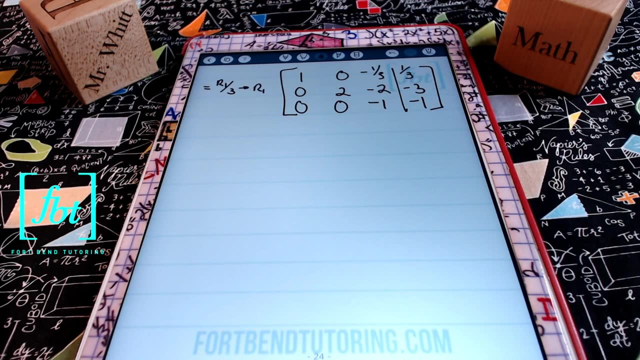 Three divided by three is one Zero. divided by three is zero Negative. one divided by three is negative one third. And one divided by three is one third. just like that, For our next step, we're going to be dividing each of the terms in row two by two. 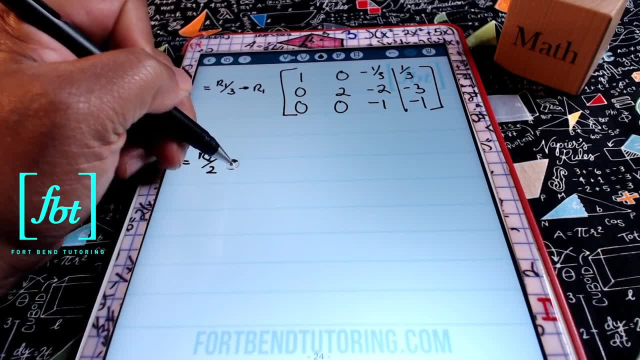 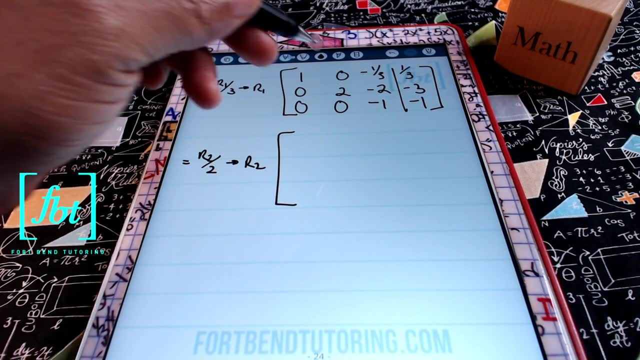 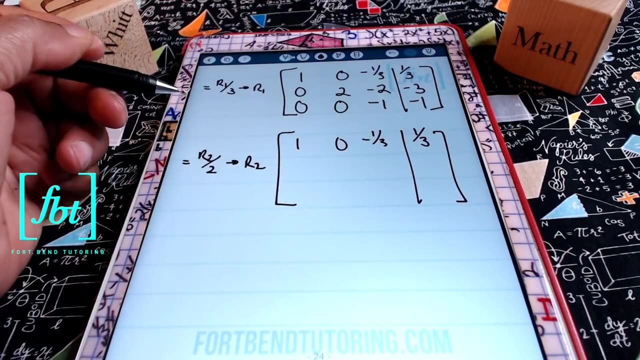 So we'll have row two divided by two, placing the result in row two. That means that row one and row three will go unchanged. for this operation, I'll be bringing down one zero negative, one third and one third, And then the third row will have zero, zero, negative, one negative one. 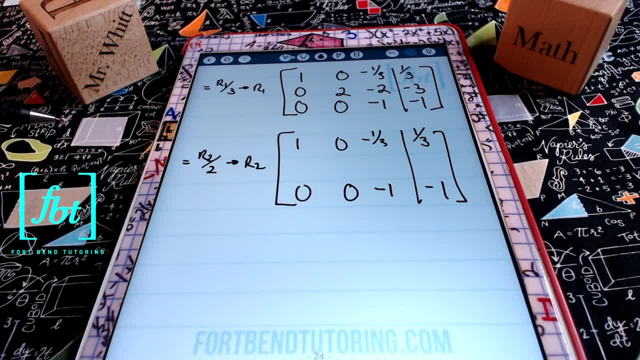 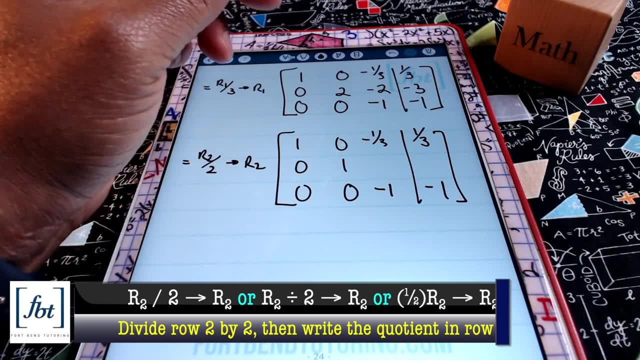 For your second row. go ahead and divide each of the elements in row two by two. Zero divided by two is zero. Two divided by two is one Negative. two divided by two is negative one And negative. three divided by two gives you negative three halves. 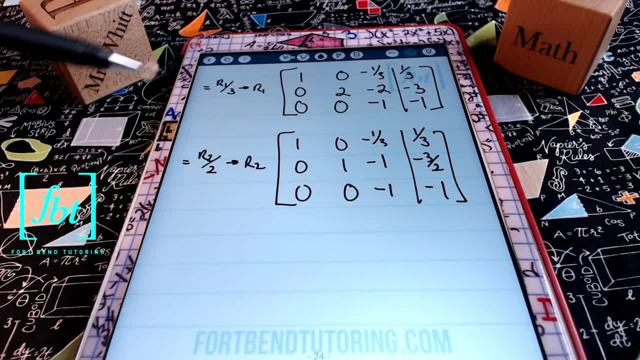 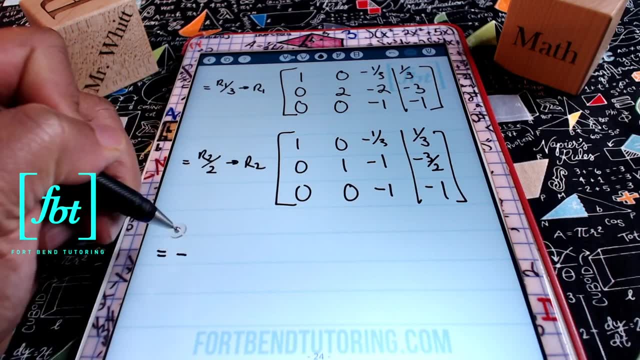 So in our next step, in order to put the matrix in row echelon form, we'll need to multiply or divide row three by negative one. So I think I'm going to do something different. I'm going to say negative one times row three, putting the result in row three. 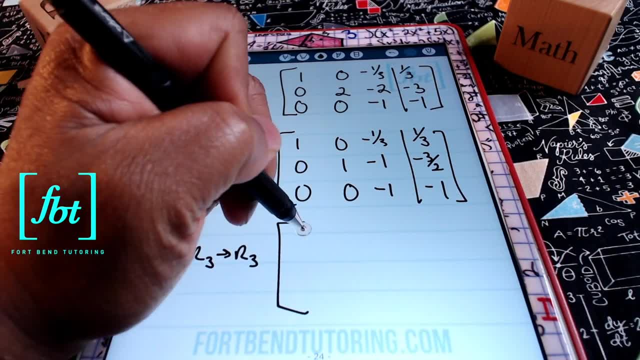 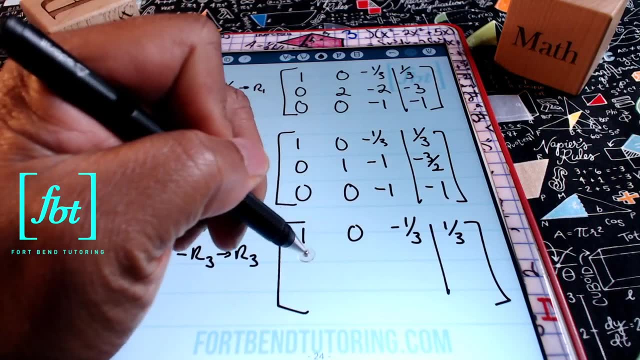 Obviously, the first two rows go unchanged. Let's bring those down. We'll have one zero, negative, one third and one third here, as well as bringing down zero, one negative one and negative three halves. And finally, for our third row, 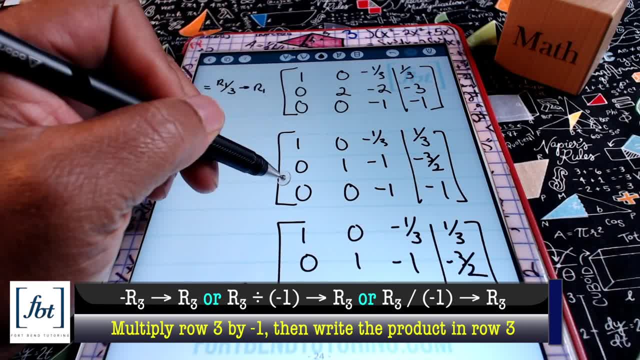 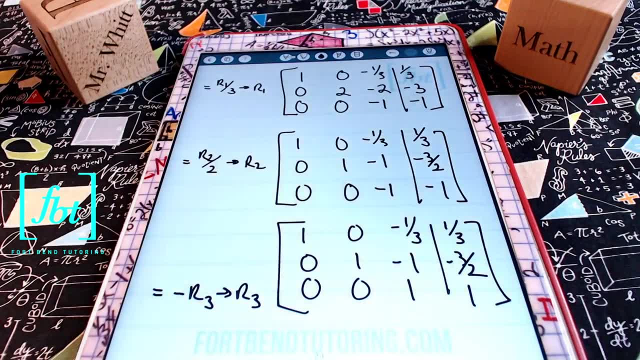 we're going to go ahead and change all the signs. So the opposite of zero is zero, The opposite of zero is zero, The opposite of negative one is positive one And the opposite of negative one is positive one. And now we have row echelon form for our augmented matrix here. 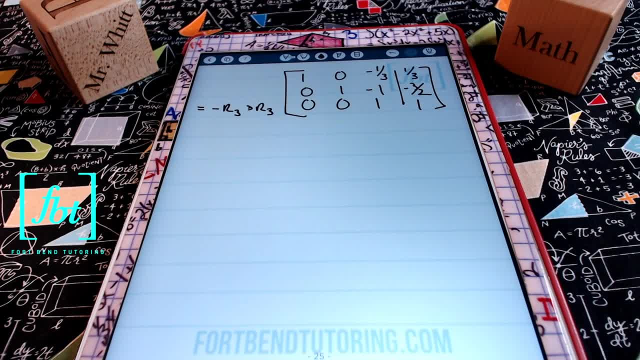 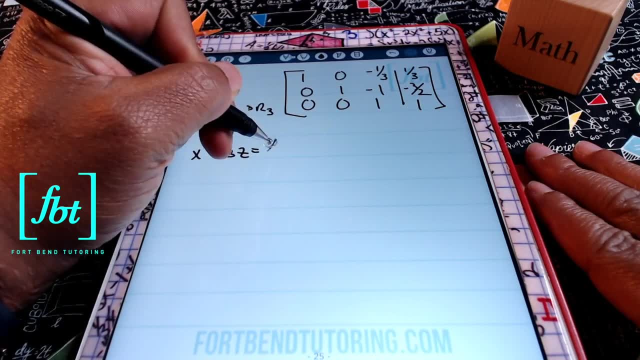 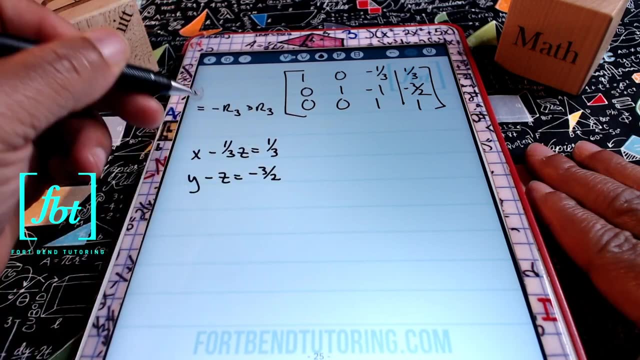 So now it's time to back substitute, and in back substituting you'll end up writing your system as: X minus one third, Z equals to one third. You'll also have for the next equation: Y minus Z equals to negative three halves, And for the third equation, Z equals to one. 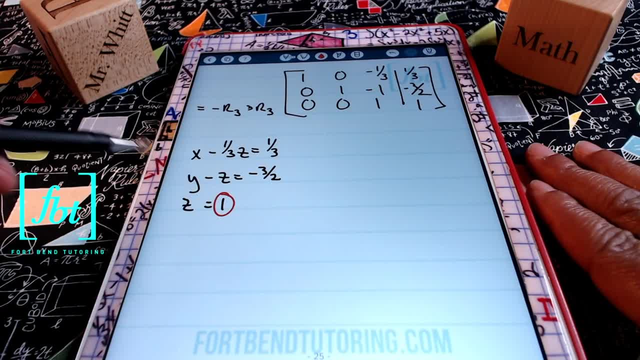 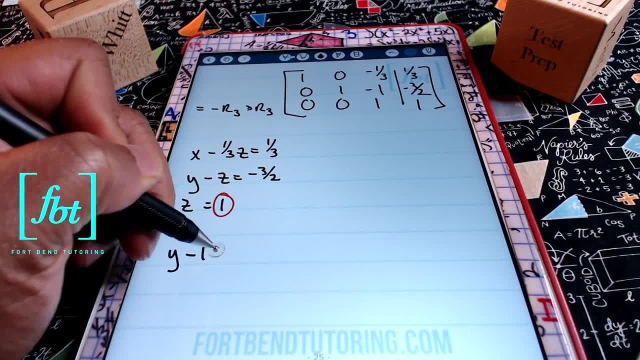 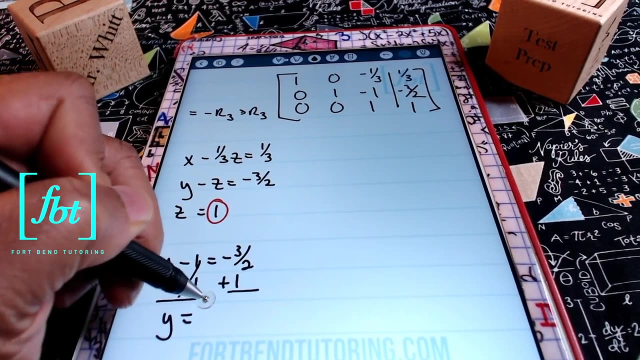 So we already have one of the three values solved for, which means we'll be plugging in one for Z in the previous equation. So I'll have Y minus one equals to negative three halves. Adding one to both sides of the equation, you'll have Y equals to two halves minus. 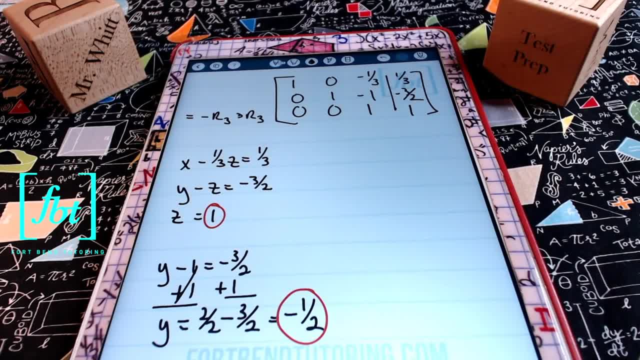 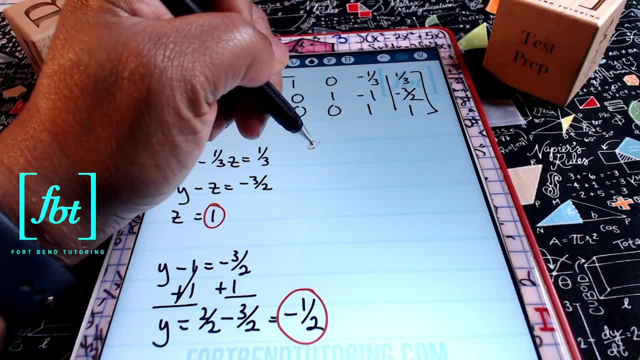 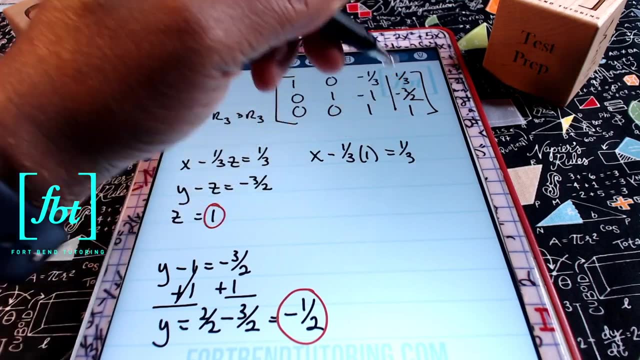 three halves, which gives you a result of negative one Half. So negative one half is our value for Y. Plugging both of these values into the first equation, we can solve for X. So we'll have X minus one third times Z, which is one equals to one third. 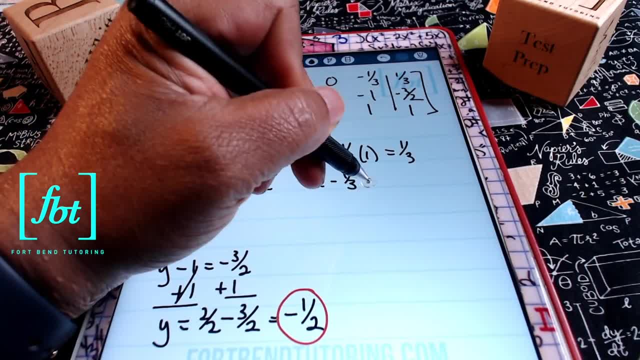 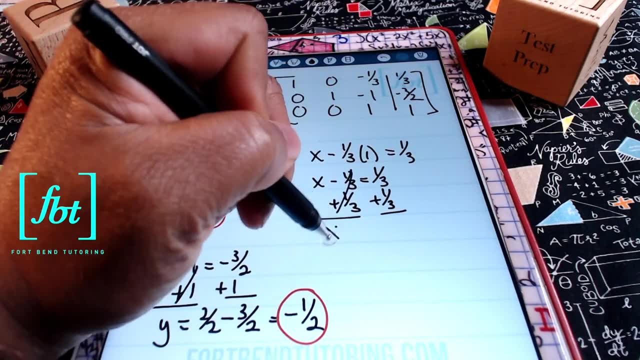 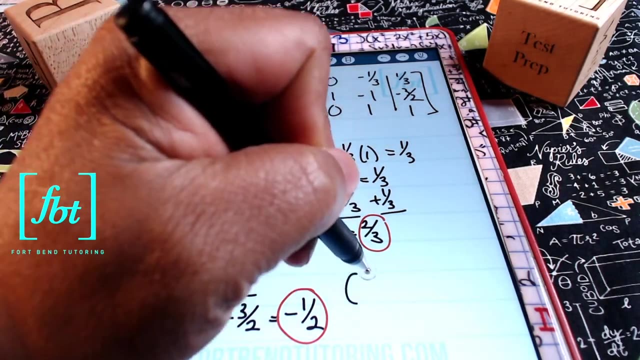 OK, simplifying, you'll have X minus one third equals to one third, And then adding one third to both sides of the equation, we'll find that X equals to two thirds. All right, So using these three values that we found, your order triple is going to be two thirds. 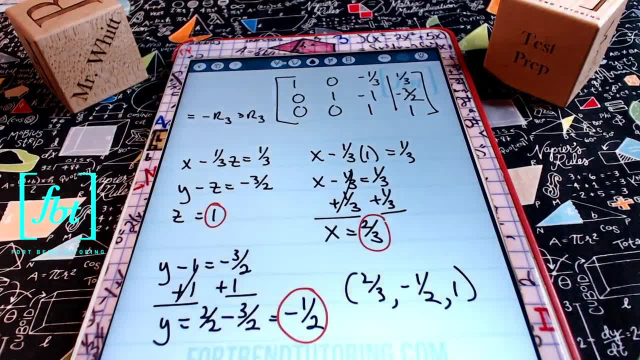 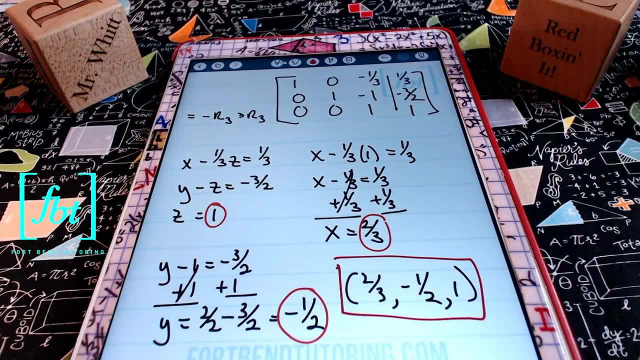 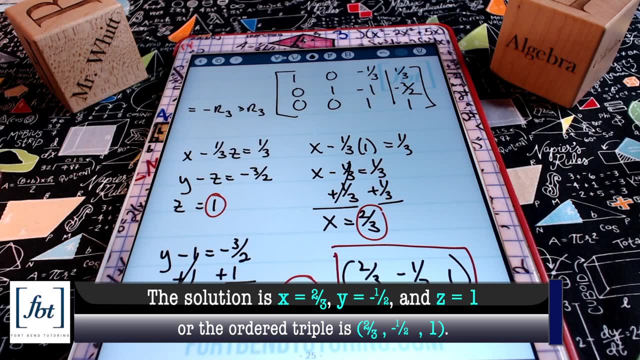 negative one, half and one, And this is the solution to problem number six. Red box: it just like that. people. There you go. That is the answer to problem number six. I want to thank each and every one of you that went ahead and stuck around to the end and go ahead and let me know if you. 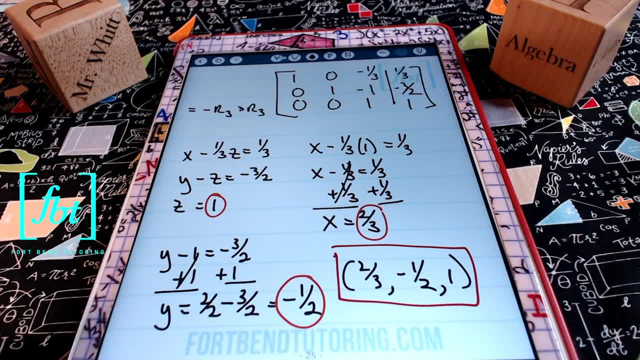 stuck around as long in the comments. OK, because the next thing I got to give you is a word problem that we'll use Row reduced form in order to solve. all right, aka the Gaussian elimination method. So here we have it, guys. 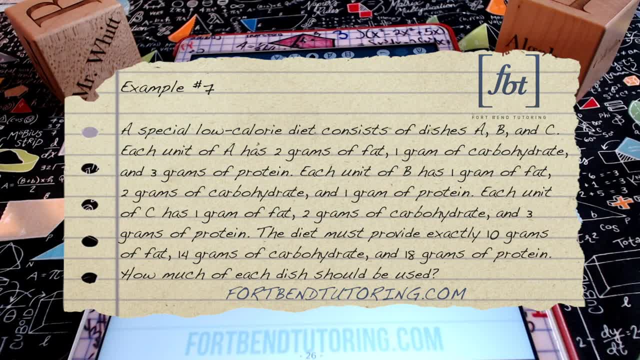 A special low calorie diet consists of dishes A, B and C. Each unit of A has two grams of fat, one gram of carbohydrate and three grams of protein. Each unit of B has one gram of fat, two grams of carbohydrate and one gram of protein. 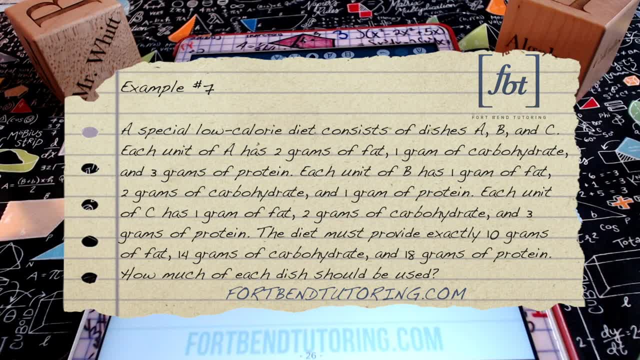 Each unit of C has one gram of fat, two grams of carbohydrate And three grams of protein. The diet must provide exactly 10 grams of fat, 14 grams of carbohydrate and 18 grams of protein. How much of each dish should be used? 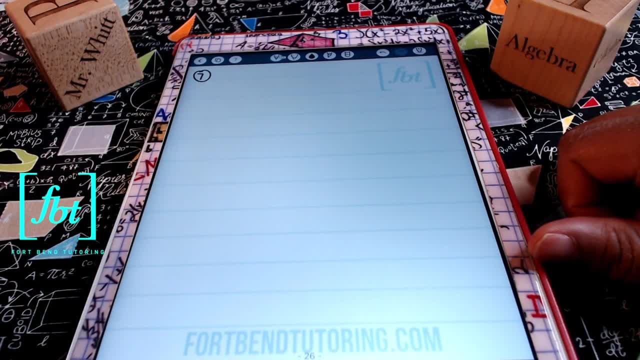 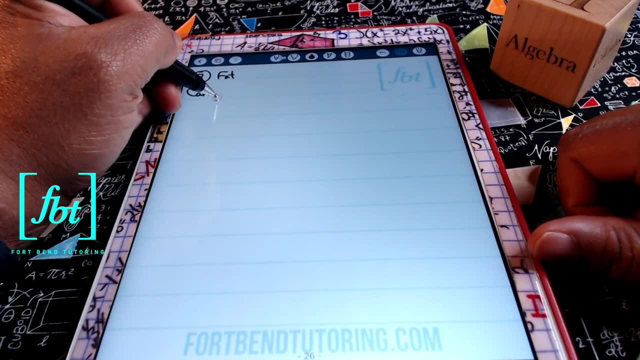 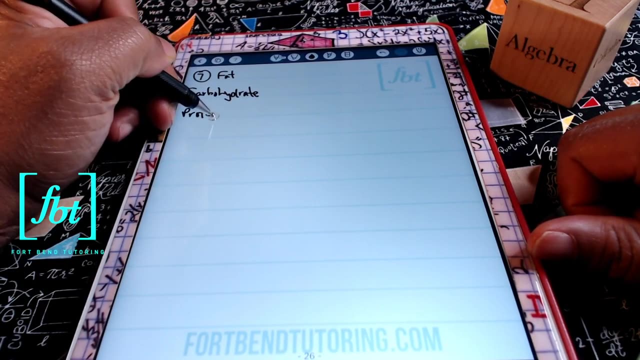 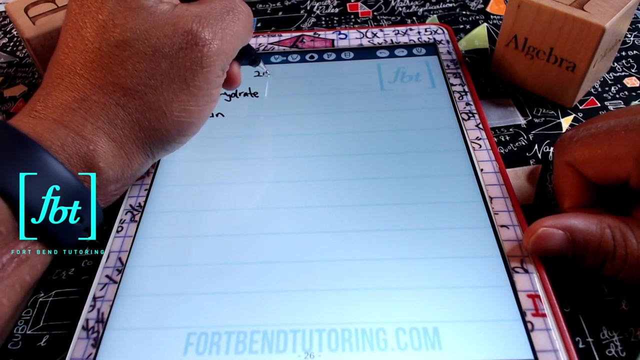 So for number seven and solving our word problem here, guys, we'll need to create an equation that represents the fat involved in the diet, as well as the carbohydrate, In addition to the protein. All right, So the equation that represents the fat in the low calorie diet is to a. 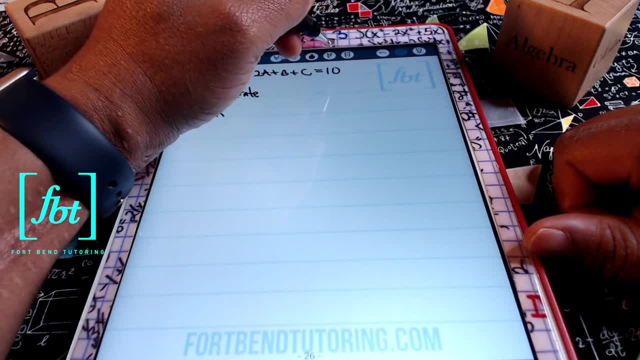 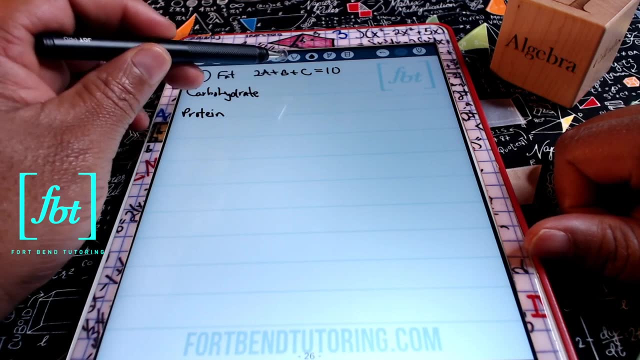 plus B plus C equals 10.. This lets us know that you will get two grams of fat and dish a, one gram of fat and dish B and one gram of fat and dish C, And the total grams of fat that the diet will allow is 10 grams of fat. 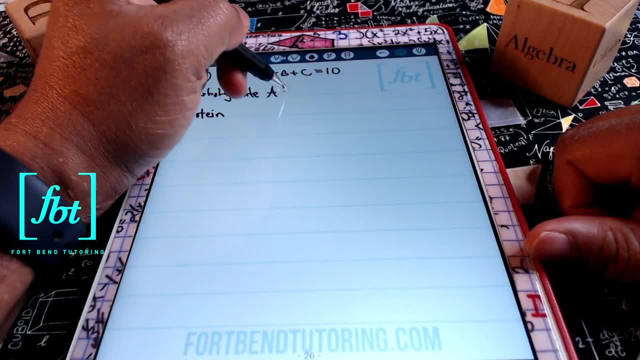 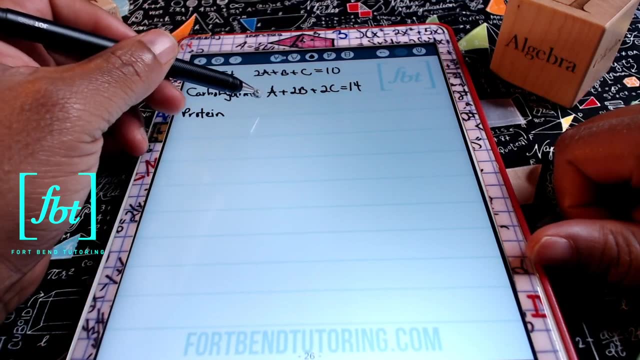 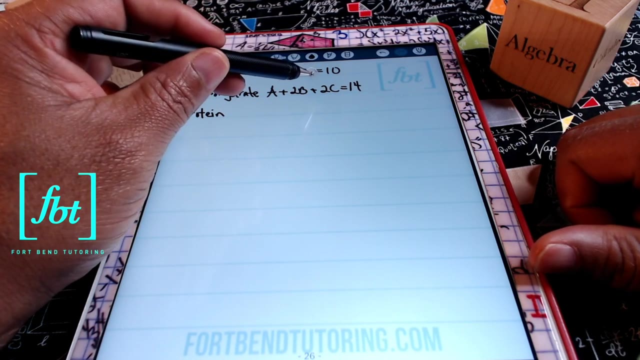 When it comes to the carbohydrate, you'll have a plus two B Plus two C equals to 14.. This is the representation of one gram of carbohydrate being in dish a, two grams of carbohydrate being in dish B, two grams of carbohydrate being a dish C. 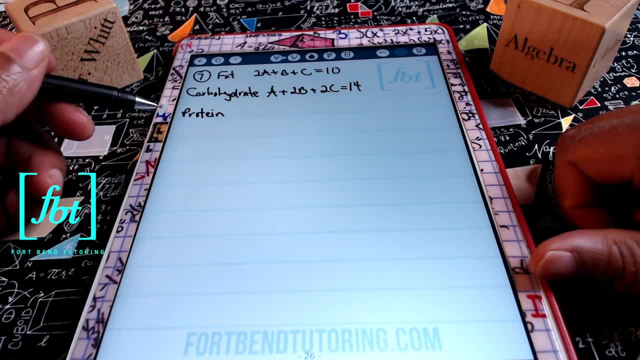 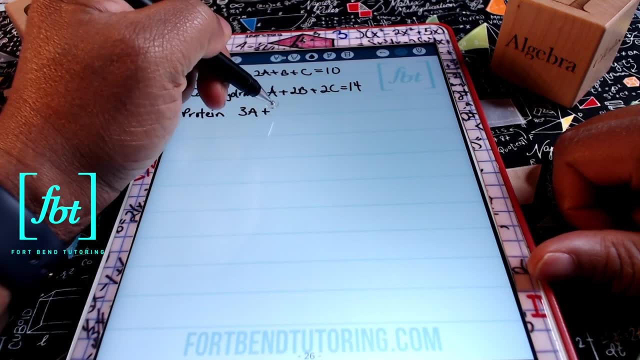 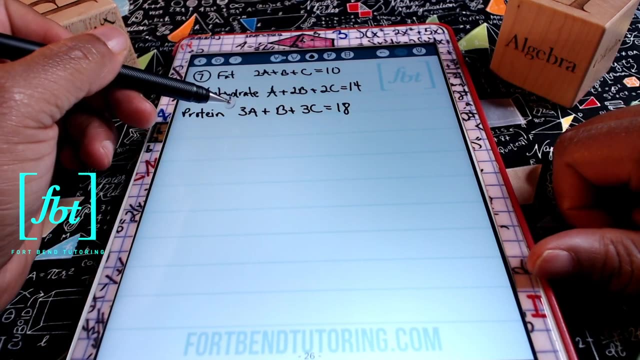 and that the diet allows for 14 grams of carbohydrate. When it comes to our protein in the low calorie diet, you'll have an equation that reads: three A plus B plus three C equals 18. And this simply means that you'll find three grams of protein in dish a one. 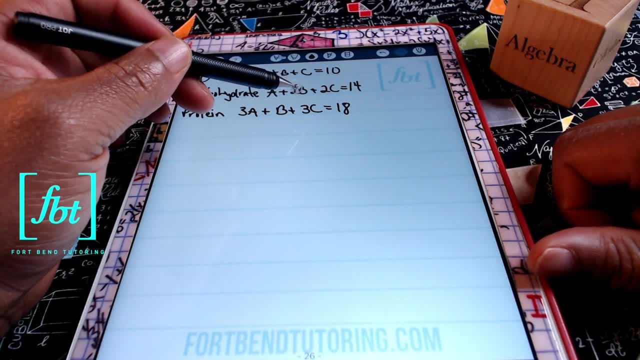 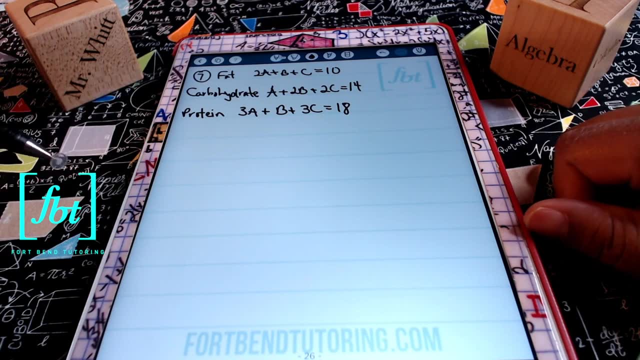 gram of protein and dish B, three grams of protein in dish C and a total count of 18 grams for the low calorie diet. Overall, these three equations make up your system with three variables, And now we'll be writing this system as an augmented matrix. 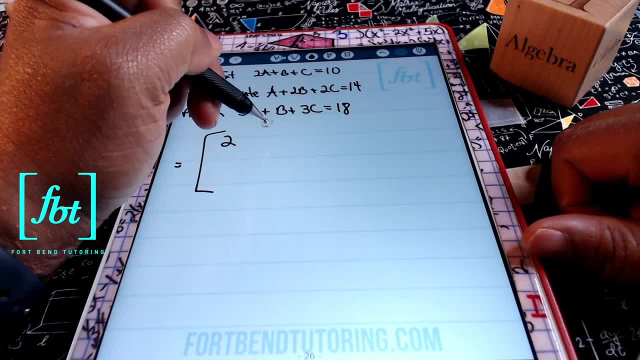 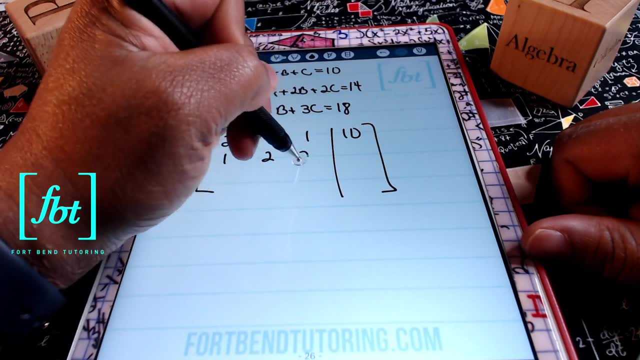 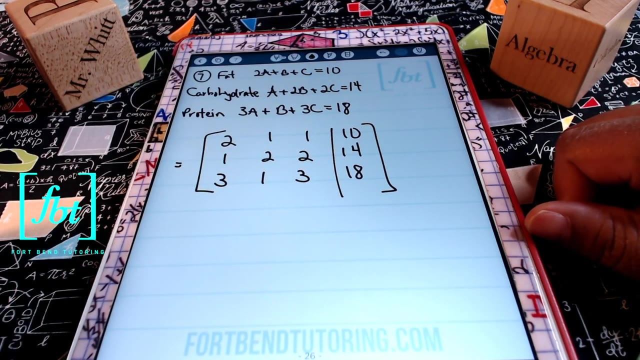 So what we'll have now is an augmented matrix with coefficients to one, one, ten, As well as One, two, two, fourteen and three. one, three, eighteen, And this is your augmented matrix, for example, seven. I really hope you guys appreciate the fact that we took the time out to present. 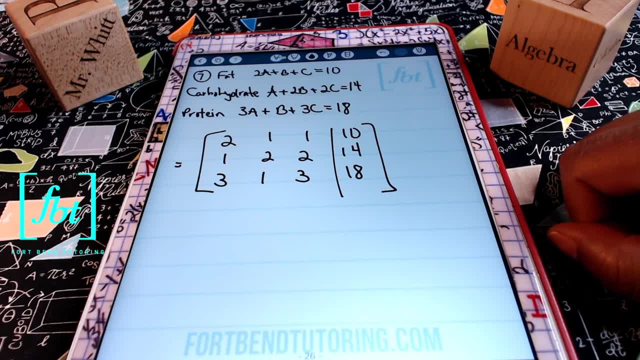 to you a word problem that can be solved using matrices and row echelon form. OK, go ahead and make sure you give us a thumbs up and share the video along the way. Yeah, So what I want to do next is I want to first of all swap out. 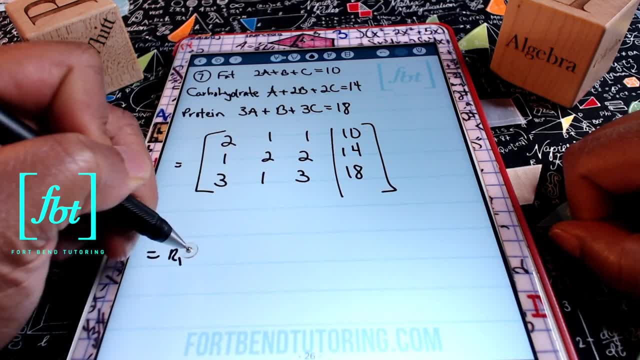 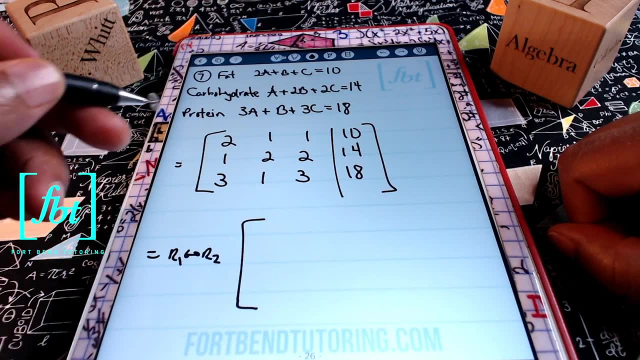 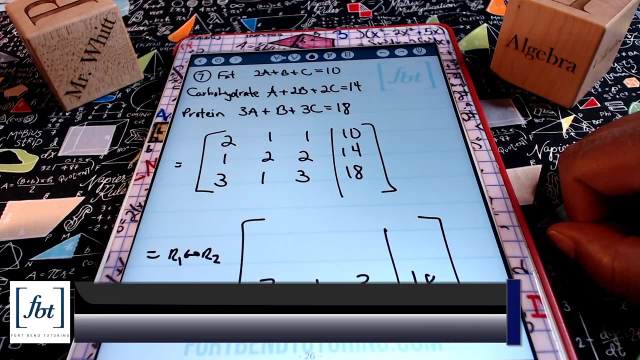 Row two and row one. so I'm swapping out row one and row two because I see that it has the coefficient that I want. so the only way that is unchanged is the last row: Three one, three, eighteen, And what we're going to do now is swap out row one with row two. 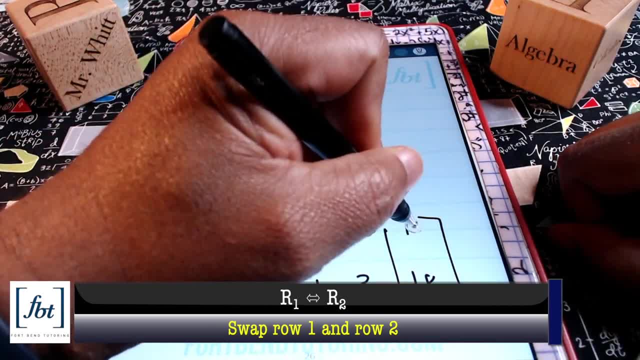 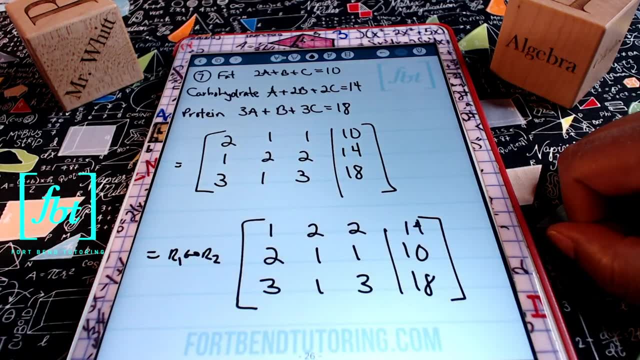 We'll have one, two, two, fourteen, And your new second row is going to be two one, one, ten, Just like that. For my next step, I'm going to want a zero where the two in the second row is. 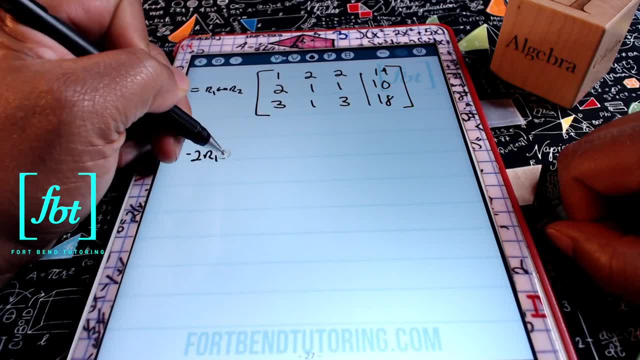 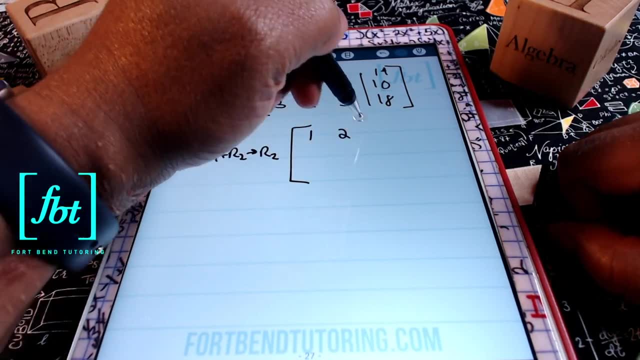 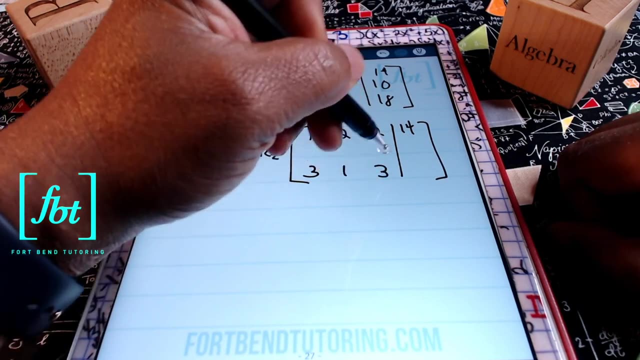 So I'll be multiplying negative two times row one and adding it to row two, putting the result in row two. That means that my first and third row doesn't change one bit. All right, They won't change. So the third column I have three, one, three and eighteen. 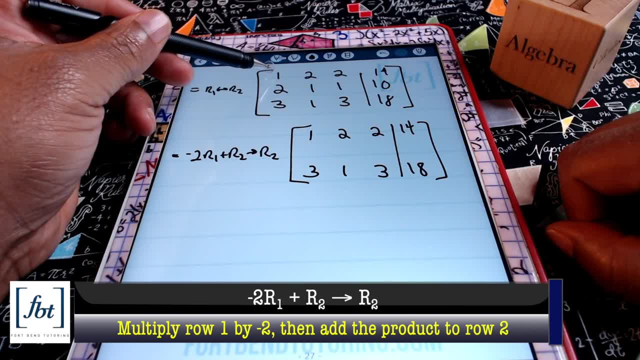 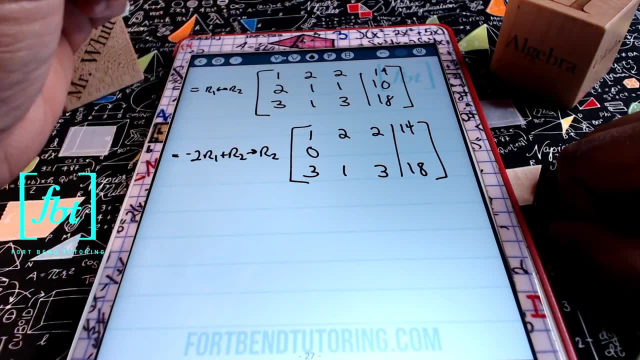 And I'll be multiplying negative two times one to give me negative two. negative two plus two is zero. Then I'll have negative two times two is negative four. Negative four plus one gives me negative three. I have negative two times two gives me negative four. 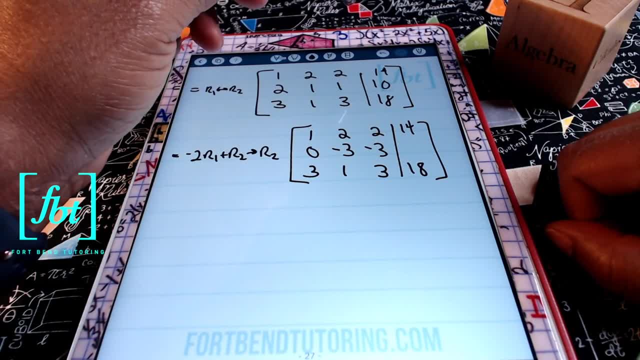 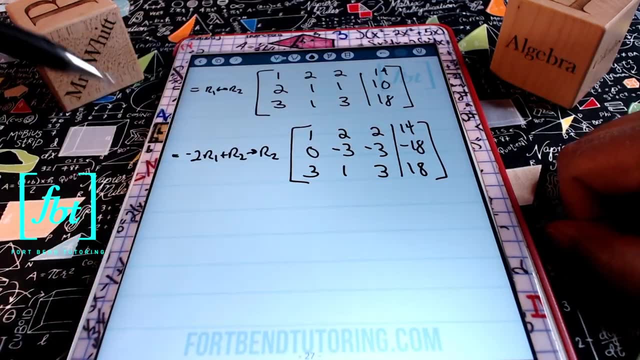 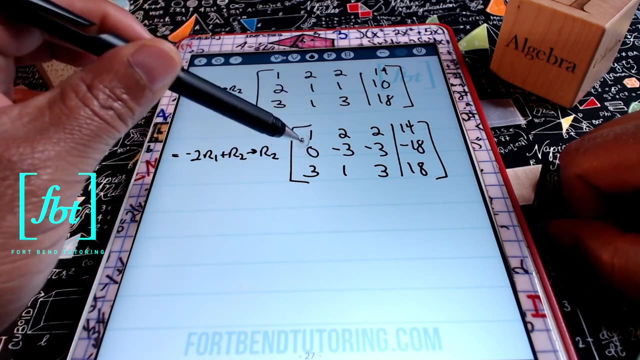 Negative four plus one gives me another negative three, And then negative two times fourteen is negative twenty eight. Negative twenty eight plus ten is negative eighteen. And this is going to be our new second row after we complete that operation, All right. Next I'll be wanting a zero where the three is in the third row. 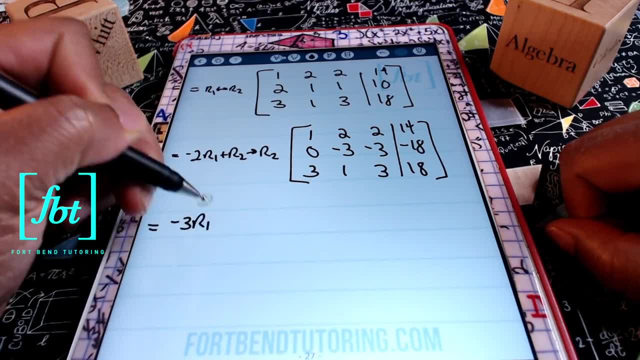 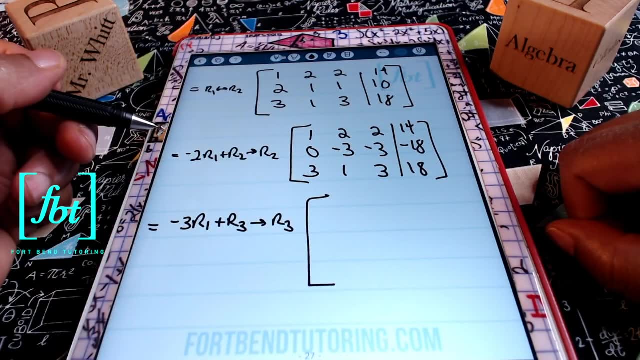 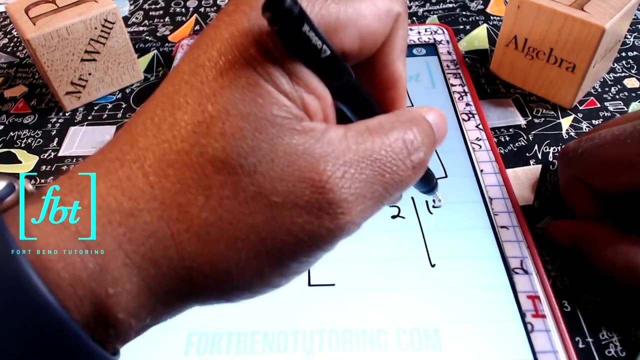 I can get that by multiplying negative three times row one plus row three, Putting the result in row three. What does this give me? This gives me an opportunity to bring down my first two rows unchanged. We'll have one, two, two, fourteen as well as zero. 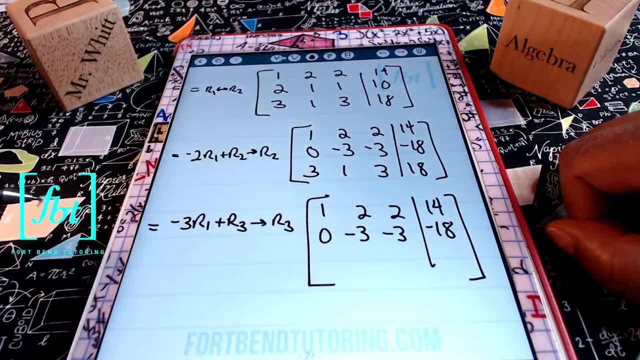 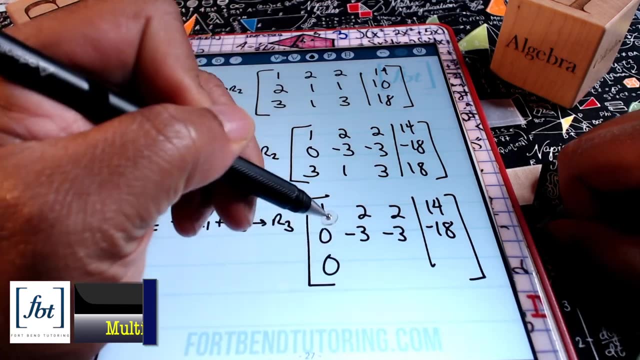 Negative three: negative three, negative eighteen. And then we also have row three where we'll be multiplying negative three times row one, Adding that product to row three, So we'll have negative three times. one is negative three Negative three plus three gives me zero. 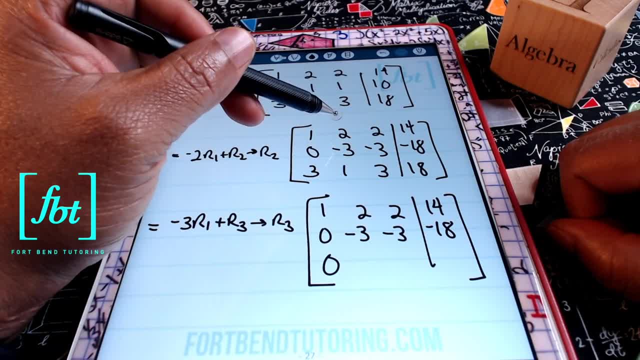 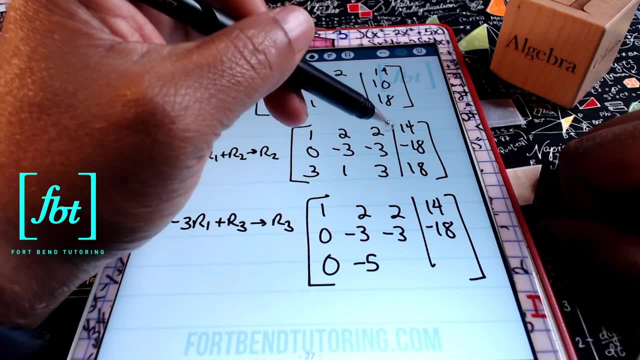 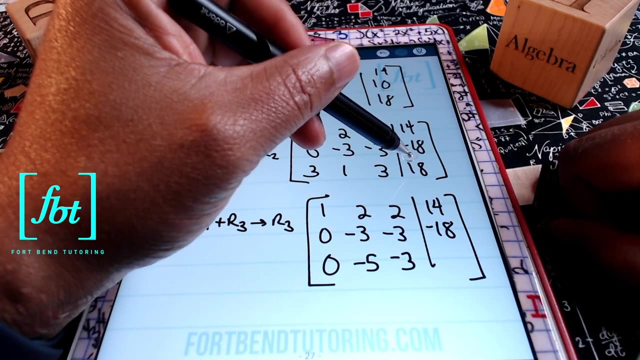 Negative three times two is negative six. Negative six plus one gives me negative five. Negative three times two is negative six. Negative six plus three gives me negative three. And then negative three times fourteen is negative forty two and negative forty two plus eighteen is negative twenty four. 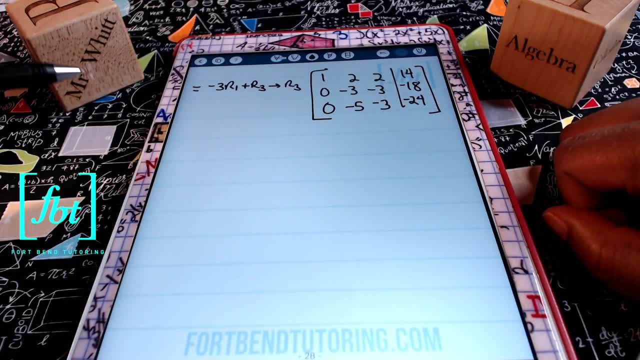 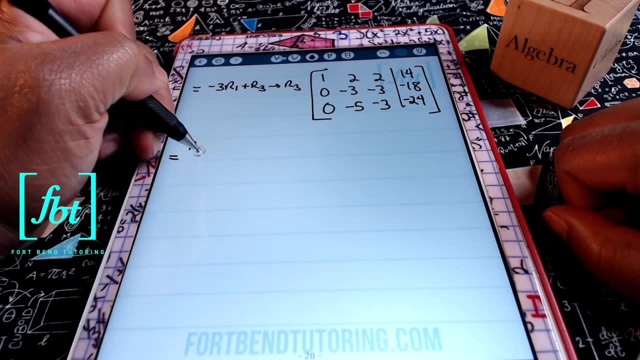 And now I want to get a one in the element in the second row, second column, aka, where this negative three is in the middle. I can do that by dividing row two by negative three, putting the result in row two. 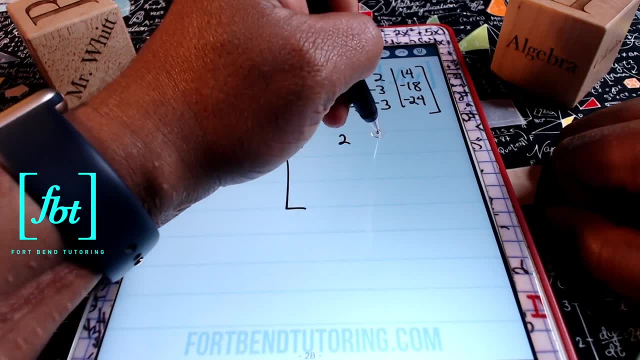 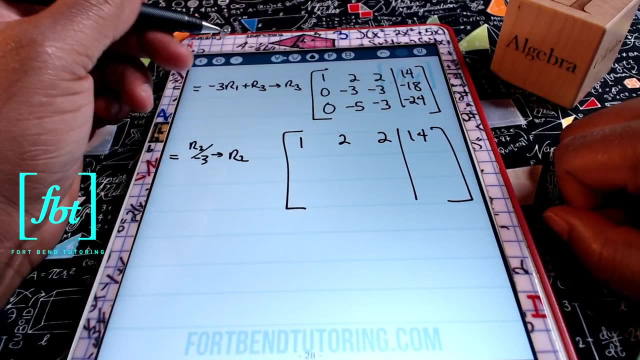 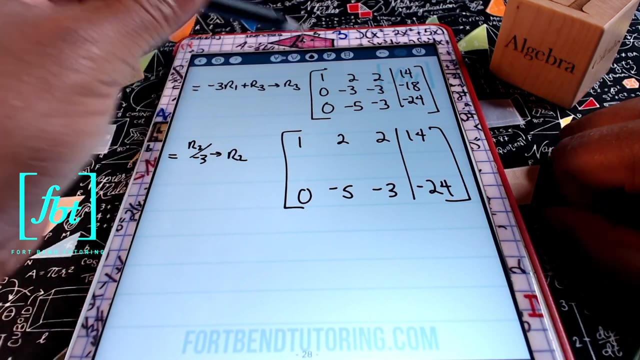 That means that the first row and the third row will go unchanged. So we'll bring down the one, two, two, fourteen. The third row is zero, negative five, negative three and negative twenty four. And then for the second row, just divide each and every element by negative three. 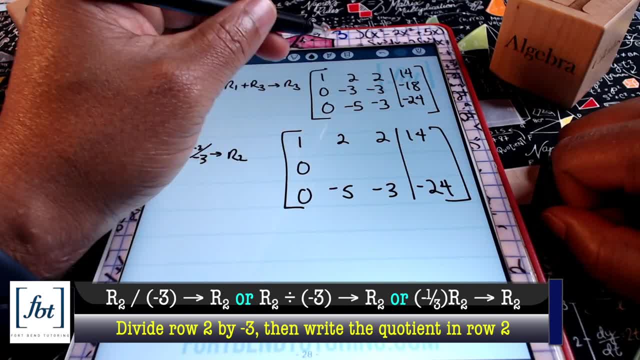 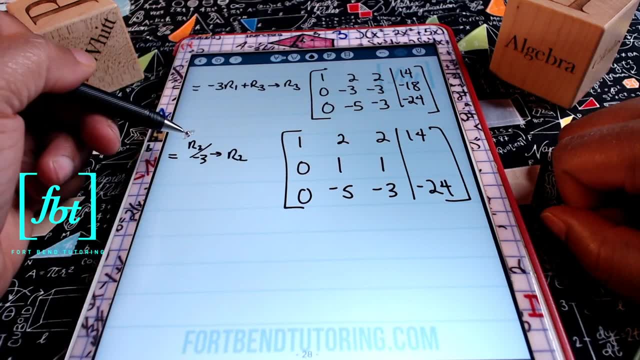 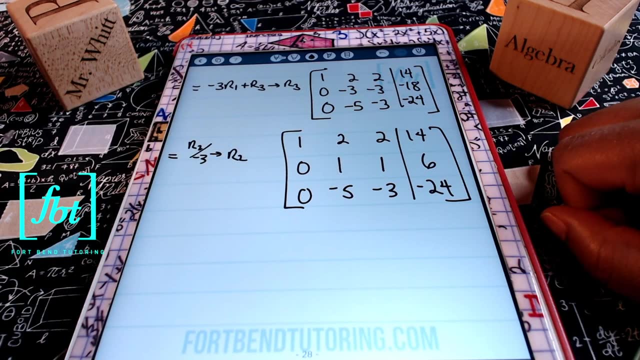 Zero divided by negative three gives you zero. Negative three divided by negative three is one. Then negative three divided by negative three also gives you one, And negative eighteen divided by negative three is six. So our next goal here is to get a zero in the third row, second column. 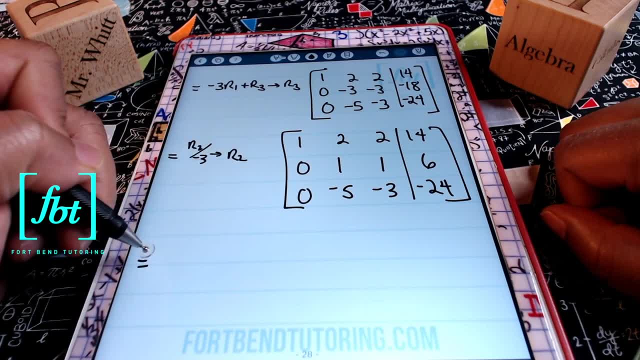 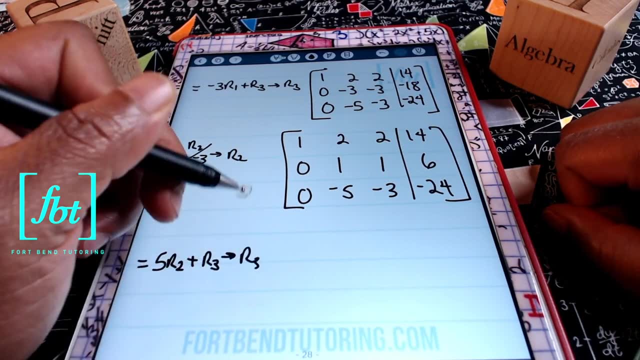 The way I propose we do that is to multiply row two by five. So I'm going to say five times row two, Add that to row three, put the result in row three and that's our next operation. Guys, this means that the first two rows will go unchanged. 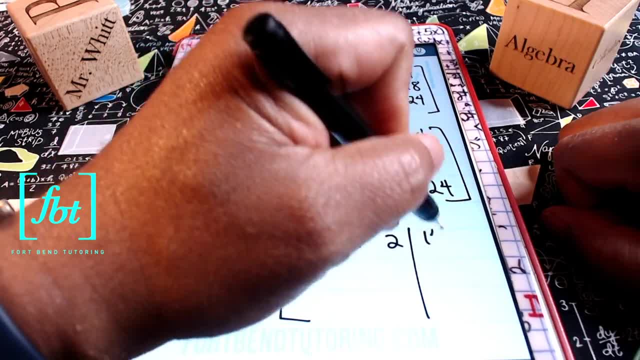 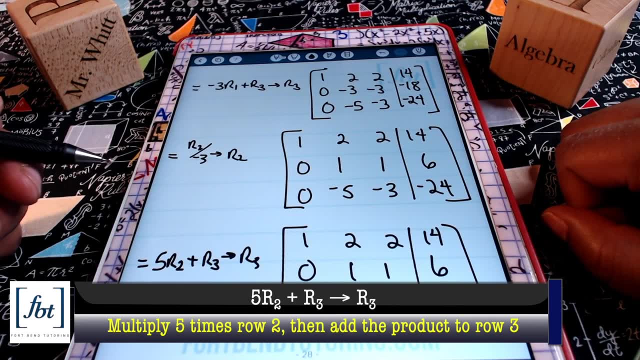 Bring down the one, two, two, fourteen, Then bring down your zero: one, one, six, And then finally, to get the third row, we're going to multiply five times zero to give you zero, and then zero plus zero is. 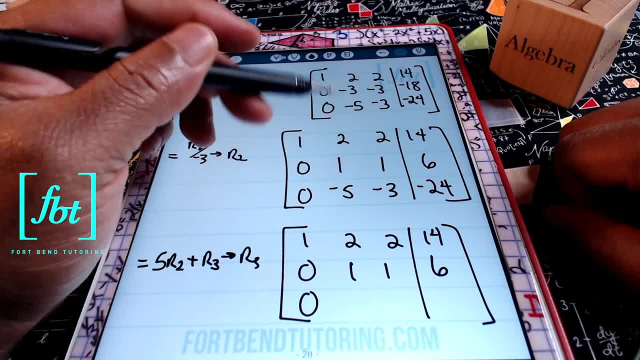 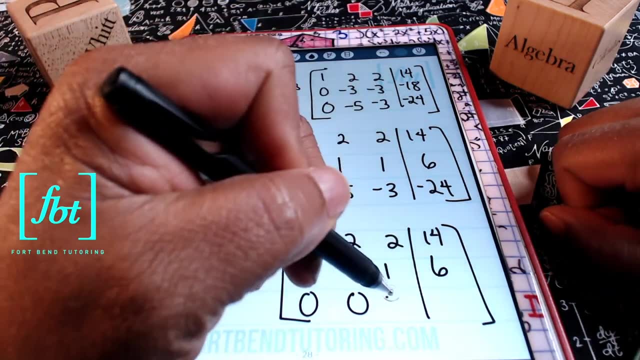 zero, Then five times one is five. Five and negative five combined to give you zero. We then have five times one is five, five and negative three combined, to give you positive two. and then five times six is thirty and thirty and negative twenty four. 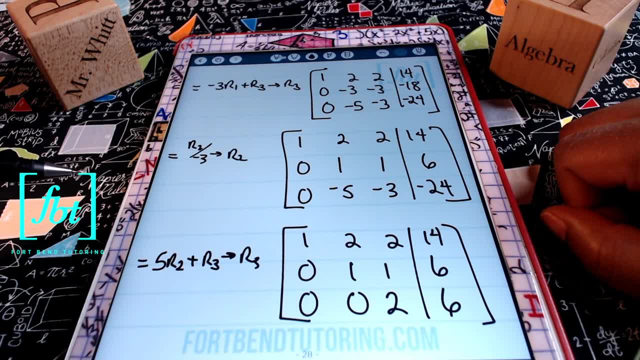 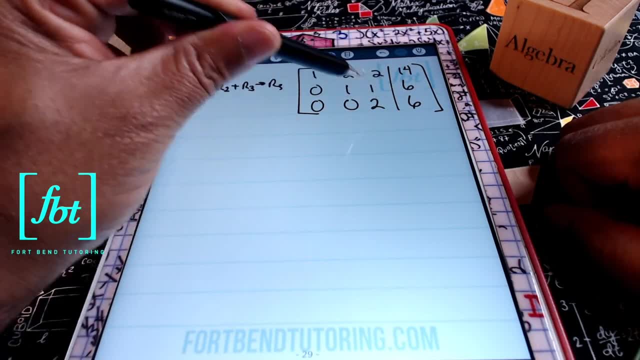 give you six. So this is our current result Before we do our last step here, guys, And what is that last step? You got it Putting a one right here where that two is in the third row. We can easily do that by dividing row. 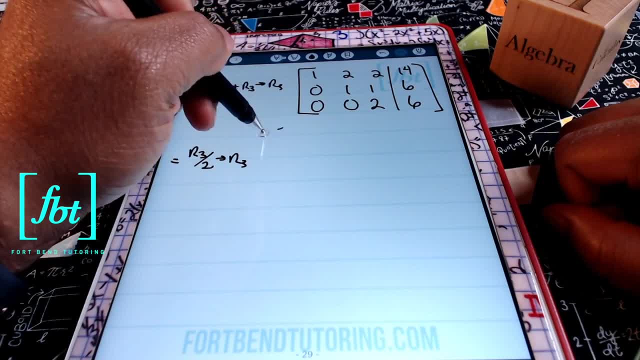 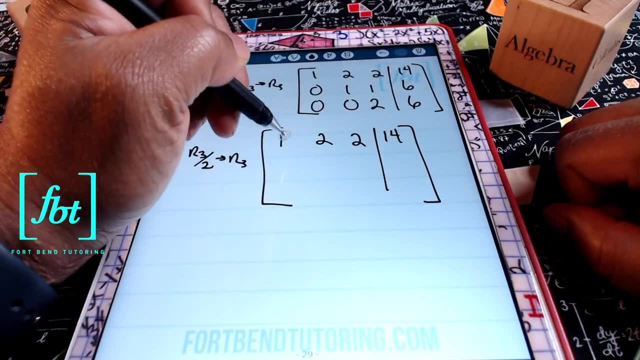 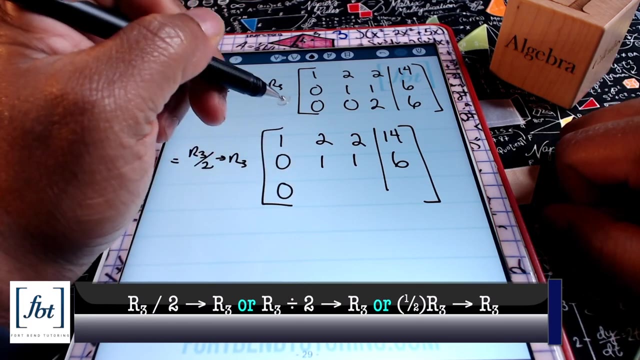 three by two. putting the result in row three, That means that our first two rows will go unchanged. So just bring that information down, guys. Zero, one, one, six And now divide every element in row three by two. So zero divided by two is zero. 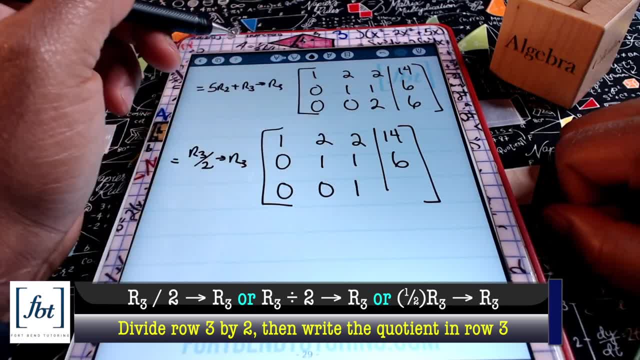 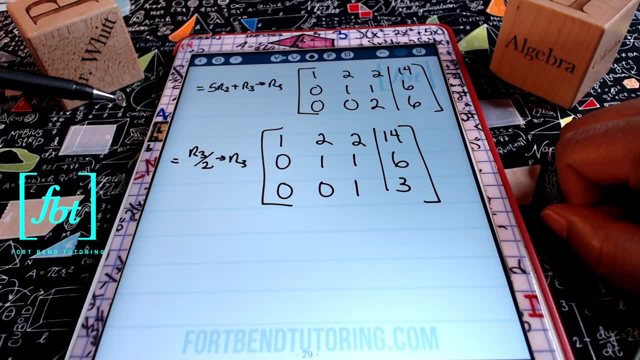 Zero divided by two is zero, Two divided by two is one, and six divided by two is three. You now have your augmented matrix in row echelon form. You know this to be the case because the elements in your main diagonal are all ones and you have zeros underneath those. 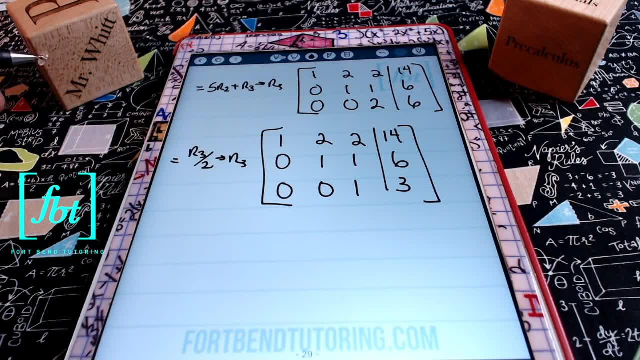 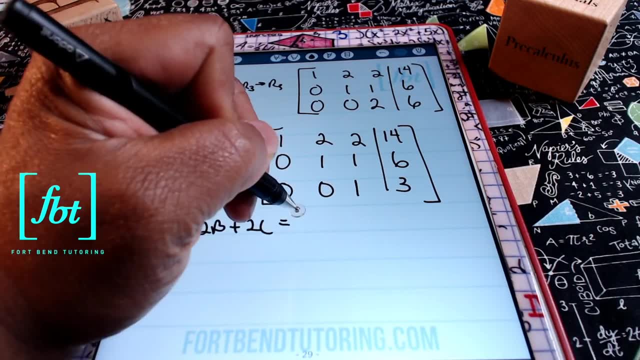 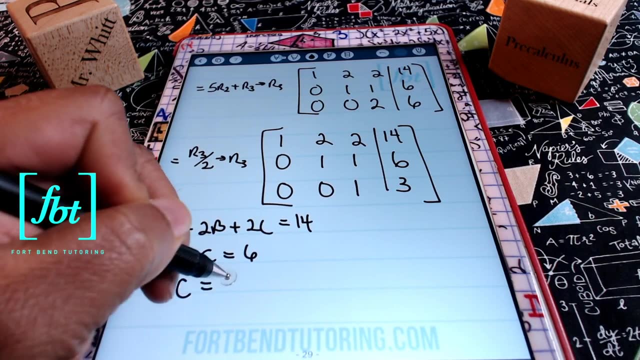 ones. OK, so that being the case, then we will now back substitute. So in back substituting, you'll have A plus two, B plus two, C equals fourteen. You'll have B plus C equals six, and you'll also have C equals to three. 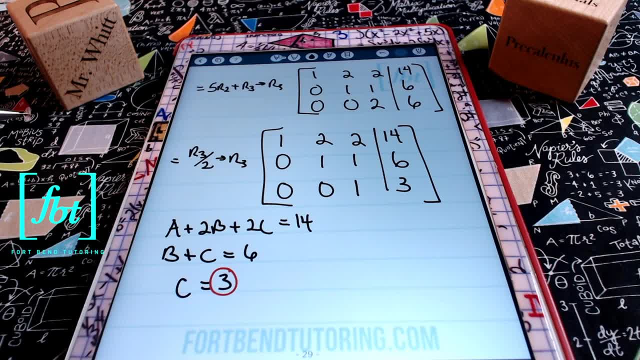 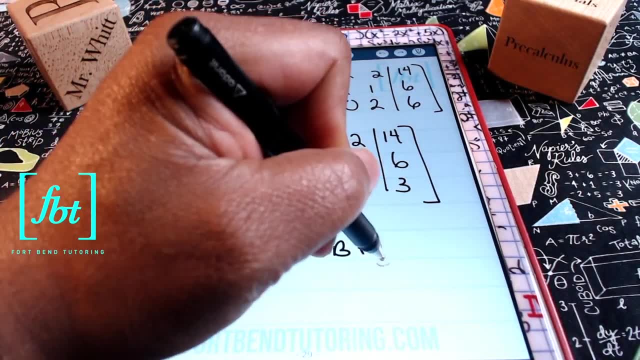 In this case we already know the value of C and we know that value is three. So using this value, we'll be plugging that into the second equation. So I'll have B plus three equals six, replacing the C with the three there. 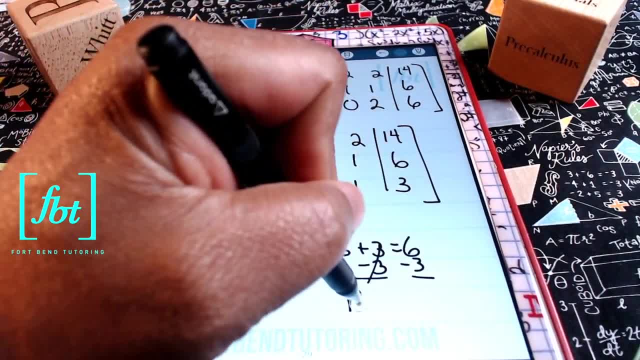 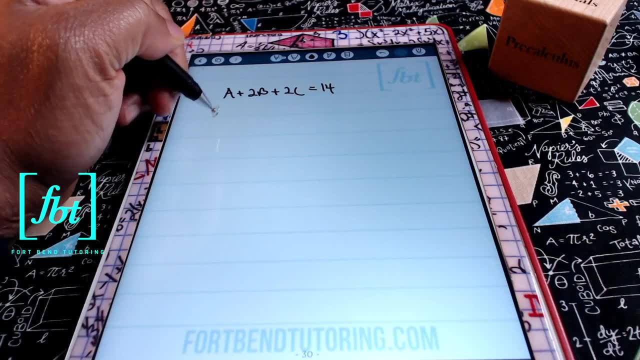 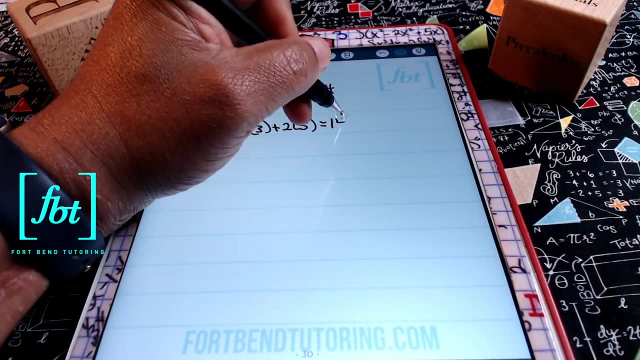 Then, solving for B, we find that the value of B is three. Using these two values, we'll be plugging that into our first equation, So we'll rewrite the equation as: A plus two times three plus two times three equals fourteen. This then gives me A plus six plus six equals. 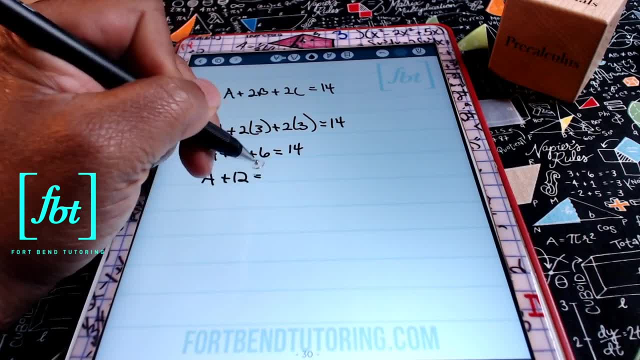 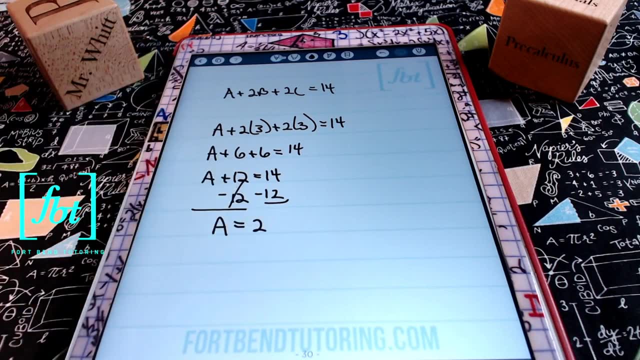 fourteen. In simplifying, you'll have A plus twelve equals to fourteen. Subtracting twelve to both sides of the equation, you'll find that A equals to two. This value of A is going to be the last value that you needed in order to write your result. 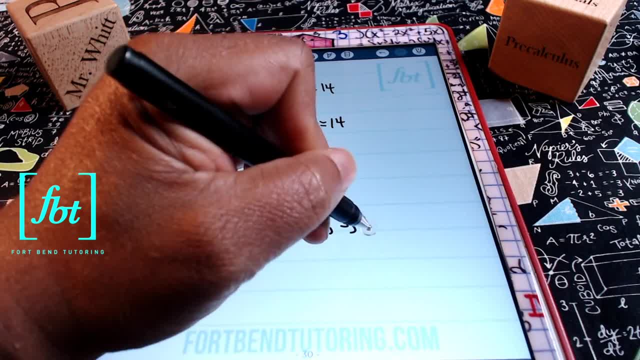 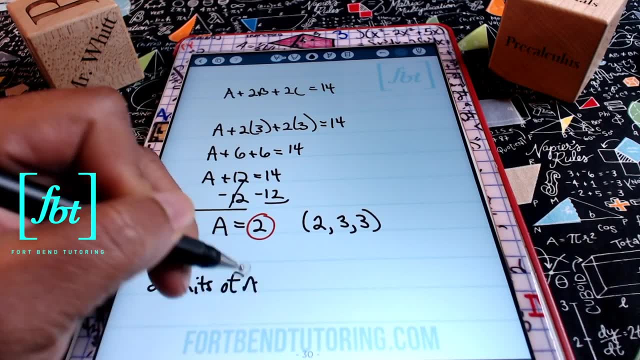 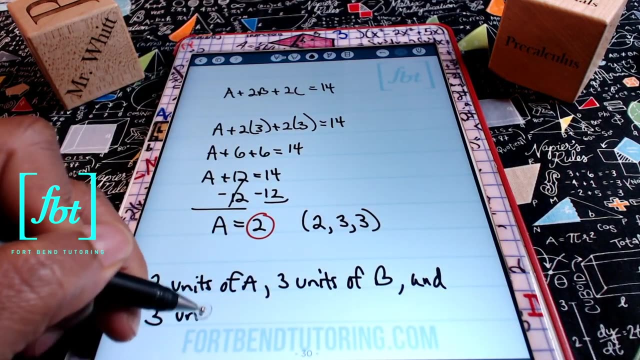 And what is your order? triple, You'll have two, three, three. And what does this mean in the context of our word problem? You'll need two units of dish A, You'll also need three units of dish B And you'll also need three units of dish C. 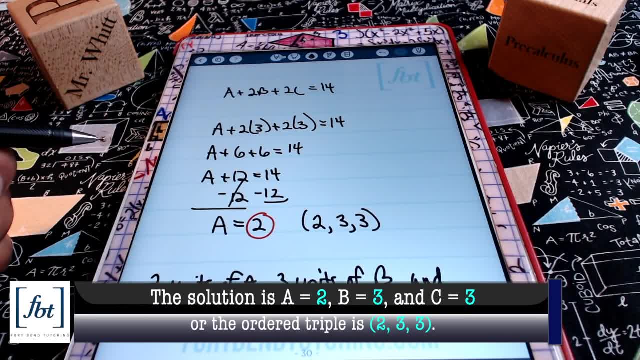 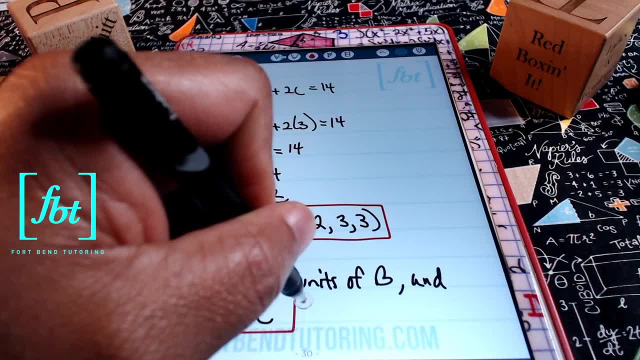 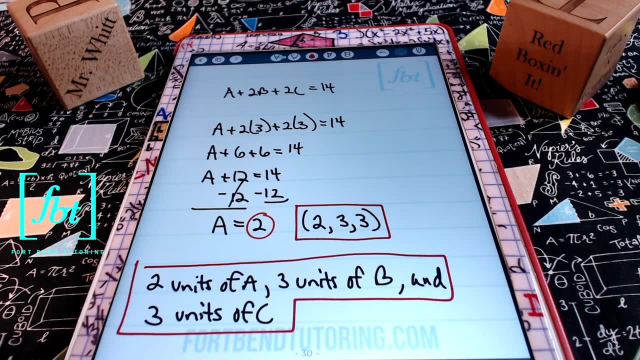 And this is going to be the answer for problem number seven, Red box it. So here we have our simplified form And if you're going to spell it out for your word, problem guys, this is the expanded version here. So this tells us how many of each dish we'll need to solve that problem. 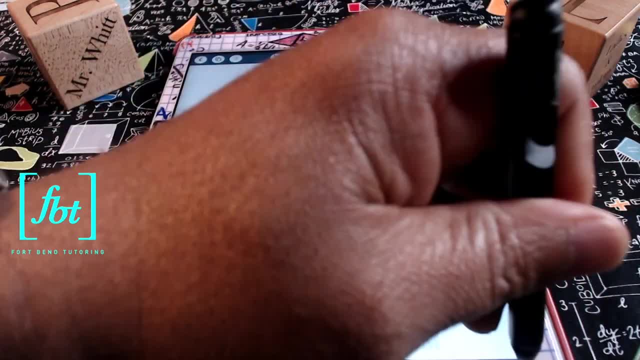 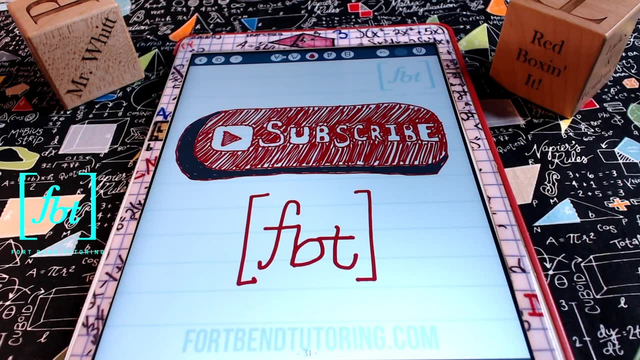 Done and done people. All right, then, guys, that means that I need you to please like, comment, share the video with everyone you know and love, because this concludes this video on the Gaussian elimination method, aka solving matrices and row echelon form, presented to you by Mr